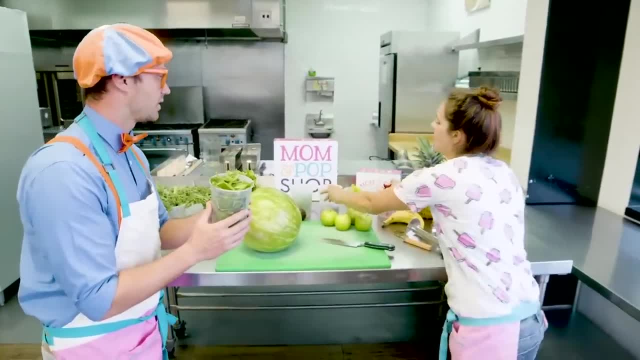 Okay, So here you go, hold the spinach. I was making a batch earlier, so I thought we could just add to it. Okay, so here's some spinach And what do you have? Strawberries, Strawberries, And to sweeten it we use dates. 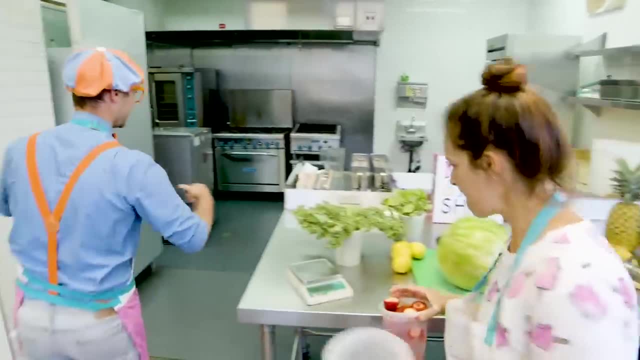 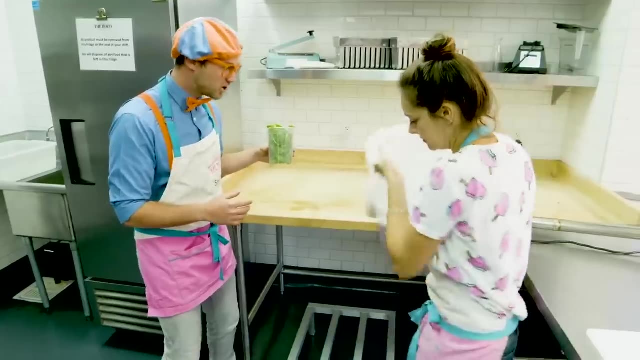 Ooh dates, All right, Come on back. Oh, okay, So here's the batch I was working on earlier. Oh, look at it. All right, That looks yummy. Go ahead, let's add it in. Okay, bye-bye, spinach. 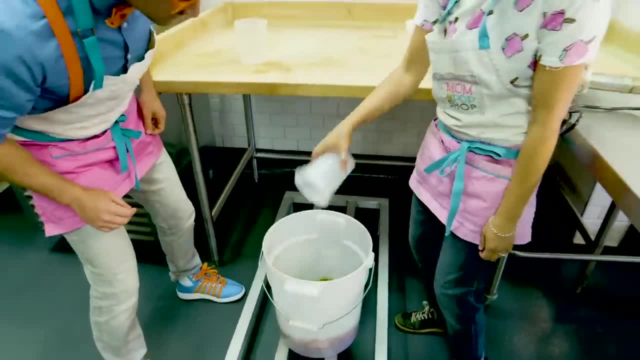 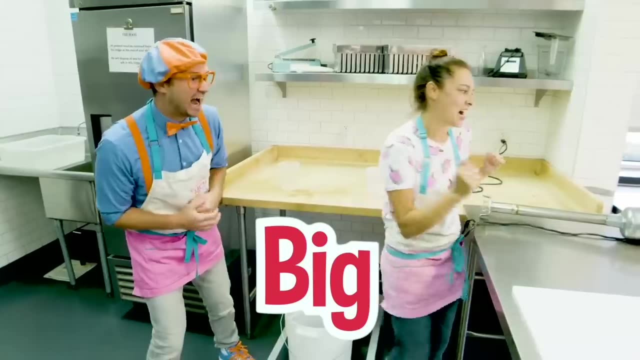 And then here are some strawberries- Ooh, And dates, Yum. Now, what might be different about your kitchen is we have some big equipment we use here. Really, I'm excited. Are you ready? Whoa, look at that. 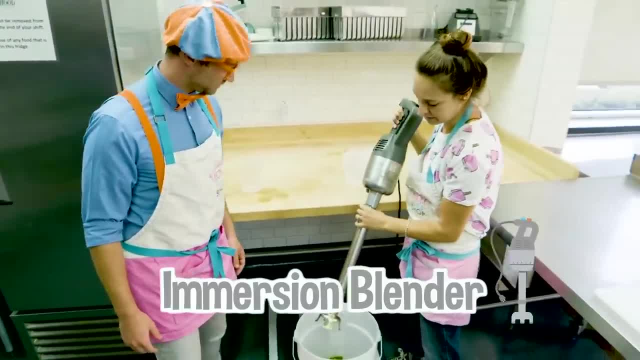 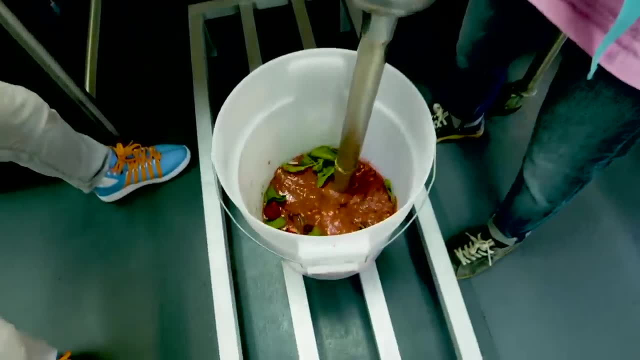 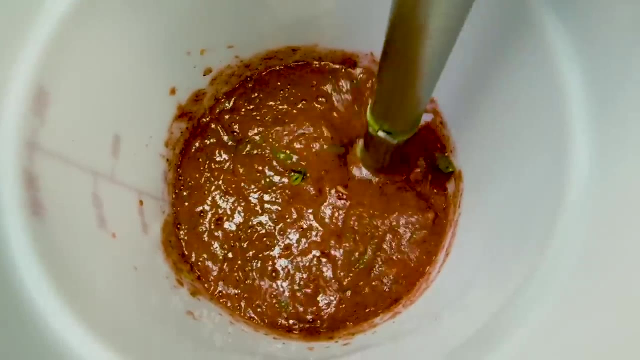 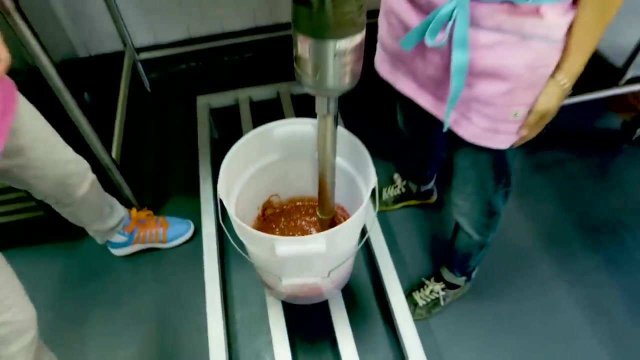 That thing is massive. What does that thing do? This is our immersion blender. Wow, So you put it in Whoa, You hit the button: Whoa, Whoa, There you go. So that just blends it up into a liquid. 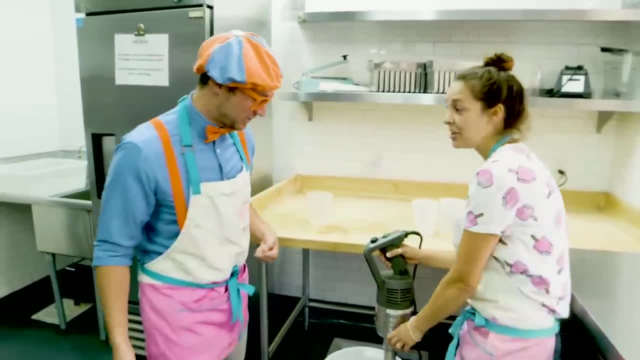 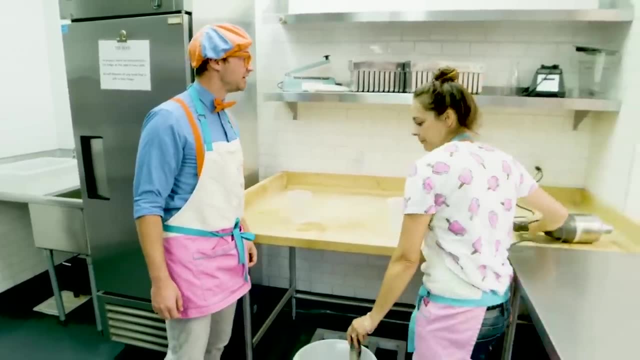 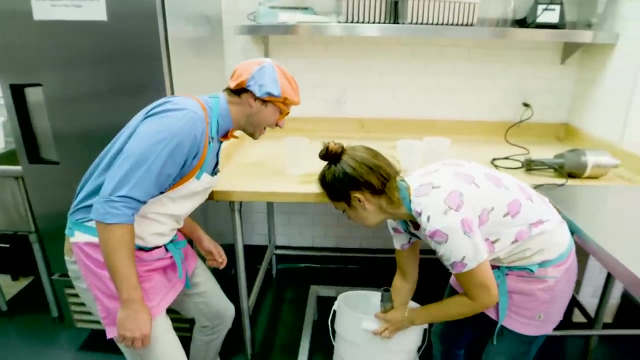 Yes, it sure does. Wow, that looks so yummy. Well, now, what do we do? Now, we're gonna put it in our mold, Okay, And I'm gonna get my trusty pitcher. Ooh, All right. So it's basically three ingredients. 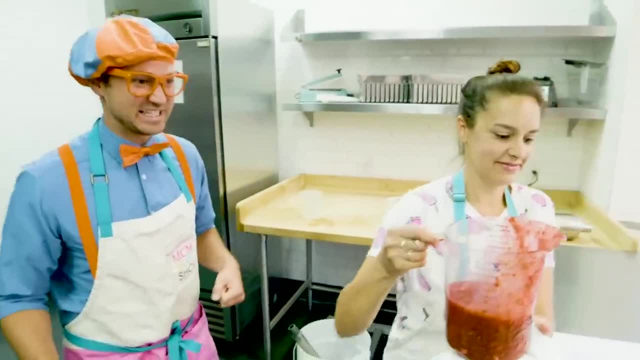 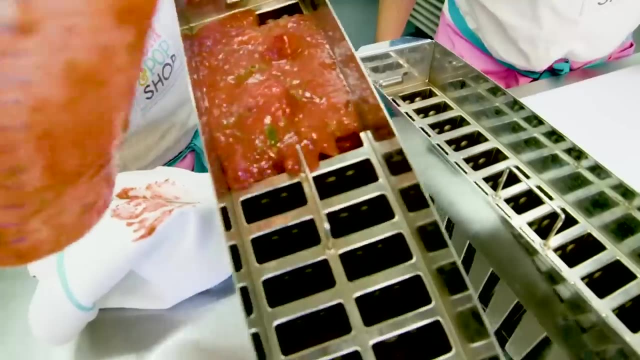 All blended up to make one yummy-tasting liquid. So now what we're gonna do is we're gonna pour it in, Oh, And then you kind of just have to feed it through, Shake it around. Yeah, May I, Of course. 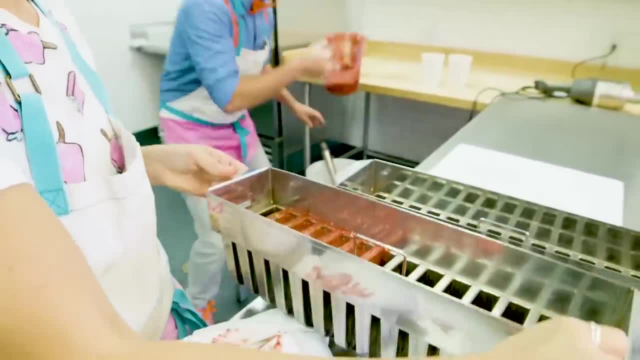 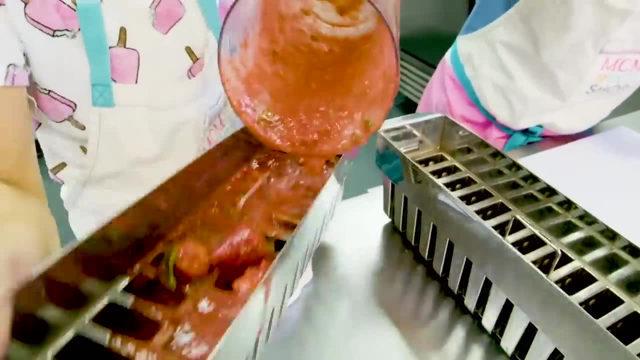 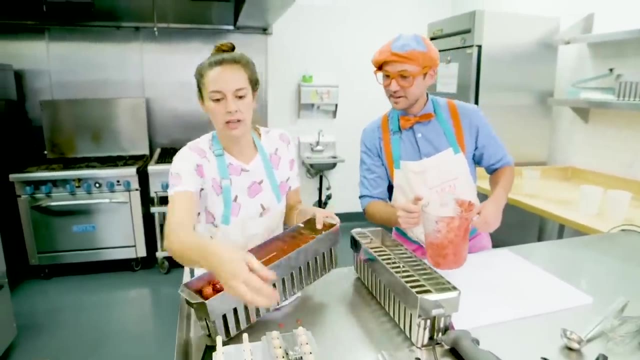 Okay, Here's some more. Whoa, We got some chunky ones in there. That's okay. There's some more? Okay, And then next, what we need to do is we'll just put in our sticks, Ooh. 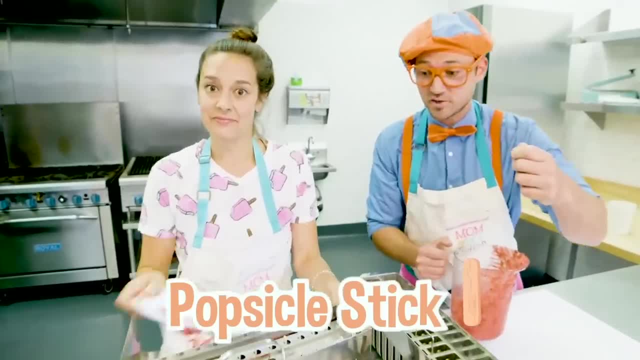 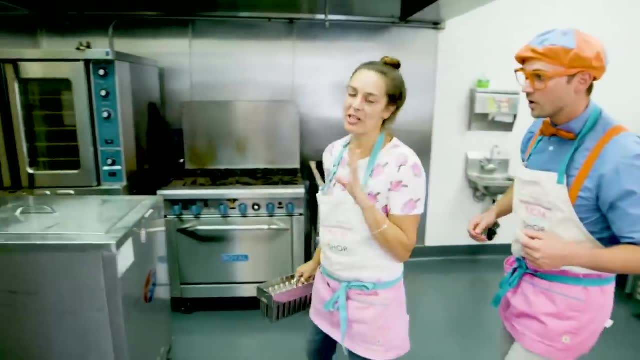 Yeah, like a Popsicle stick. Have you ever eaten a Popsicle? and you hold onto the piece of wood? Yeah, that's what we just put in there. That's what makes them so handy. Okay, And now we put it into our extra special Popsicle machine. 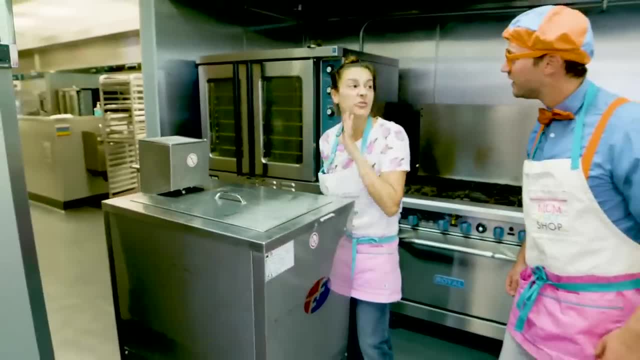 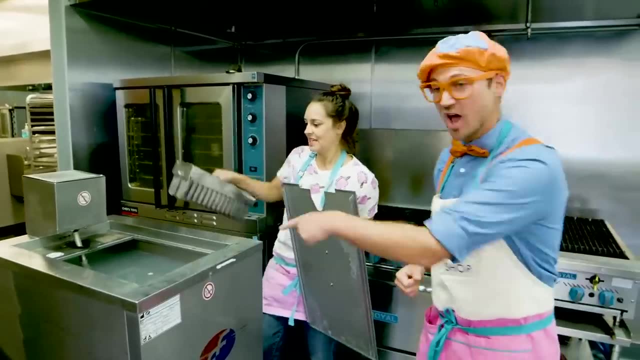 Whoa. What does this thing do? It makes it super cold. It freezes a Popsicle in 18 minutes. Wow, I'm so excited. I sure do love Popsicles. Hey, check it out, Let's put it in. 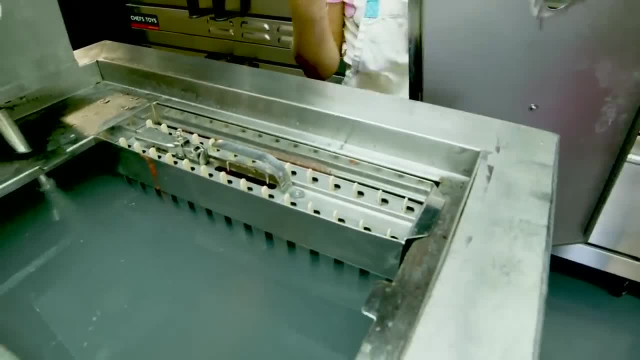 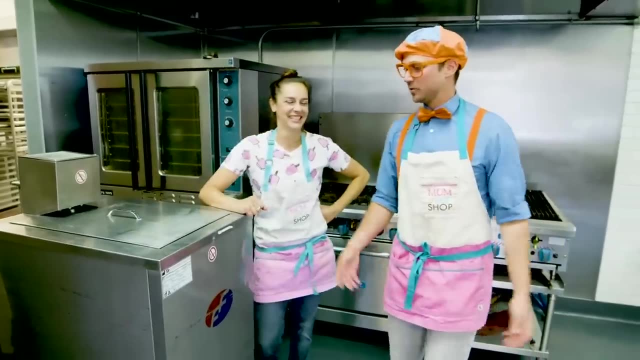 Whoa. So is that just really cold in there? Yes, it's actually made out of a special Popsicle freezing liquid Whoa. All right, I can't tell you all my secrets. Huh, Maybe for later. Well now, what do we do? 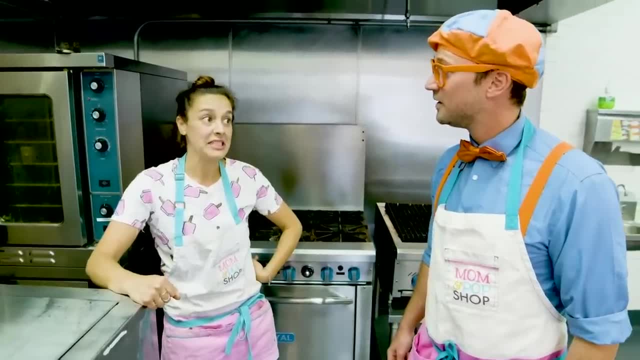 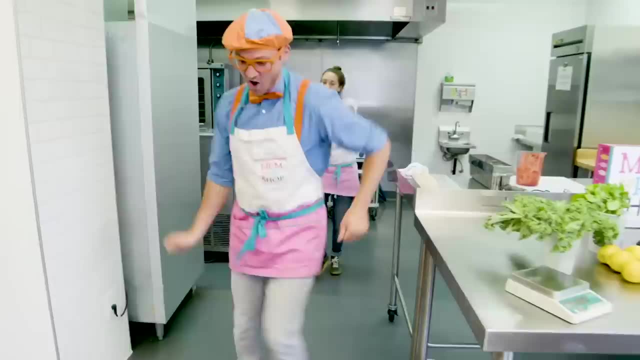 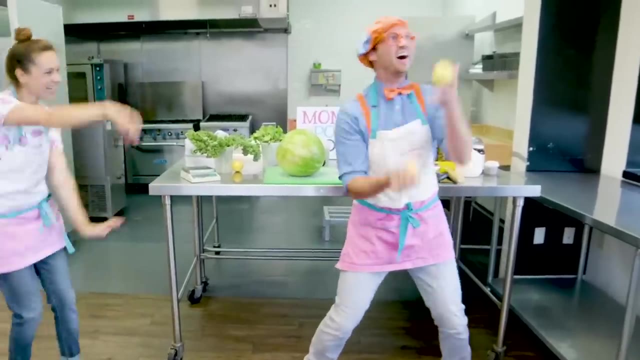 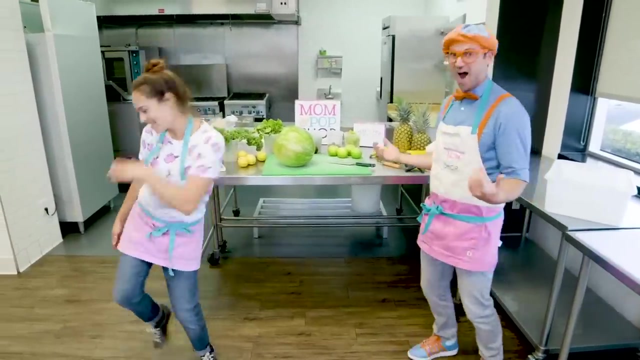 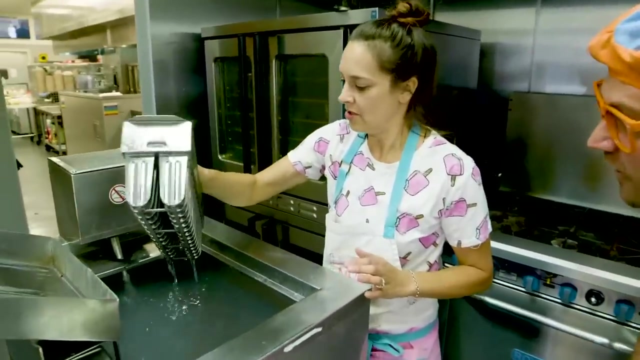 Well, usually when I wait for Popsicles to freeze, I like to dance. Okay, let's go. Woo-hoo, Whoa. Does that mean it's done? Sure does. Oh, All right, let's shake off that good Popsicle liquid. 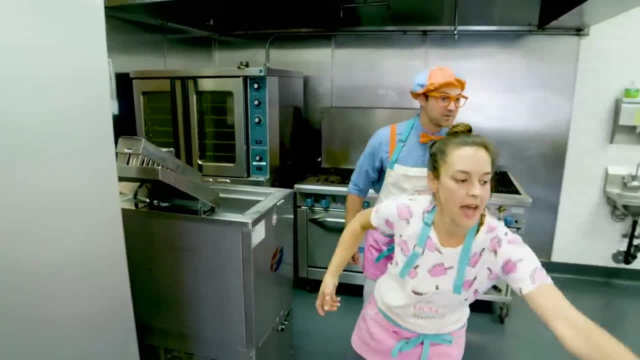 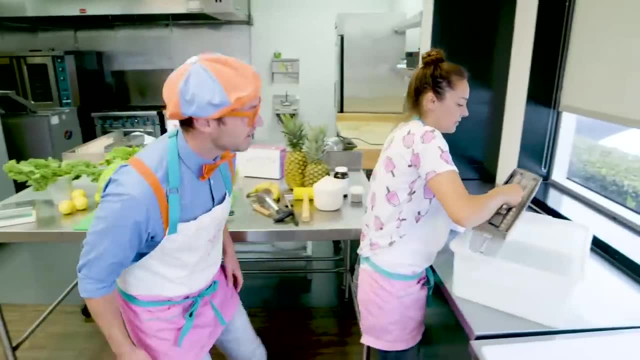 Okay, Let it dry. All right, I'm going to grab this towel, so we don't slip on it. That'll make a fun dance move. Yeah, We have to put it in the liquid. Okay, and what does that do? 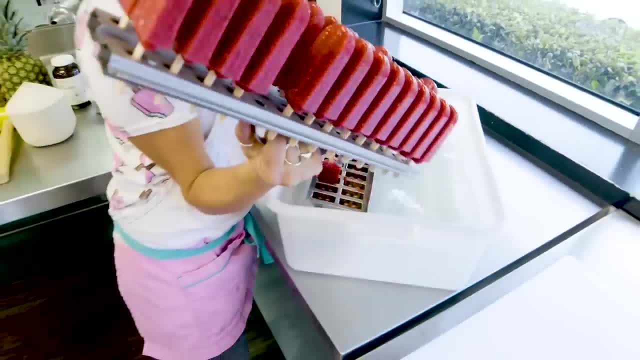 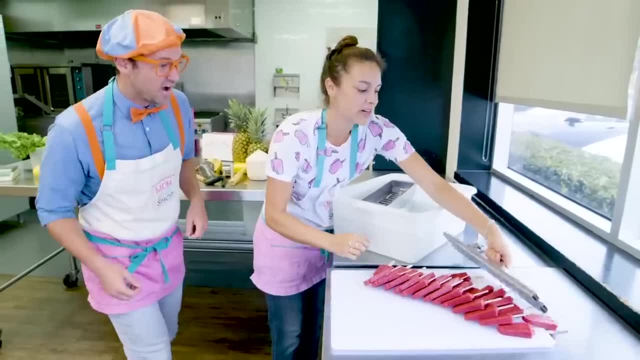 It kind of softens it up, so it comes right out. Oh, lost one. There they are. Those look so yummy. I am so excited. Go ahead, try one. Okay, how about this one? Wow, Ha-ha. 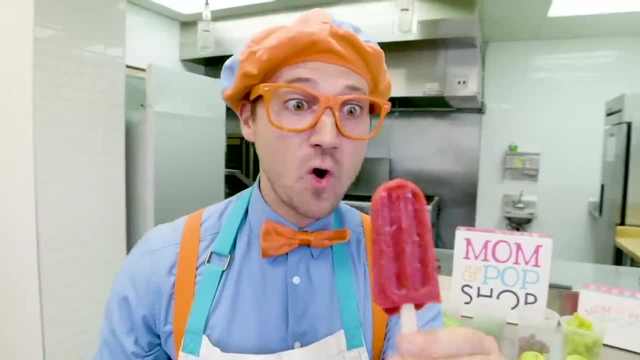 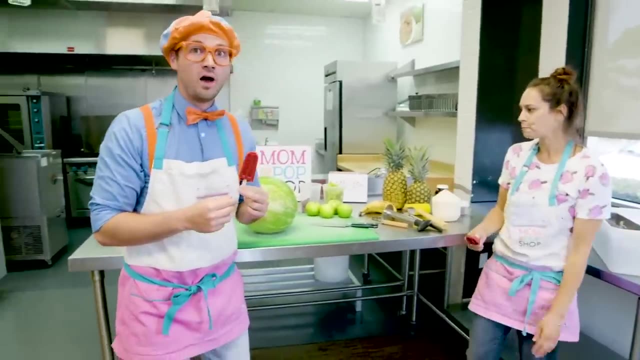 Mmm Yum, That is so yummy, Mmm Yum. That reminds me I got to go back out and sell more Popsicles. Okay, cool, Do you think you could watch the kitchen for me? Feel free to make your own flavor. 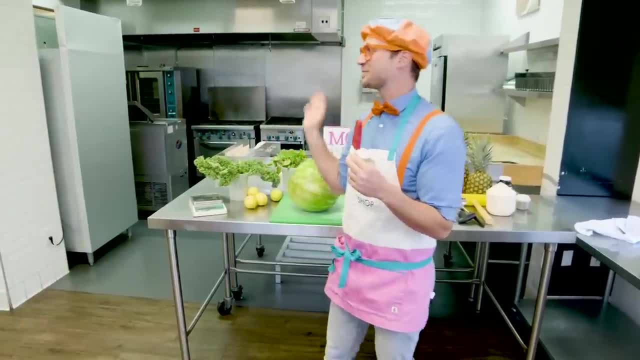 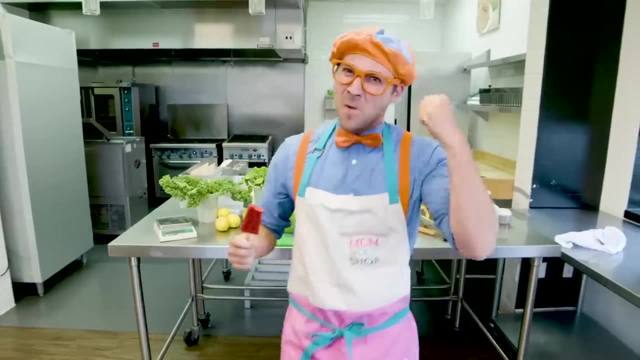 Make our own flavor. That sounds like fun. See you, Blippi. Thanks for showing us around, No problem, Did you hear that You and I get to make our very own Blippi flavor? Let's do this, Woo-hoo-hoo-hoo. 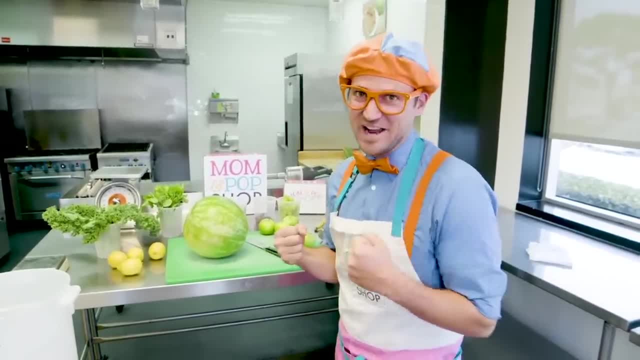 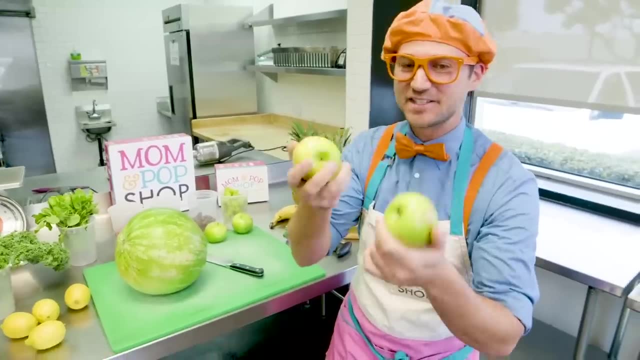 Did you hear that? All right, you and I get to make our very own flavor, and I am so excited. All right, let's see what we have to work with. All right, you know what kind of fruit this is right. 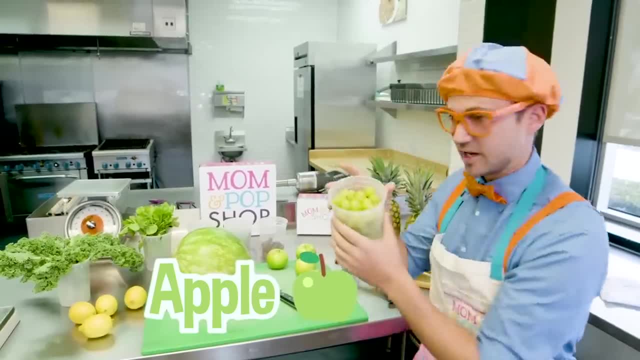 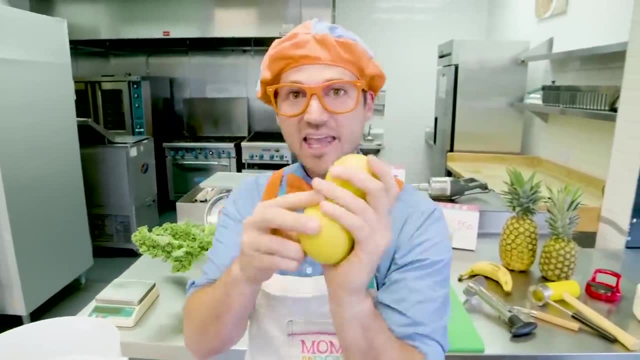 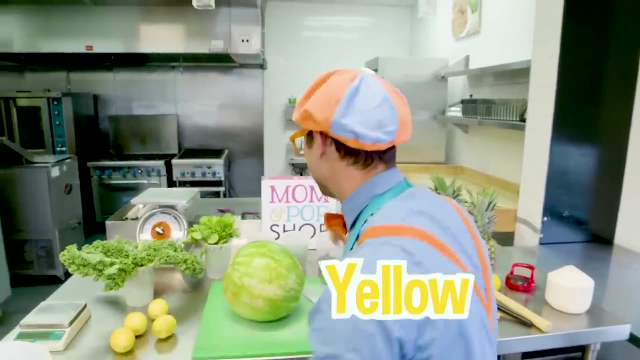 Yeah, This is an apple. Okay, looks like we have some grapes. Yum, Ooh, what are these? Check these out. Yeah, These are lemons. Lemons are the color yellow, Wow. and then we have some greens, over here. 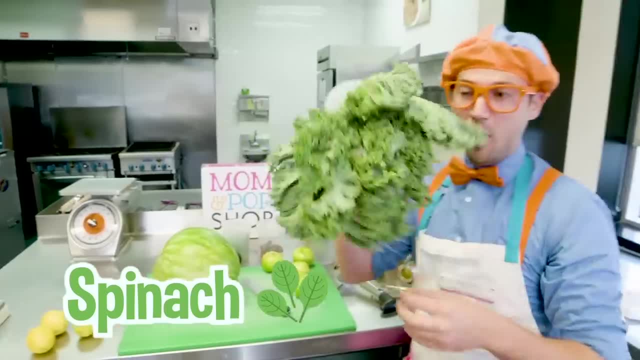 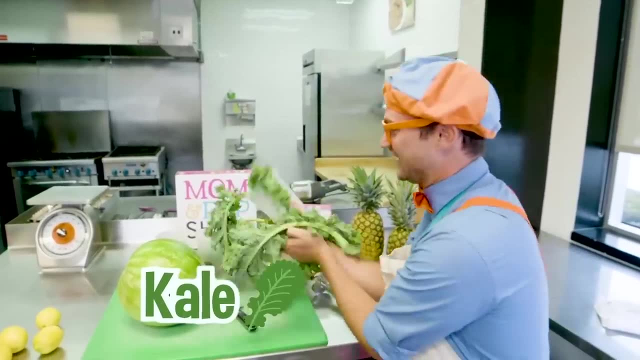 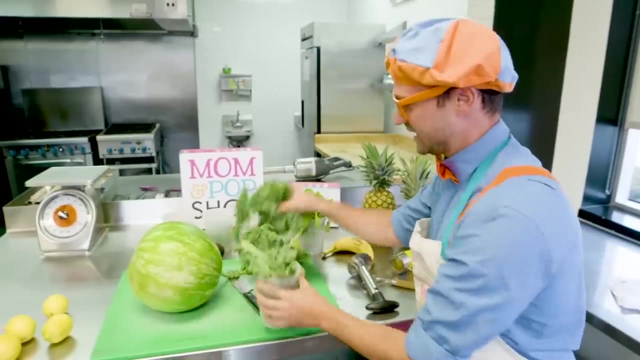 Whoa spinach. Wow, Whoa Hello, It's like hair. Whoa oh, This is kale. Kale is really yummy And it doesn't like containers. That's silly. Okay, let's put these back in here. 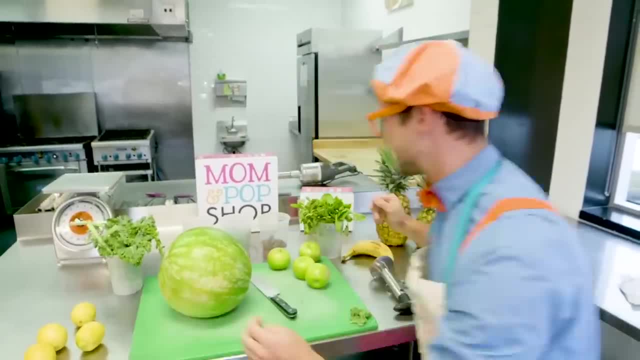 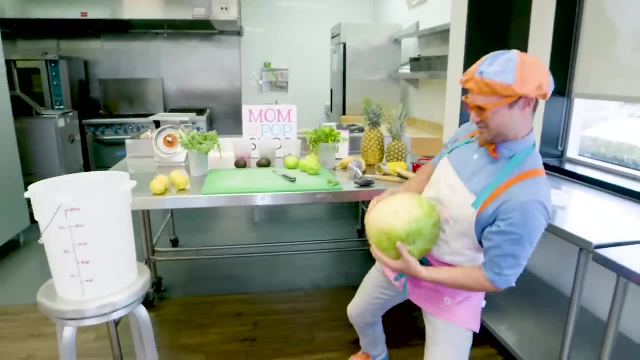 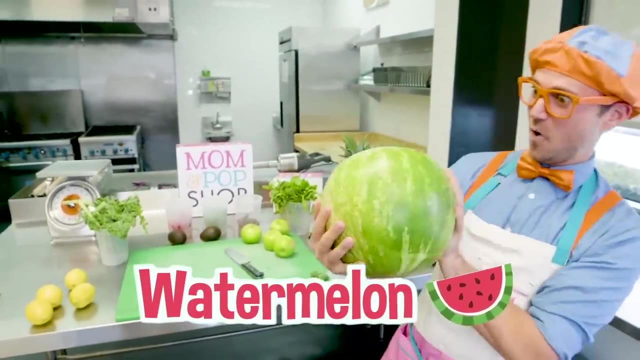 so then we can continue to see what type of fruits and vegetables we have, Like this: Whoa, This is so heavy. Whoa, Whoa, Ugh. Yeah, This is a watermelon, and watermelons are so big and yummy. 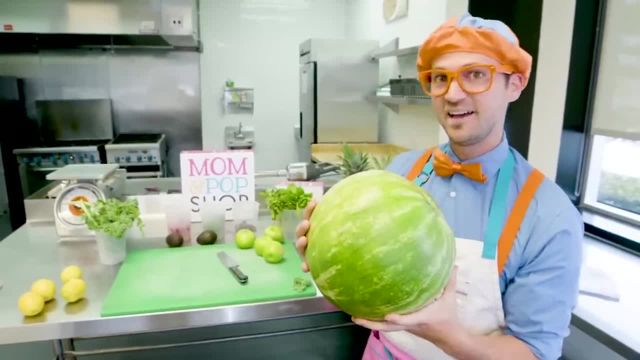 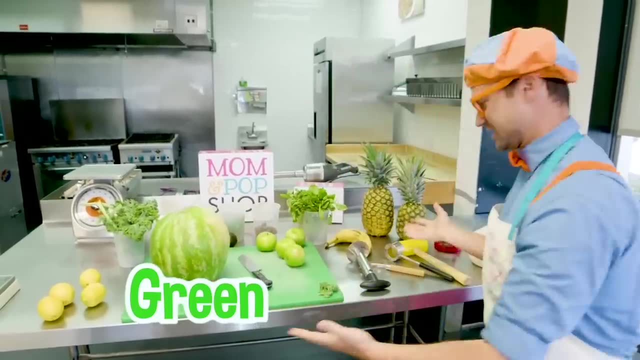 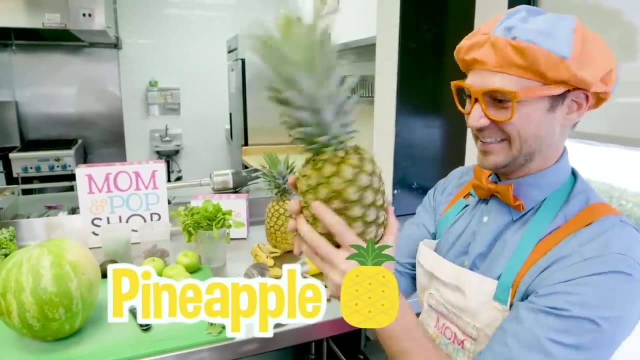 Do you know what color is on the inside? Do you know what color is on the inside of the watermelon? Yeah, red, And the outside is green. Okay, just a couple more Bananas And pineapple, Yum, Okay, so you can see, we have this big bucket right here. 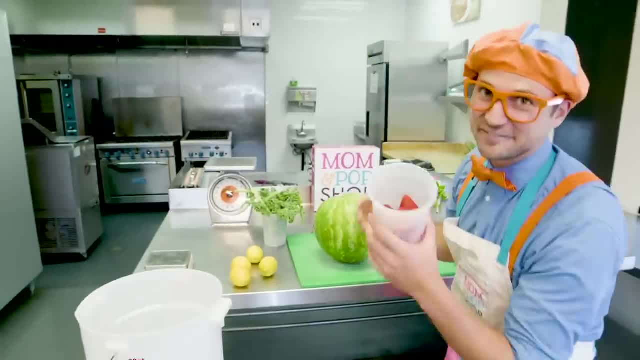 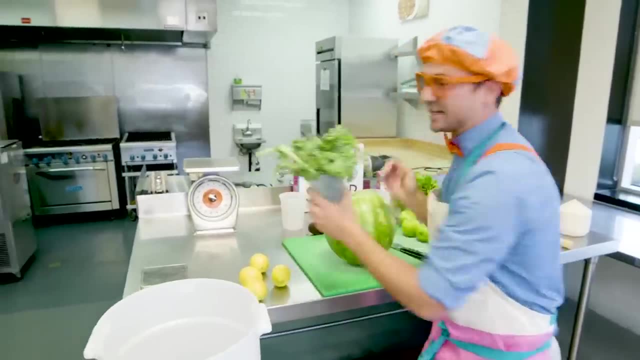 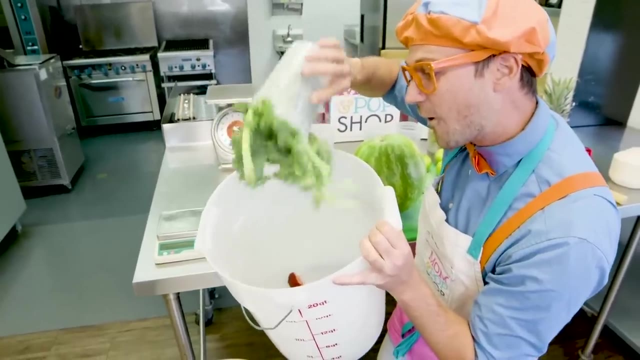 and we need to put a lot of the ingredients right in here. Can't forget about the strawberries. We'll start with those. Here we go, Woohoo. Okay, that kale? Whoa, Let's put some in there, Woohoo. 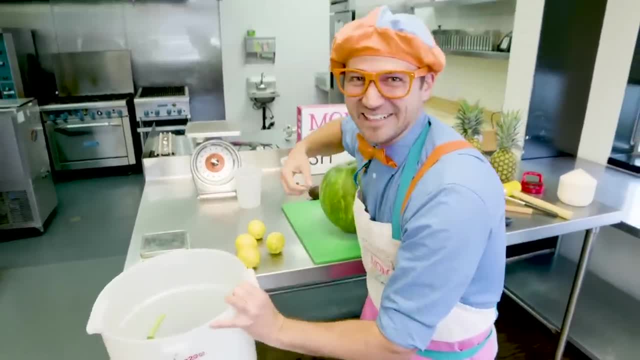 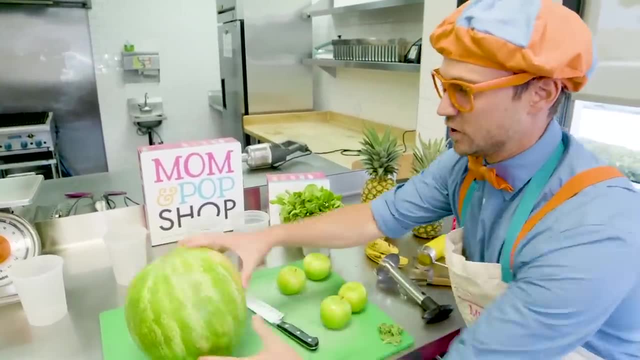 Woohoo, woohoo, woohoo, woohoo, Woohoo. We are doing so good. Oh, apples. Okay, we could put the whole apple in there, but I think we should probably slice it. Have you ever had a slice of an apple? 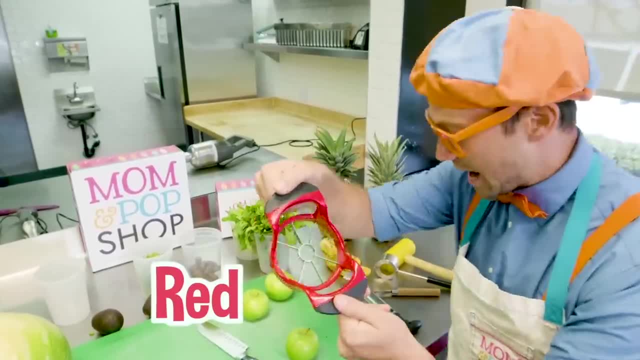 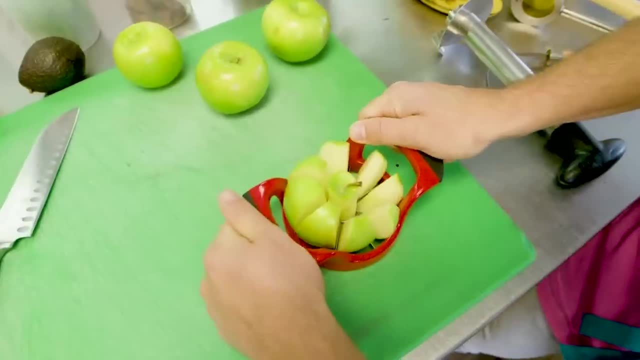 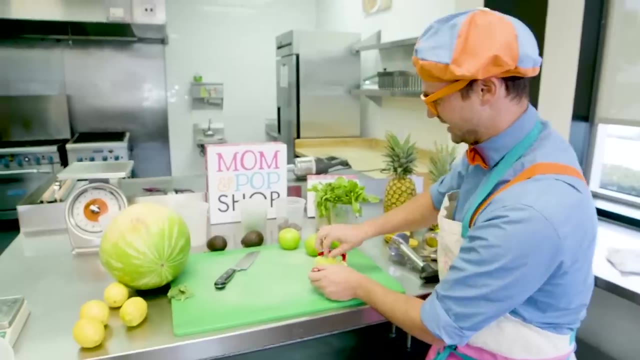 They're so yummy. Okay, So here is our red apple slicer. And then put it right in the center, just like that, And then you push down: Whoa, Look at that, That is awesome. Slice the apples, so then you pull them out. 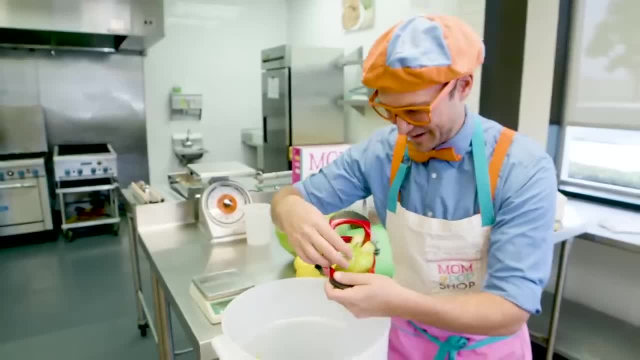 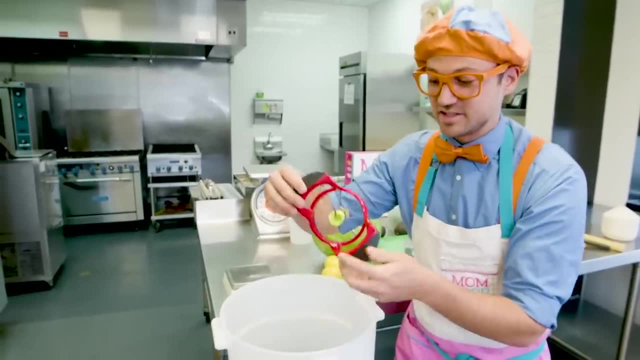 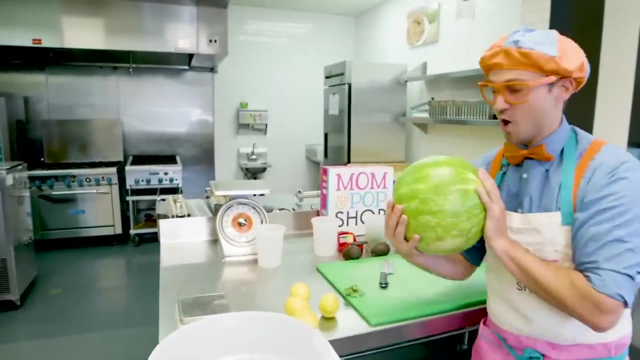 and then you can put them right in our big bucket. Wow, And you keep the core. whoop, you keep the core, which is the center out of it, Because there's a lot of seeds in there. Speaking of seeds, watermelons have seeds. 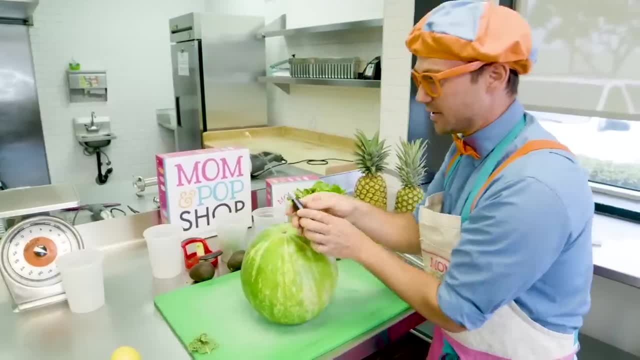 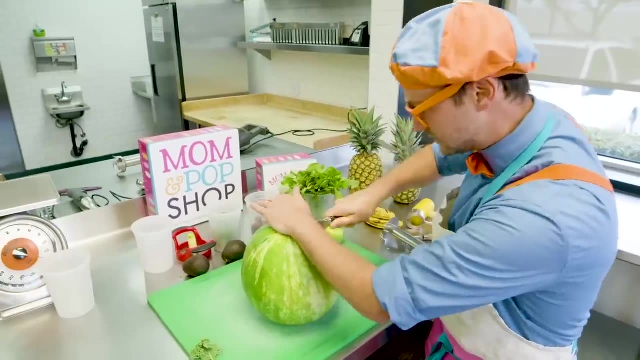 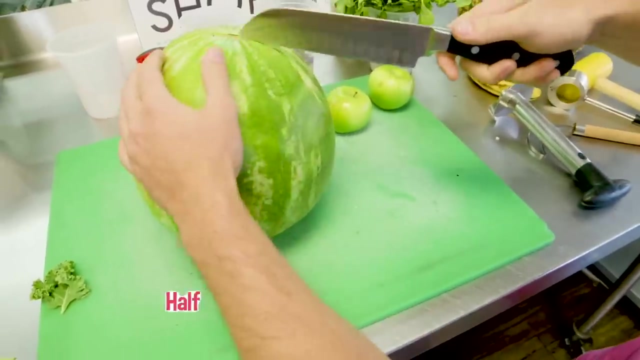 Okay, Let's cut open the watermelon. Whoa, I'm going to be very careful because I'm a grownup- with this knife Ready. Okay, Here we go. Chop it in half just like that, Flip it around. 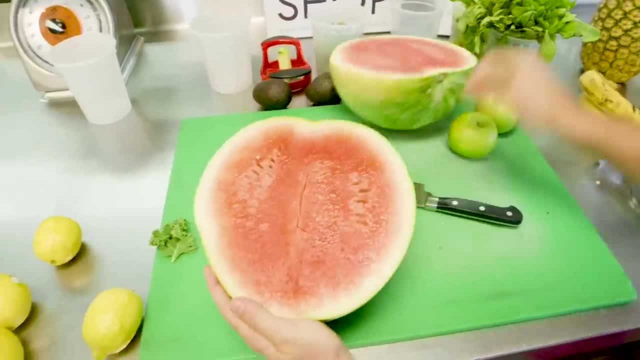 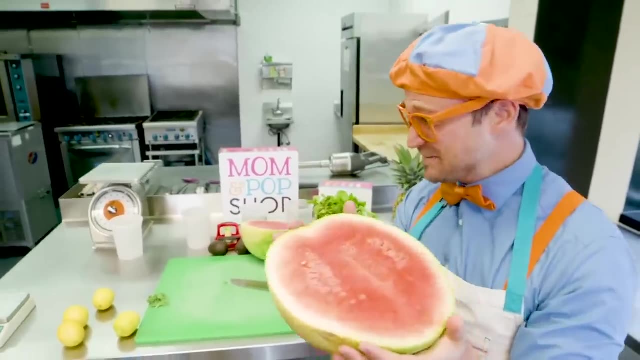 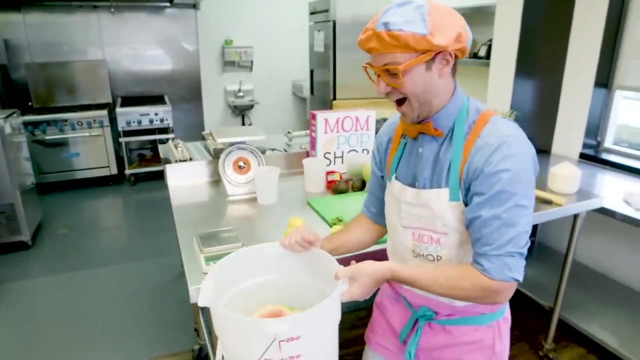 Whoa, There we go, There we go. Wow, Look at that, That looks so yummy. Our popsicles are going to be so yummy. Okay, I have an idea. Here we go. All right, We have some bananas. 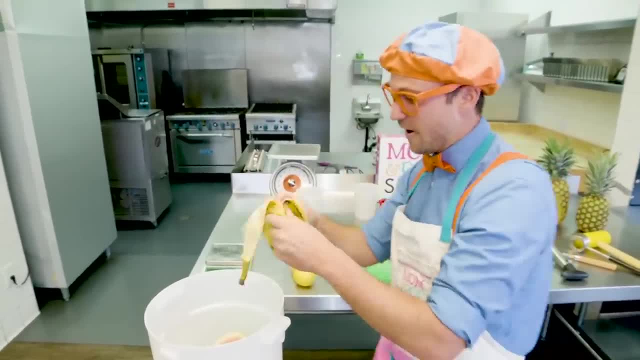 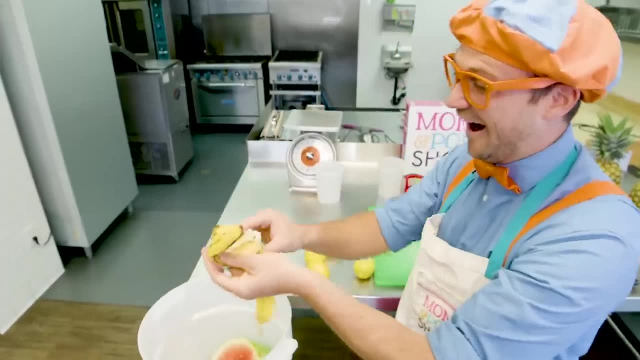 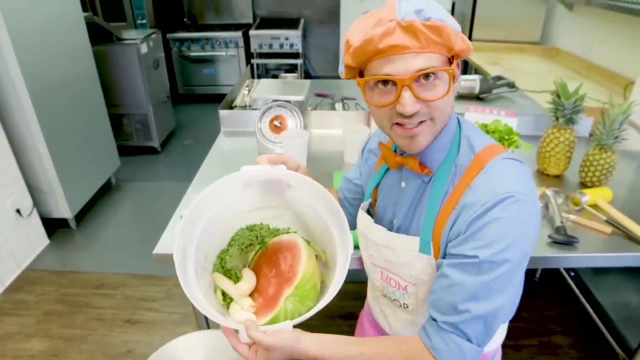 Open those up. Here we go, Bye-bye. banana Woo-hoo, And we'll do another banana Yum, Here we go. Yum, Look at it. Is that looking tasty? Or does that look tasty? Whoa? 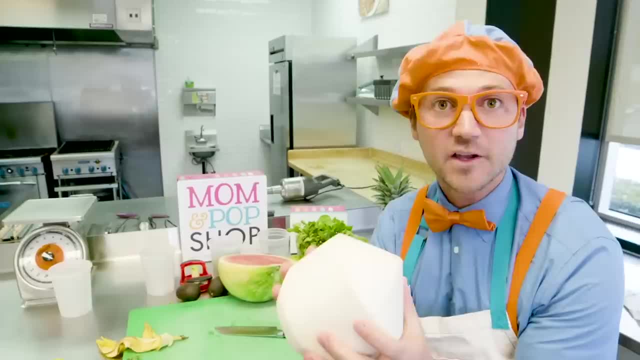 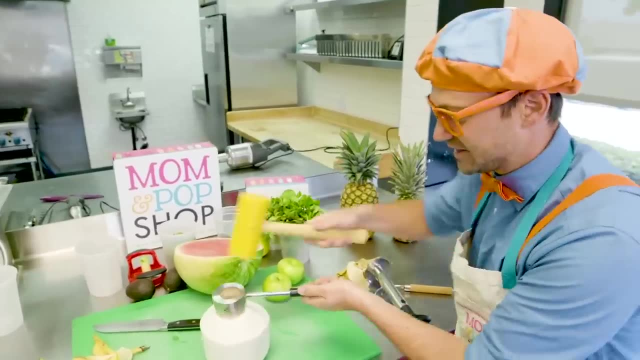 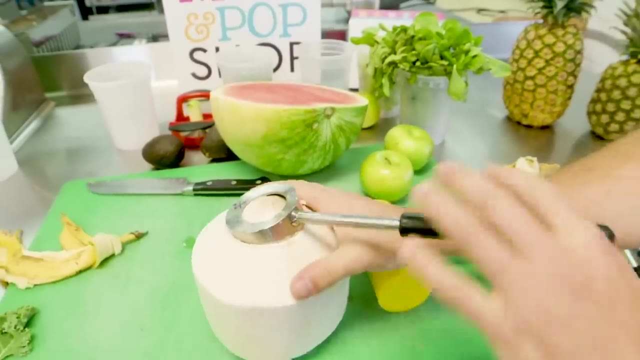 And remember we learned what fruit this is. Yeah, the coconut. All right, These are a little tricky to open, but it's worth the trouble, So let's take the coconut opener. Whoa, We did it. Look at that. 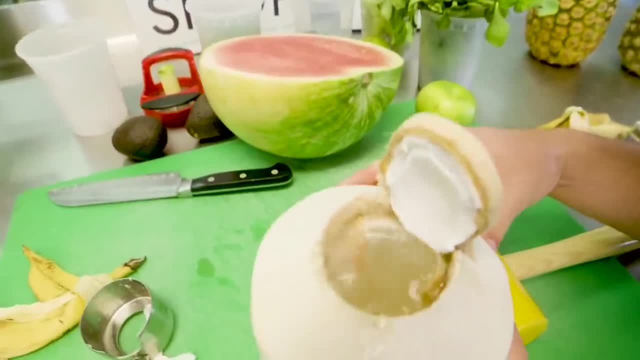 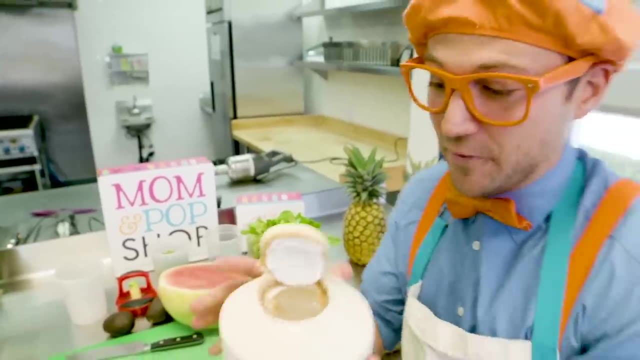 Whoa, Whoa. Look at all that liquid. I just want to drink it all up. Oh, Okay, We'll put that in the bucket. fur The popsicles. Whoa Yum, Okay, Use this little coconut device and pull out some of the coconut. 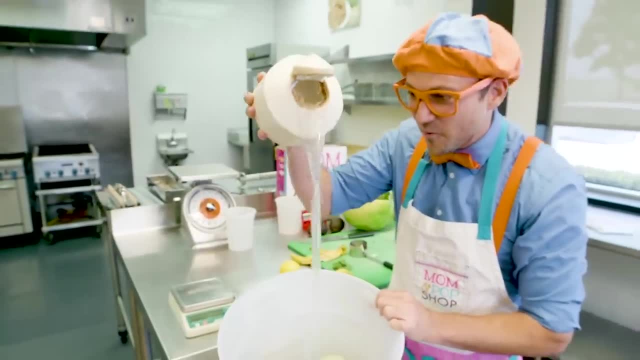 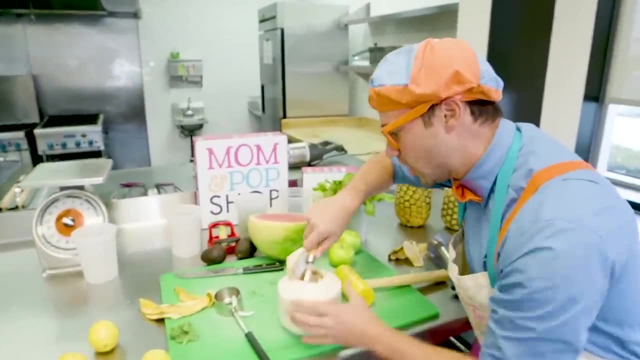 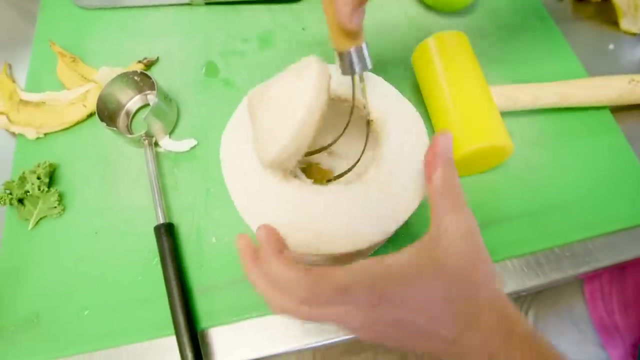 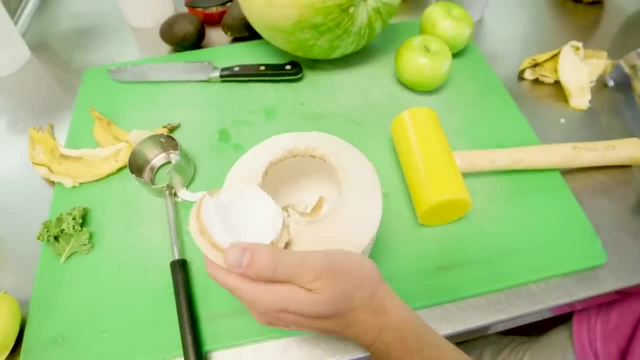 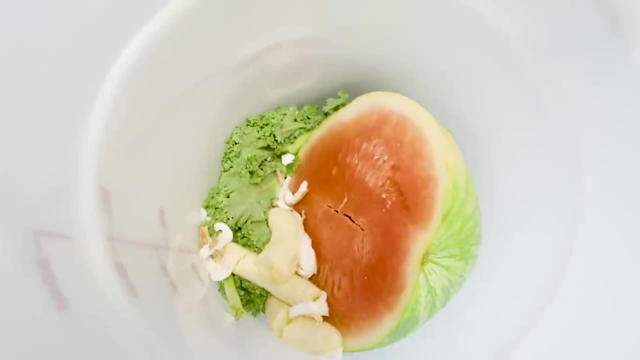 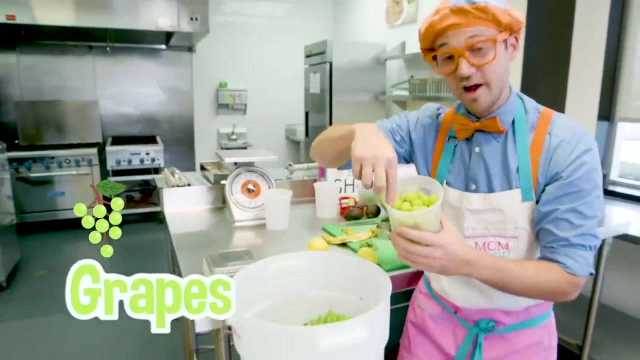 All right, Perfect, Let's bring it right over here. Yum, All right. Oh, Spinach right here. Whoa, And then we have a bunch of grapes. We'll do one, two, three, four, five, six, seven, eight. 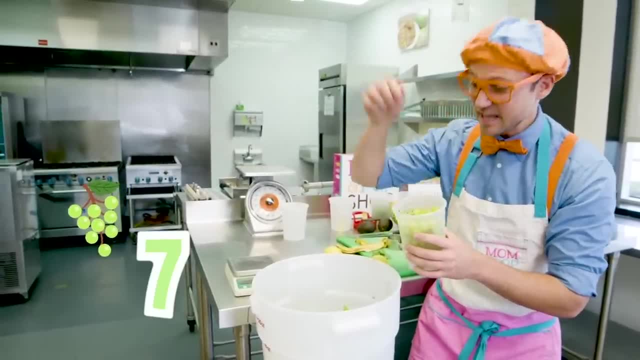 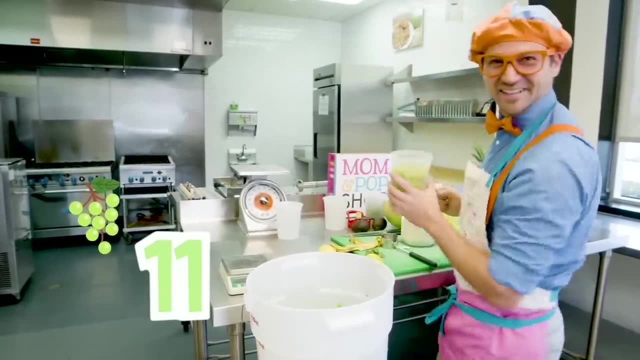 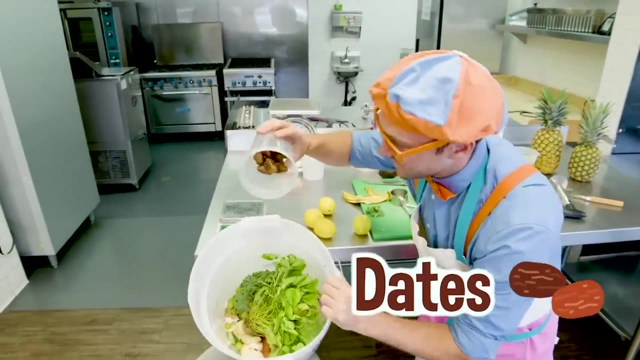 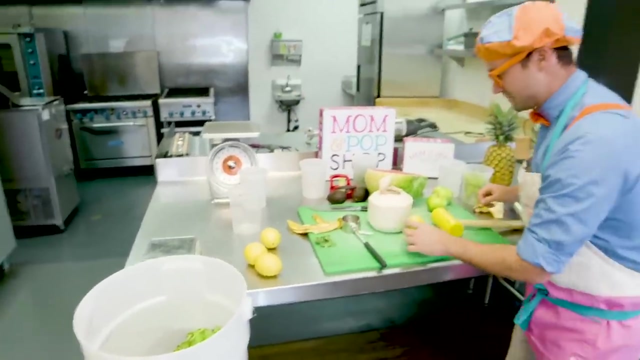 Oh, 5,, 6,, 7,, 8,, 9,, 10,, 11 grapes. All right, And then remember these. we used these earlier. These are dates. Here we go, Whoa, Okay, can't forget about the lemons. 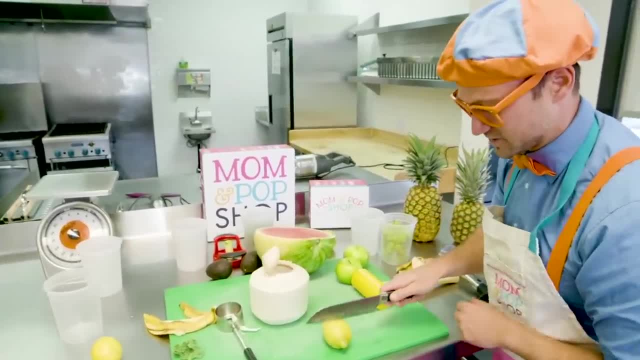 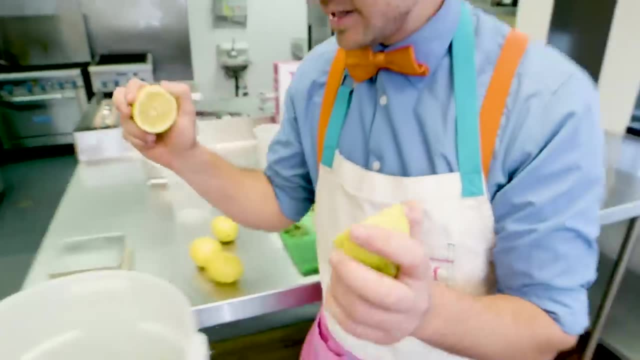 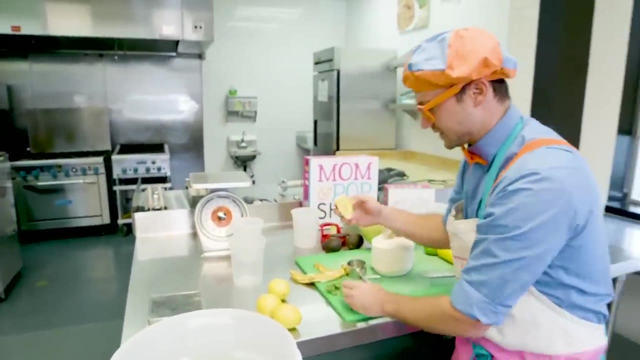 We have so many types of fruits and vegetables in here, Here we go. Wow, Okay, let's take these and give a little squeeze. Woo-hoo. Have you ever tasted a lemon before? Okay, let's try some. Whoa. 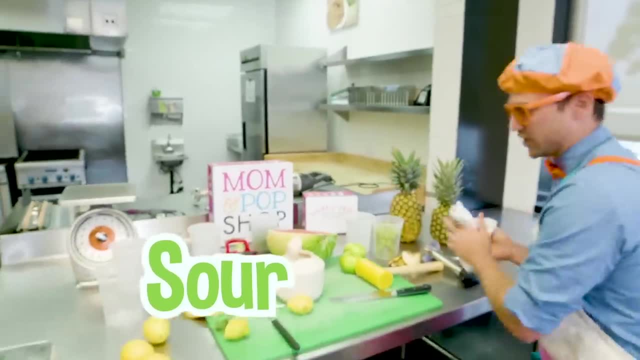 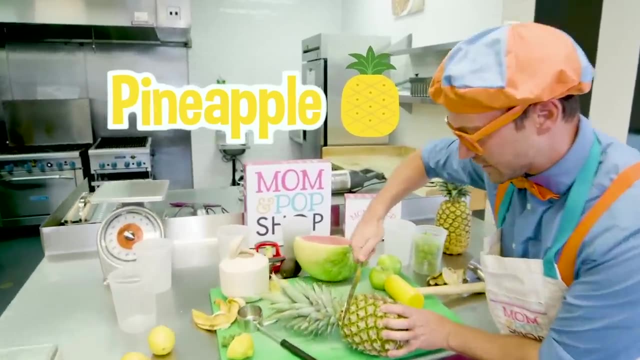 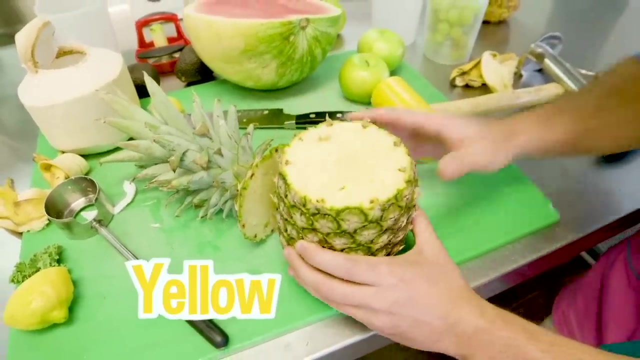 Whoa, That's sour. Okay, let's wash our hands. And then, last but not least, we have a pineapple. We cut the pineapple, Just like that, And you see that yellow That looks so yummy. So now we take this pineapple tool, put it right on top. 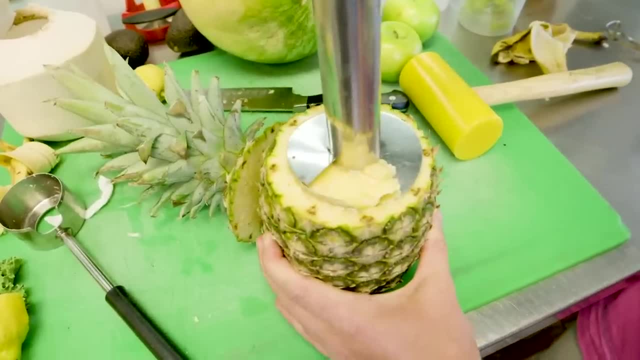 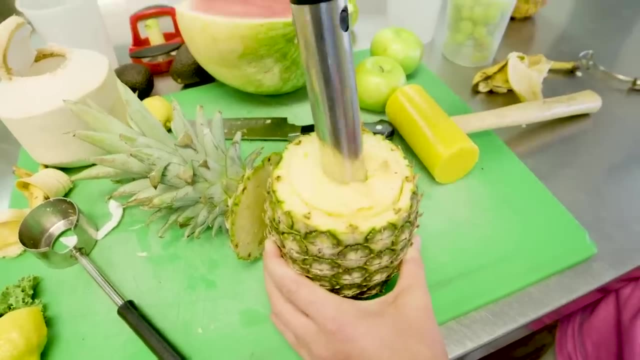 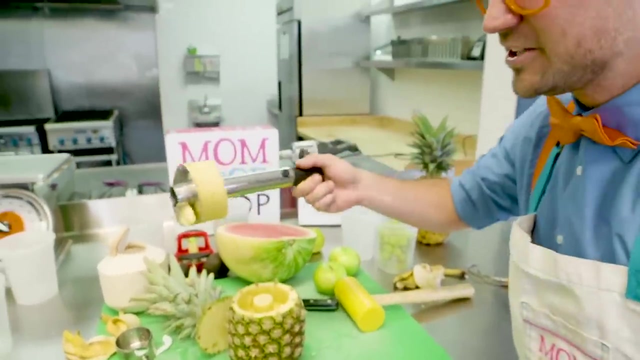 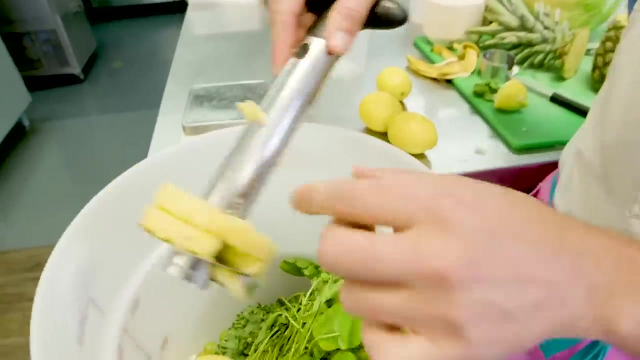 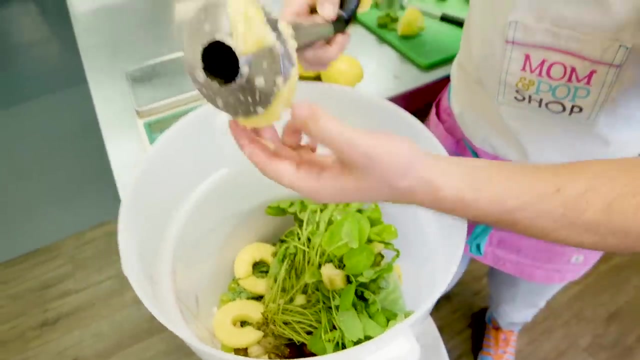 And then give it a little twist- Wow, Look at that. And then you pull it out- Whoa, Check this out, Check that out. And then take it off, just like this, And that's going to give it some nice sweetness to these yummy popsicles. 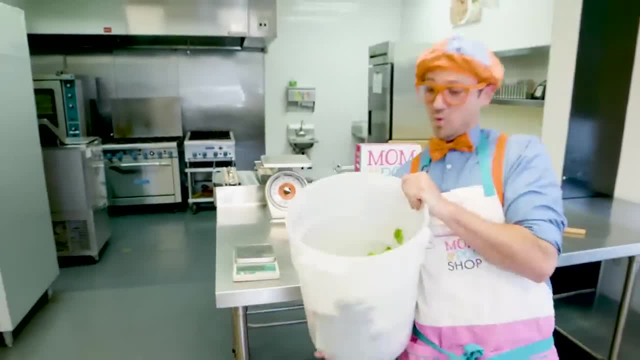 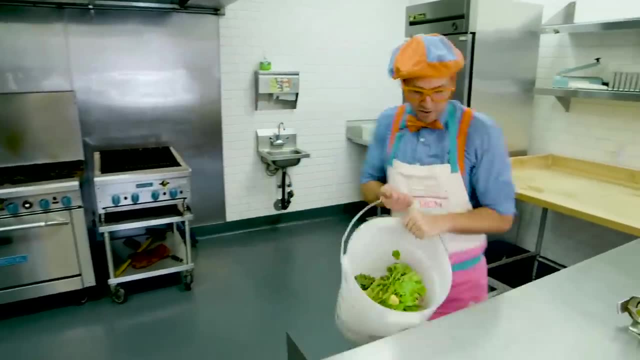 All right, I think that's plenty. Look at Whoa, That's so heavy. Come on back here. Remember that next step that we do. Yeah, she taught us that. you put the bucket right here, You take the big blender. 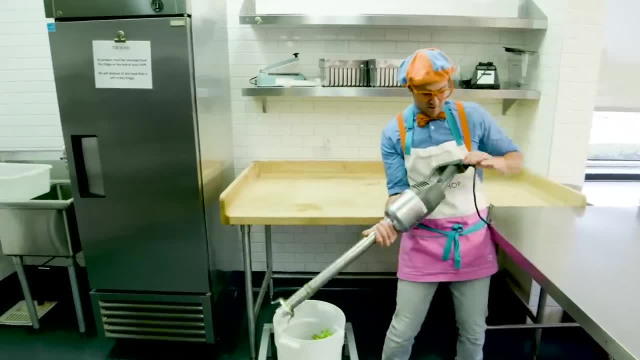 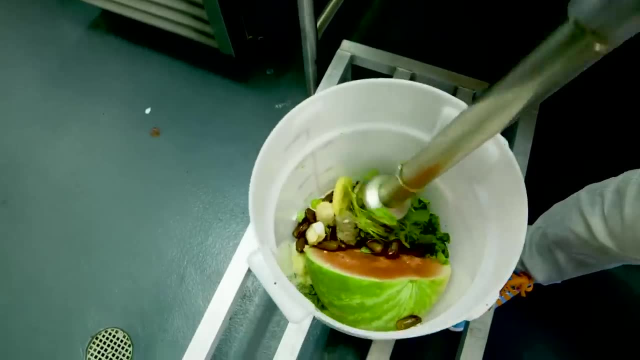 Whoa, Whoa, And we blend it up. Here we go. Whoa, All right, Now it's all mixed up. Wait a second, though. We need the magic tool. This is a giant whisk. Whoa, Whoa. 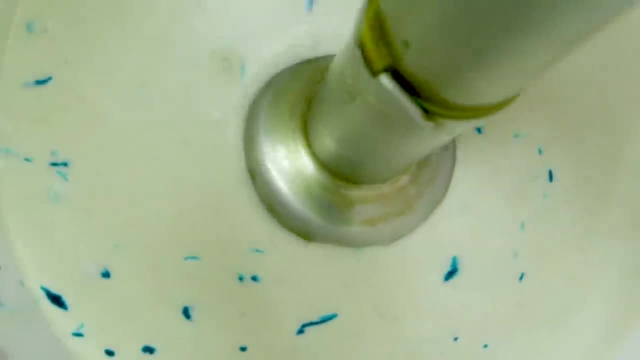 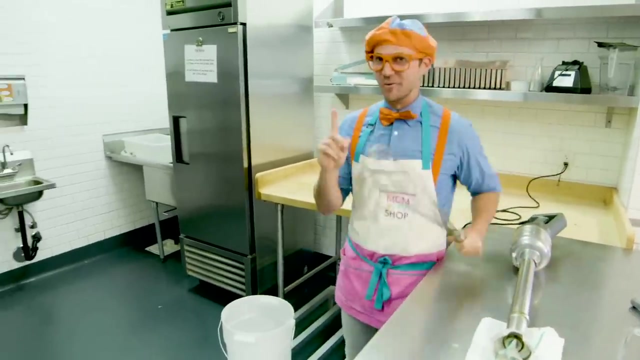 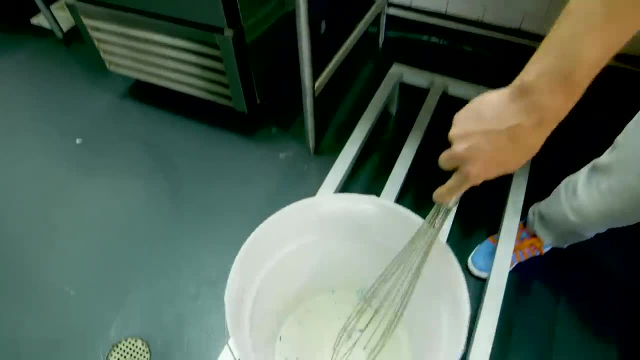 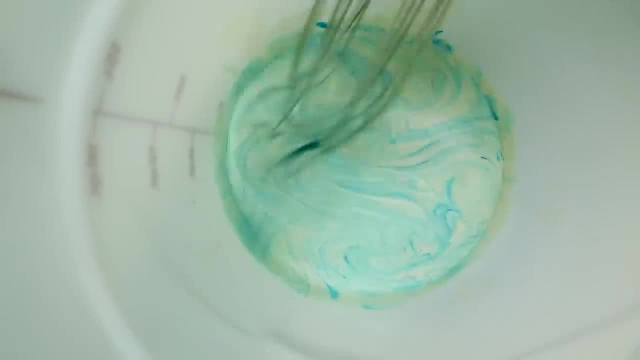 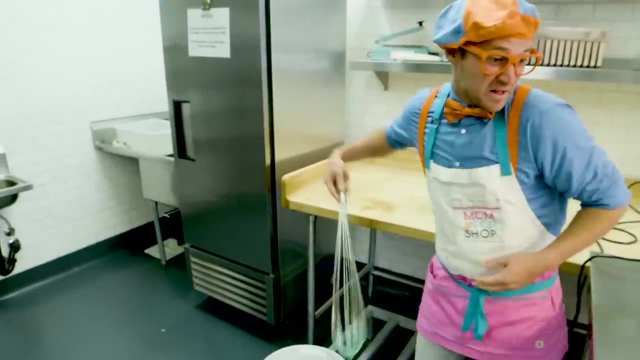 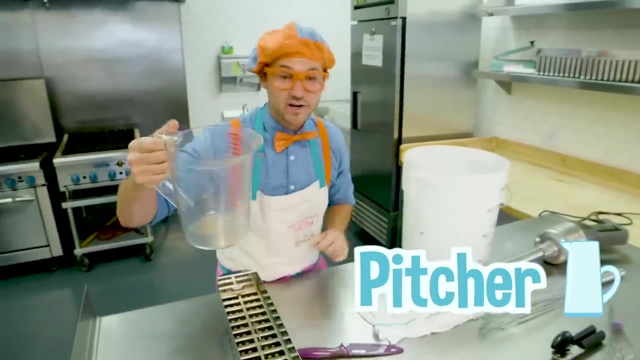 Whoa, Check this out. All right, It's adding some color. Okay, Let's put this right over here And then we can bring this up and grab this pitcher. Remember from earlier: We need to scoop some out, Whoa. 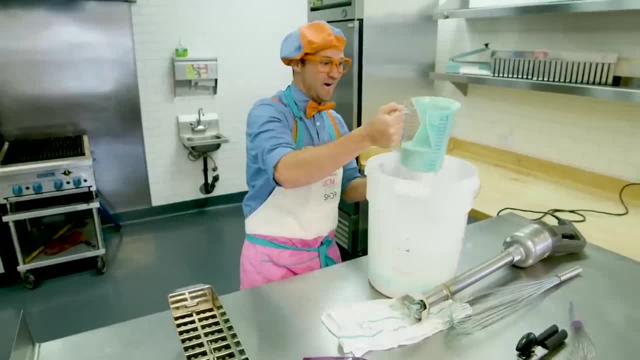 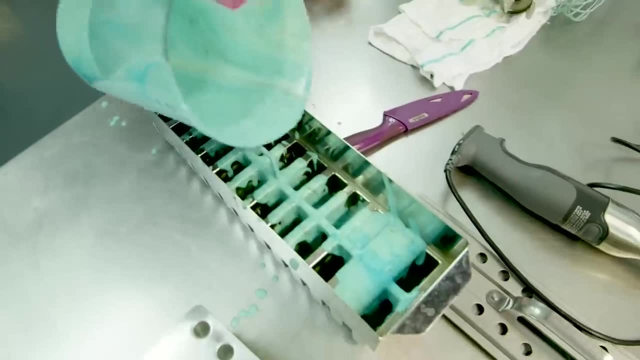 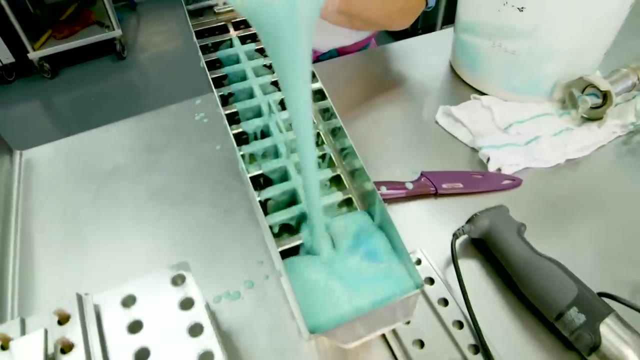 Whoa, Whoa, Whoa, Whoa. I am so excited. Pour some in, Let's grab another scoop. Okay, here we go. Okay, Whoa, All right, I think that's plenty. Let's give it a shake. 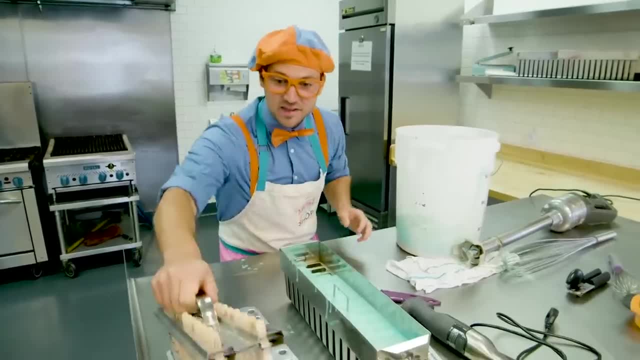 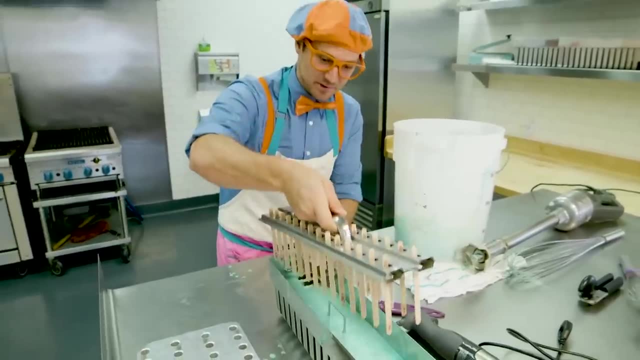 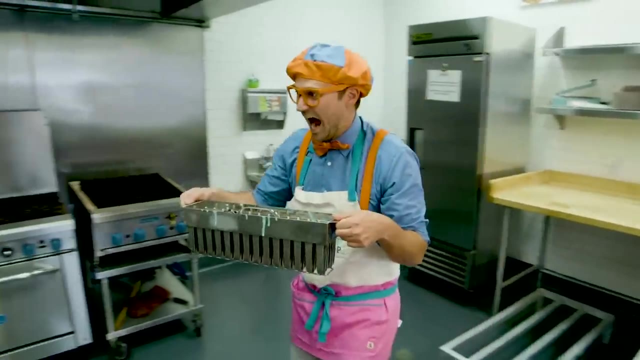 Okay, yes, These are gonna be so yummy. Let's take these sticks. Wow, That's a lot of Popsicle sticks. Put them right in there, Perfect, Okay, now we need to bring it to the cooling station. Here we go. 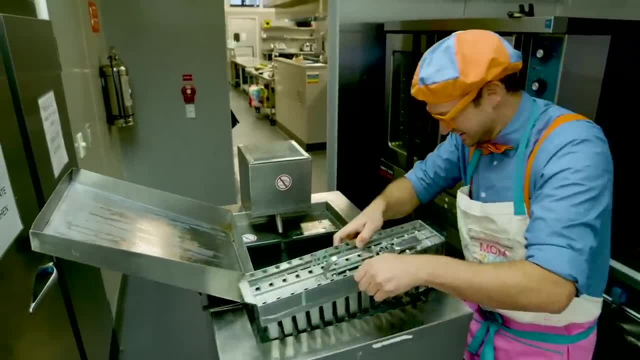 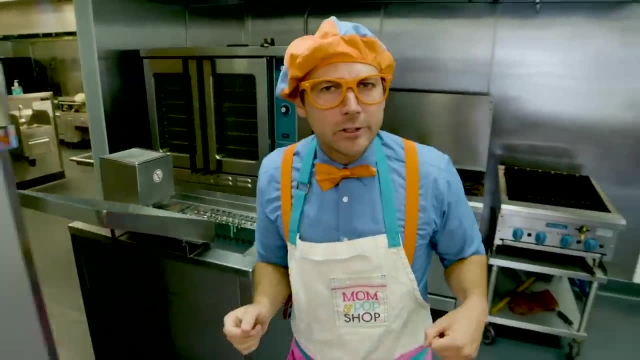 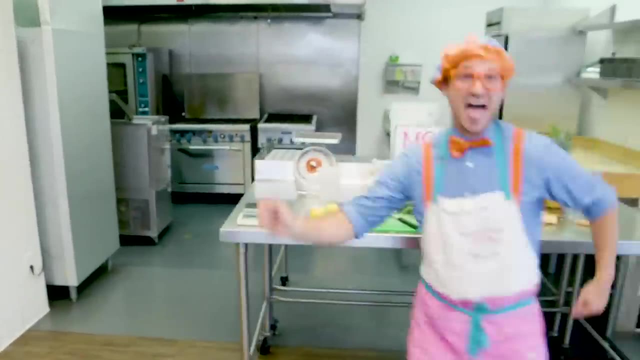 Set it down. Woo-hoo, we did it All. right now, remember what we had to do earlier. It's gonna take a long time, So we get a dance while we wait. But now let's do the last thing. 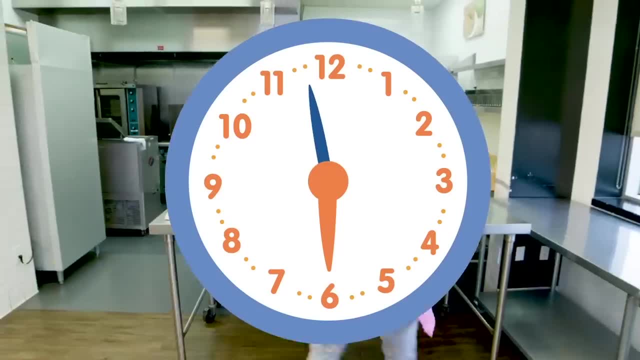 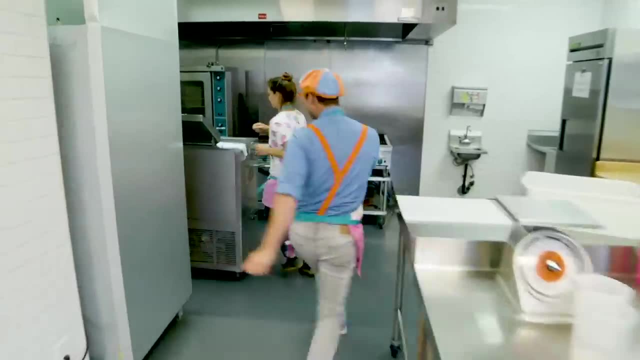 Okay, this is where we roughly know what we're gonna use. The soy sauce. Okay, let's do the soy sauce. Woo-hoo, that's gonna be pretty good. All right, let's do that again. Did I use Carradine? 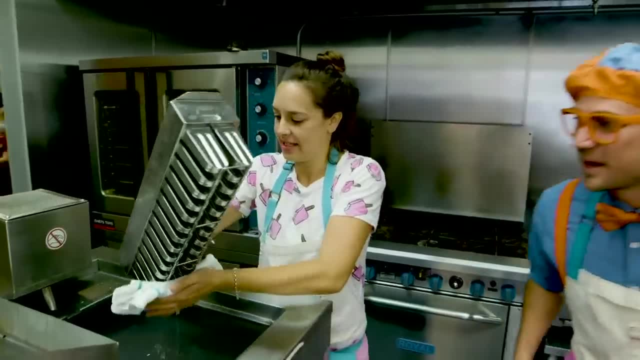 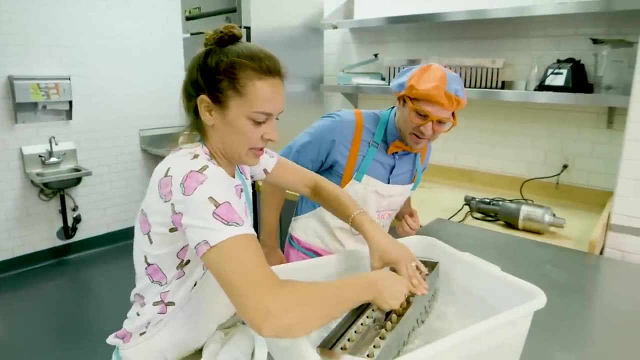 Ooh, you sure did. The Popsicles must be ready. Let's check them out. Woo-hoo, All right. Whoa, I am so excited. Hey, we gotta drain them. I can't wait to see the ingredients you used. 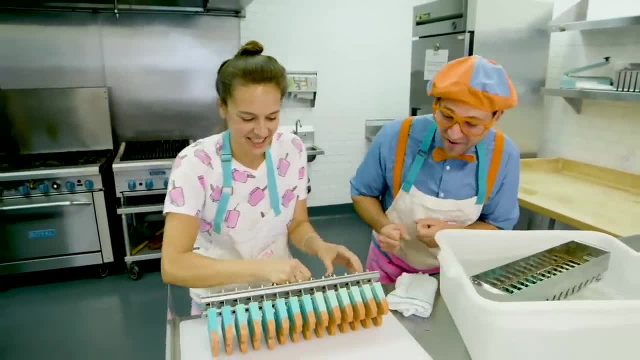 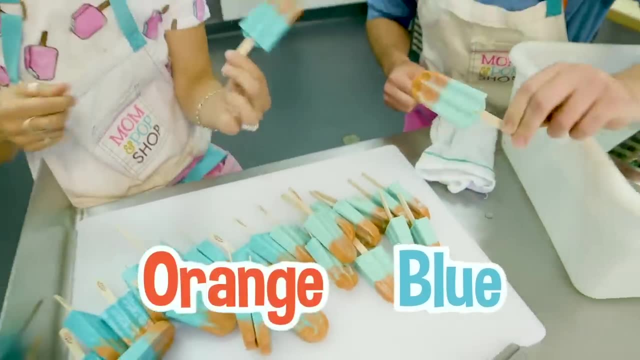 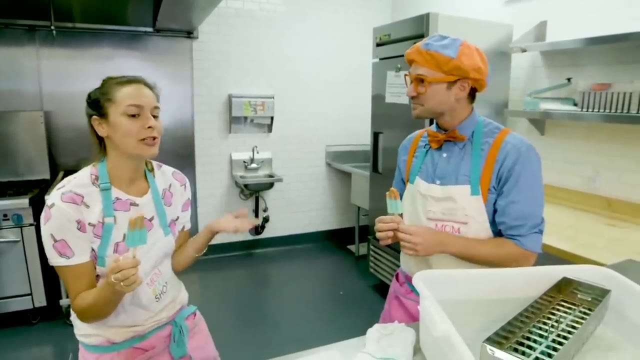 Whoa, Look at them. Whoa, My two favorite colors: Yeah, Check them out. Blue and orange: Shall we try them? Yeah, Mmm, Do you like them? These are delicious. Flippy, You know what You need to take those outside and go sell some pops. 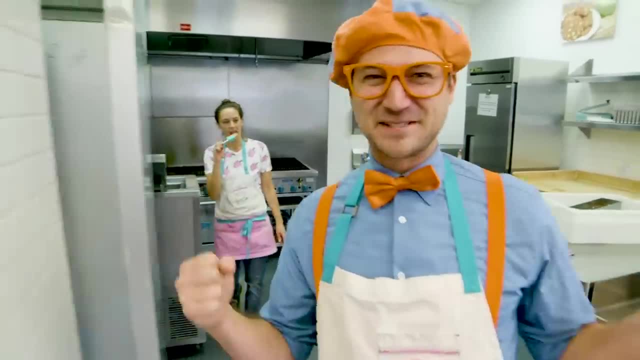 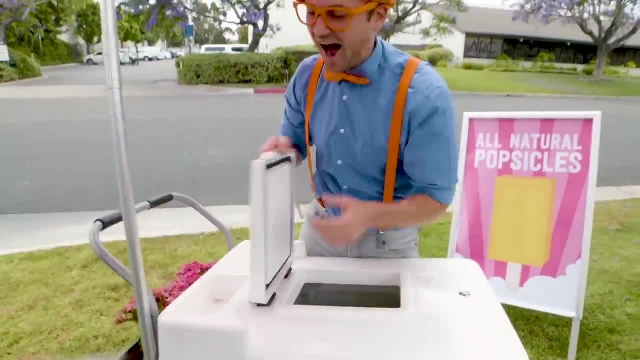 Mm. Awesome, Alright, let's go try some. Sell some popsicles, Popsicles, Popsicles, Popsicles. Who wants a popsicle? I love popsicles And that was so much fun learning about how to make popsicles. 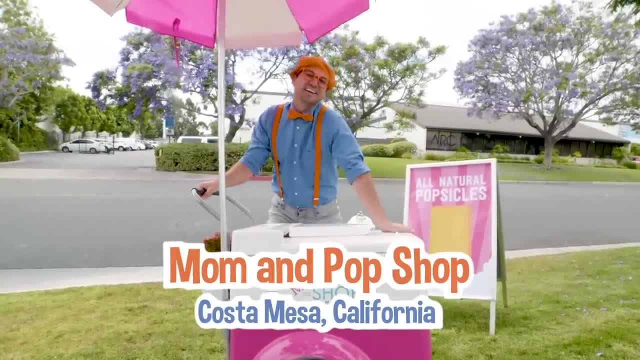 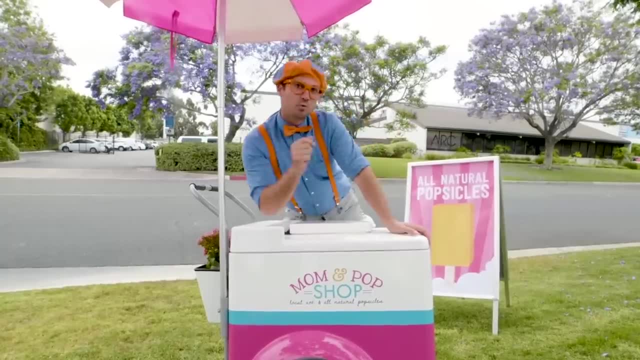 with you at Mom and Pop Shop in Costa Mesa, California. Well, this is the end of this video, But if you want to watch more of my videos, all you have to do is search for my name. Will you spell my name with me? 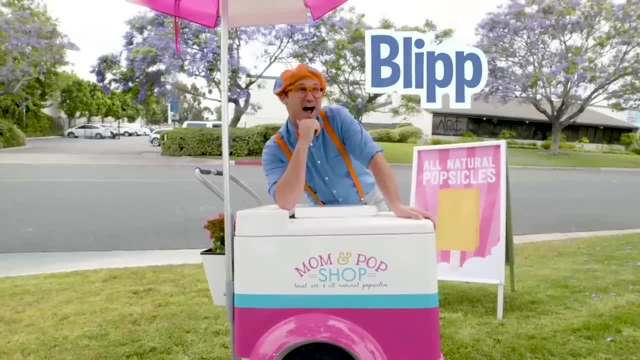 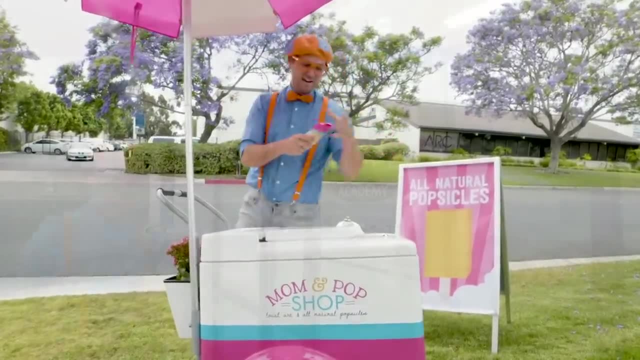 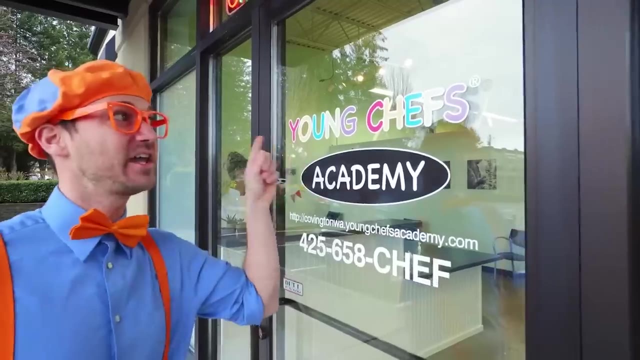 Ready B-L-I-P-P-I. Flippy, Good job. Well, see you later. Bye, Hello, Hey, It's me Flippy, And look at where I'm at Whoa Today I'm at Young Chefs Academy. 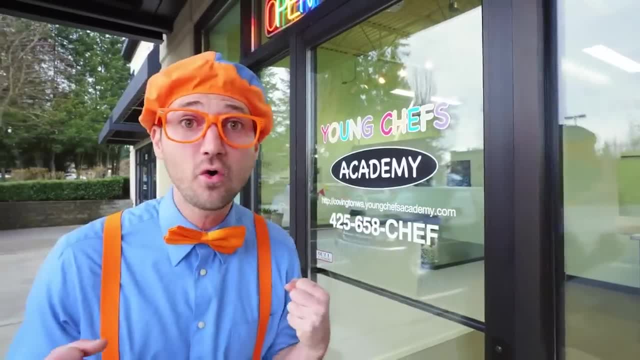 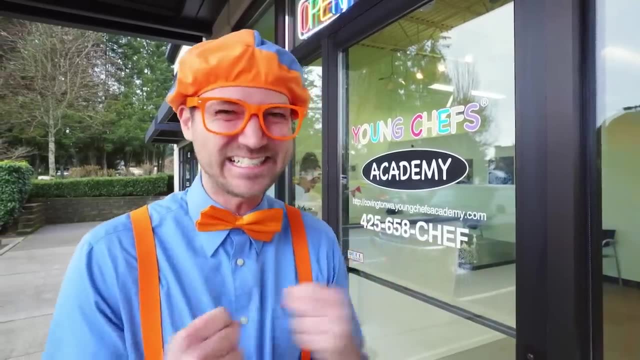 in Covington, Washington. This place is so cool, Yeah, where young chefs, kids just like you, can come here and learn to cook some delicious treats. Ha-ha, Let's go. Hi, Flippy, Hey, Who are you? 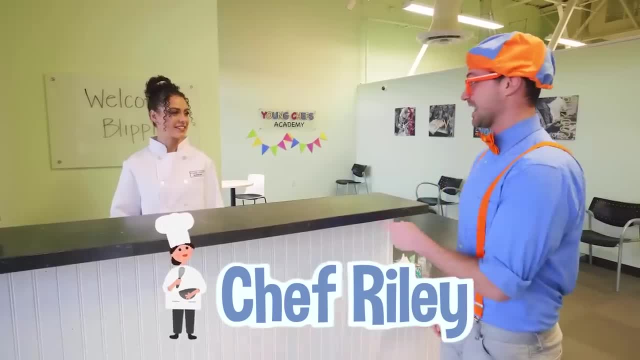 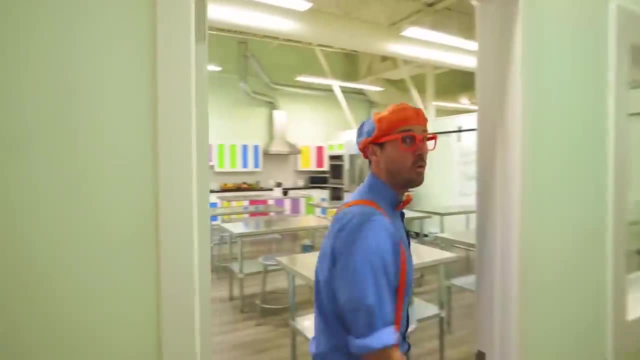 My name's Chef Riley. Oh nice to meet you, Chef Riley. Hey, do you mind if we go explore the kitchen, Go for it. I'll see you in a sec. Okay, Let's go. Wow, Look at this kitchen. 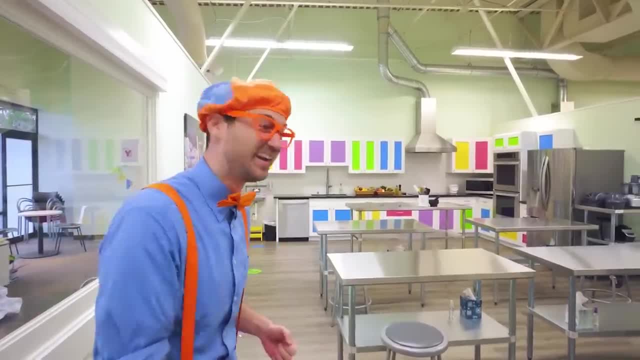 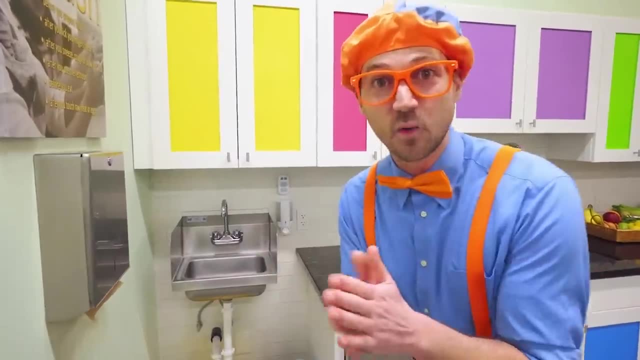 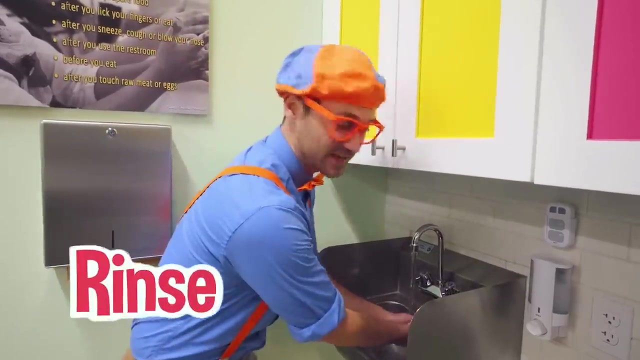 It is so bright and colorful. Whoa, Come on. Okay, the very first thing that I need to do when we enter a kitchen is wash our hands. Okay, I'm gonna turn on hot water And then I'm gonna rinse them. 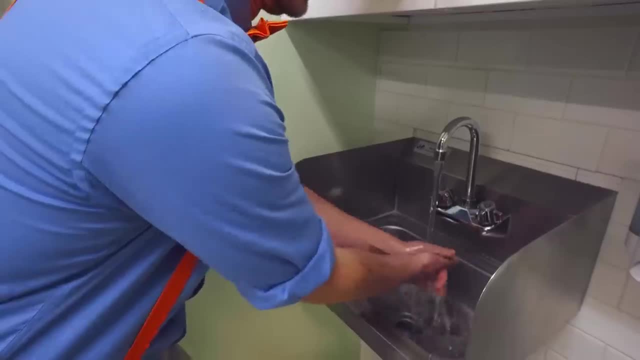 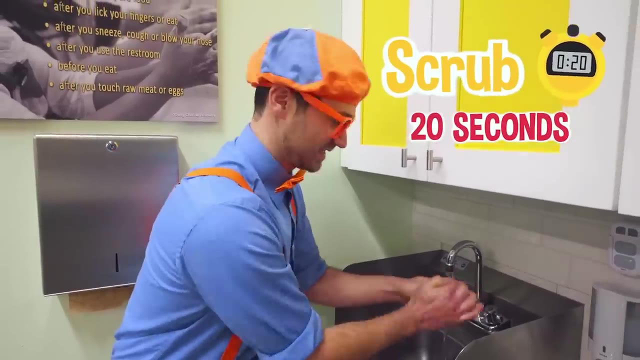 Okay, get them nice and clean. Okay, get them nice and clean, Get them nice and moist. And then we need some soap, Okay, and we need to scrub for 20 seconds, And one way to do this is to sing the ABCs. 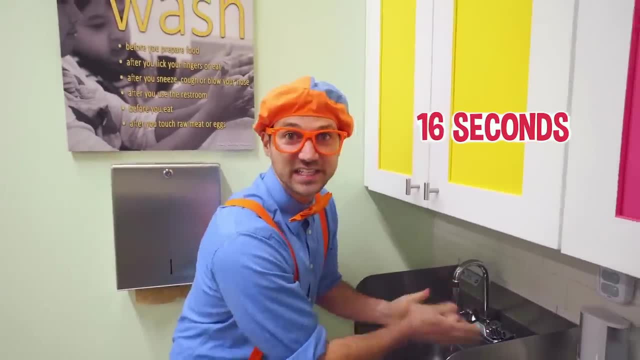 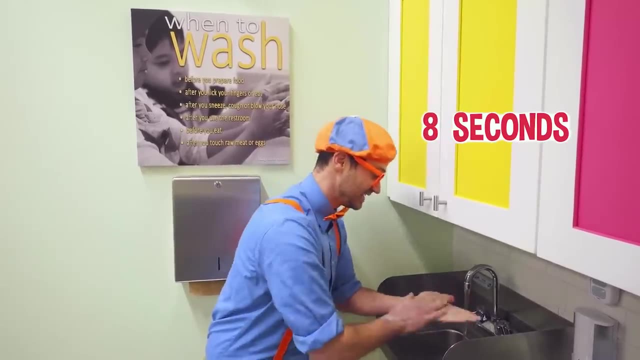 Ready A, B, C, D, E, F, G, H, I, J, K, L, M, N, O, P, Q, R, S, T, U, V, W, X, Y and Z. 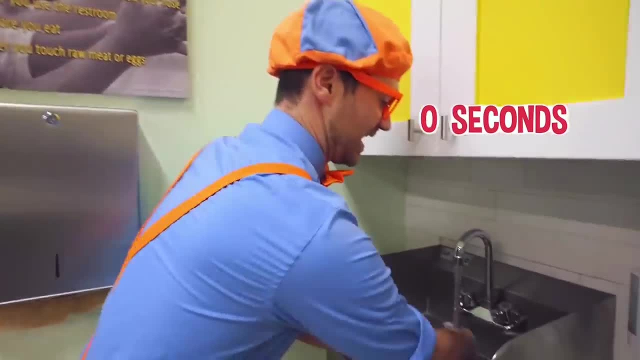 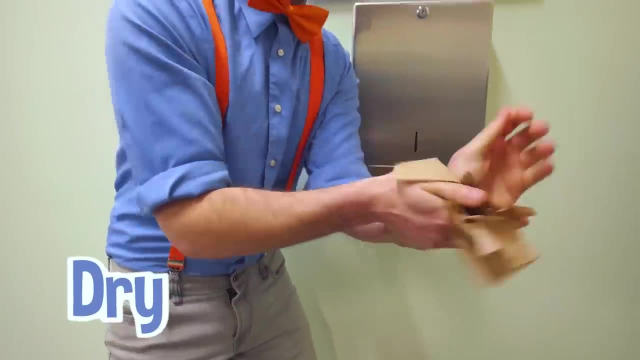 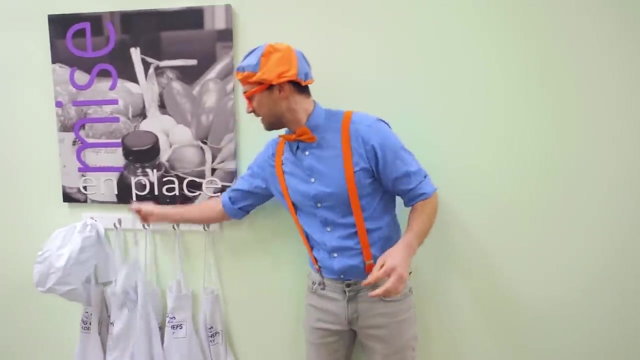 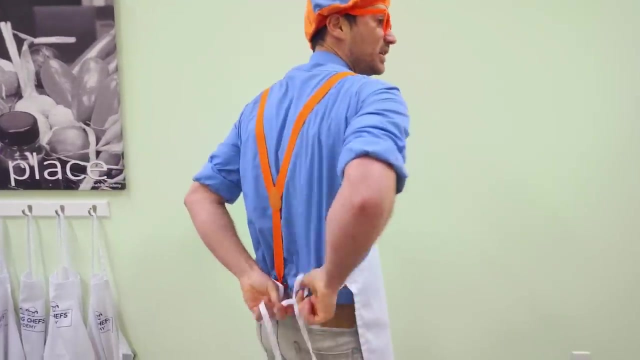 Ha-ha. Okay, Now we're gonna rinse off our hands. Let's get them nice and dry Now. once our hands are dry, clean, now we can put on an apron. Yeah, an apron is used. so then, clothes not get dirty. 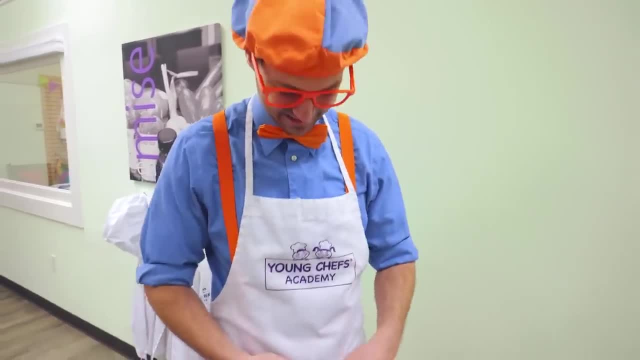 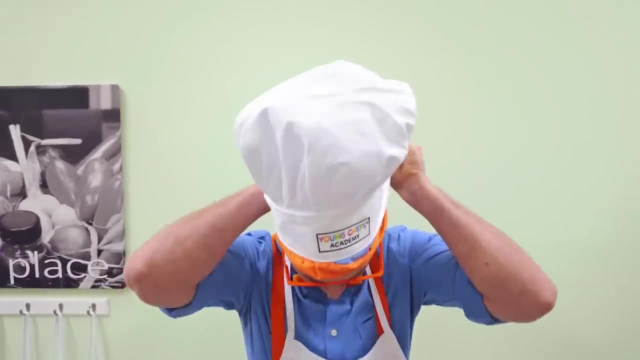 when you're cooking with some food, All right, And can't forget my young chef's academy chef's hat. How do I look? All right, Check it out. This kitchen is so colorful. Do you see all these cabinets? 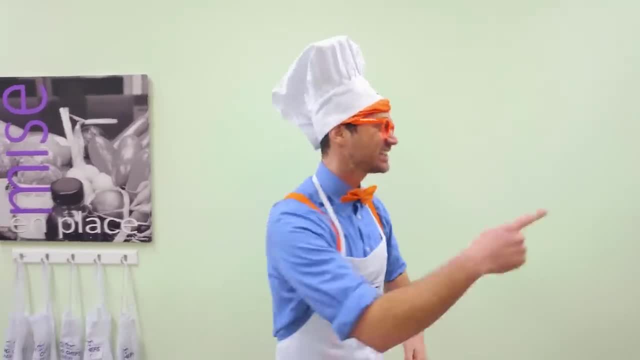 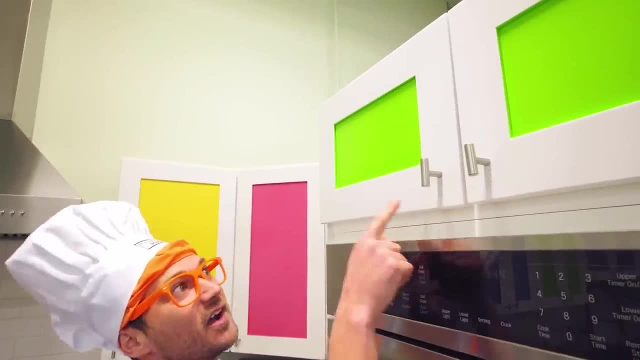 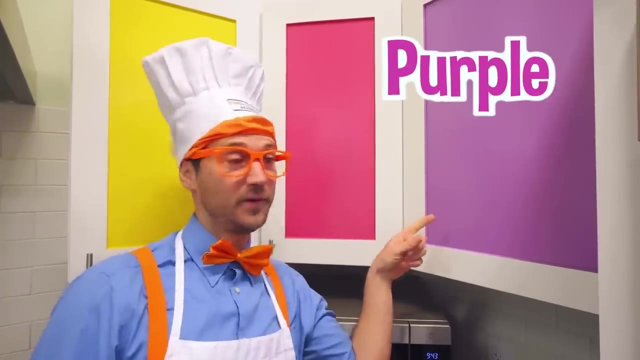 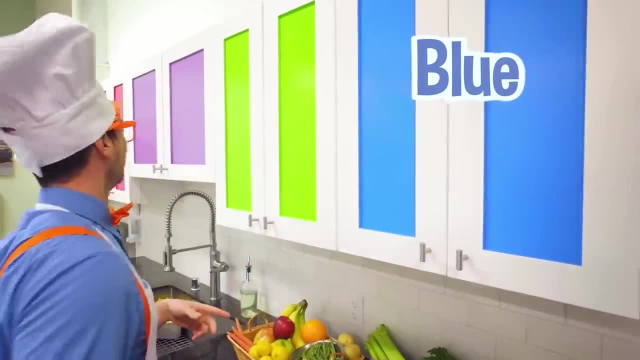 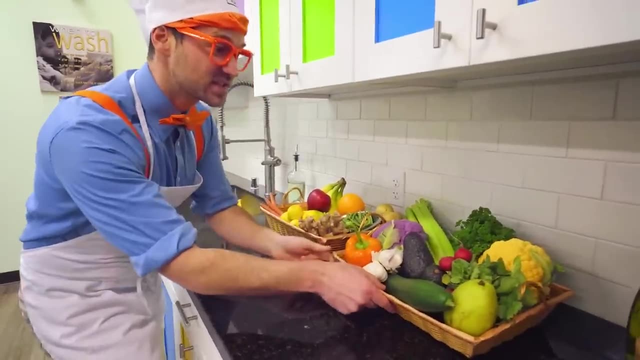 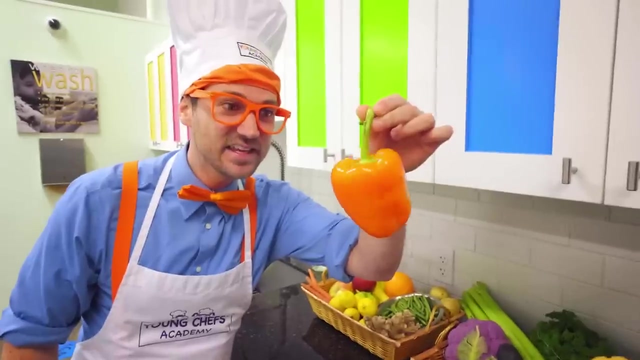 Whoa, I bet there's a lot of cool things in these cabinets. Whoa, Look at this, some yummy vegetables. Hey, you know what kind of vegetable this is? Yeah, this is an orange pepper. Look at these. Yeah, some green beans. 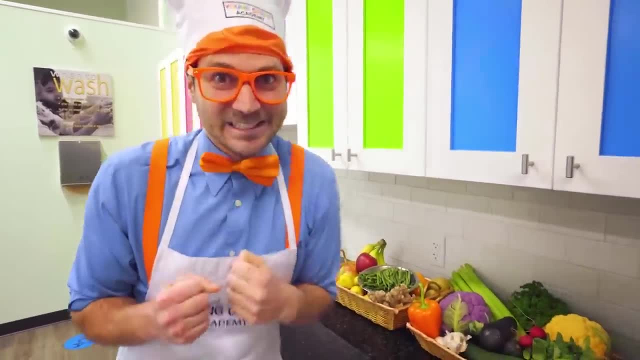 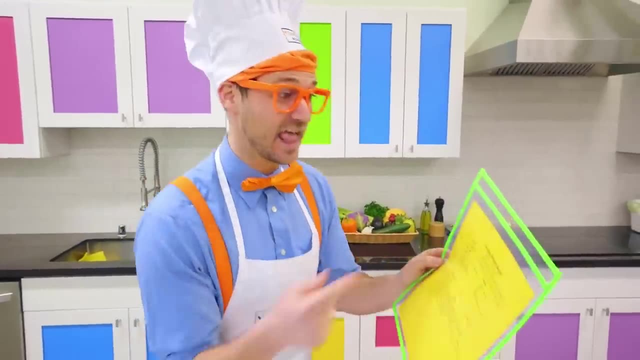 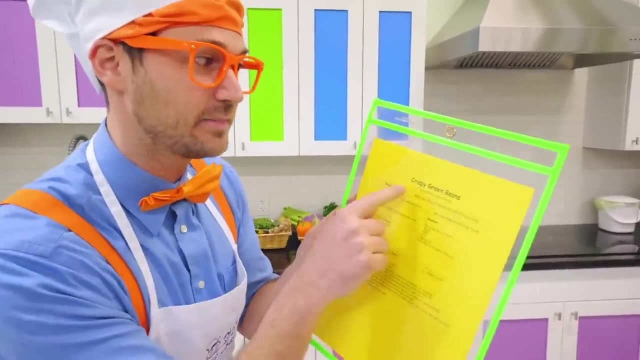 I sure do love vegetables. All right, I'm so excited. Whoa, I am so excited. This is gonna be tasty. I am looking at the recipe of what we're gonna be making today. Looks like we're gonna be making crispy green beans. 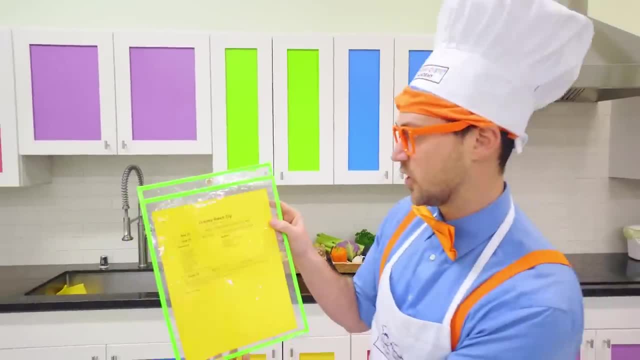 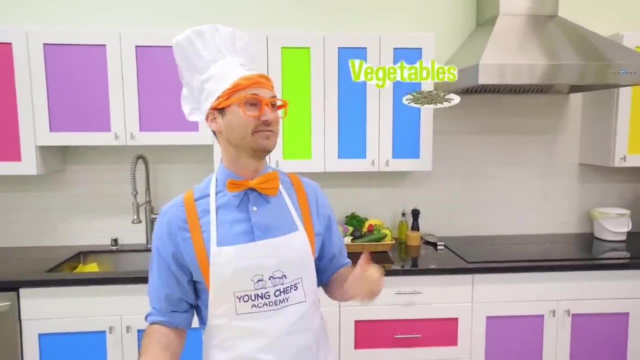 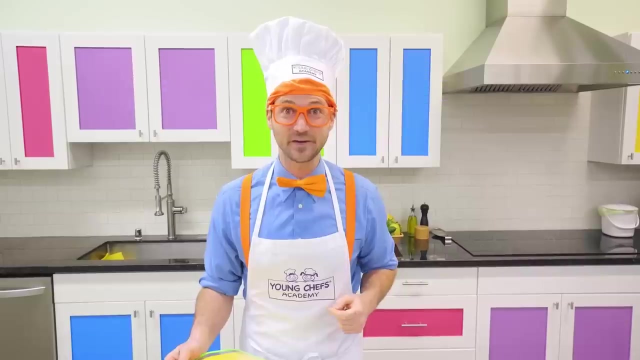 Whoa, those look tasty And creamy. ranch dip- Oh, this is gonna be so yummy and healthy. I love vegetables and I love ranch dip. I wonder if we're gonna be able to dip the green beans into the ranch dip. Yeah, 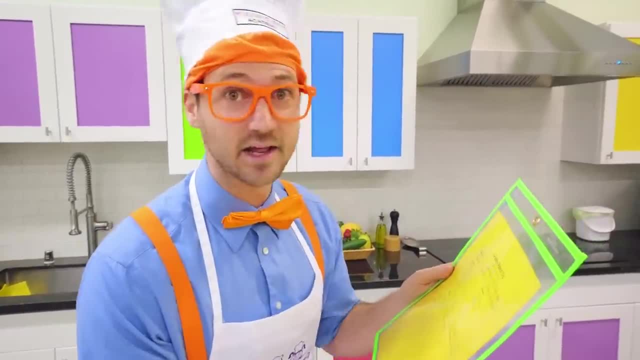 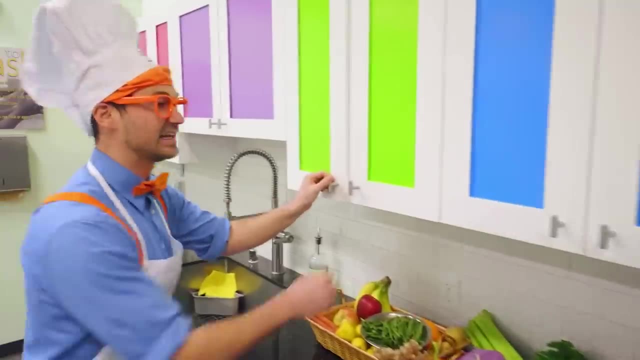 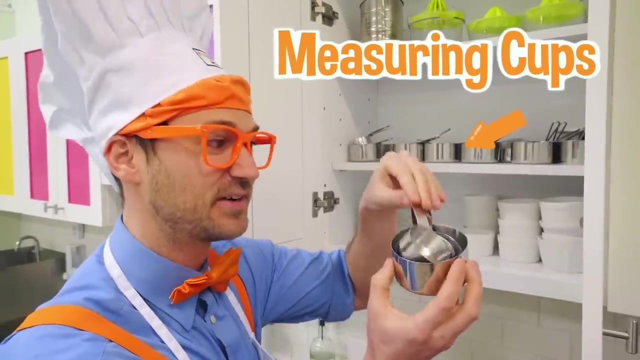 Okay, so it seems like we need a lot of tools and a lot of ingredients, So let's get to it. All right, let's see what's in here that we need. Okay, looks like we need some measuring cups. Oh, a small one. 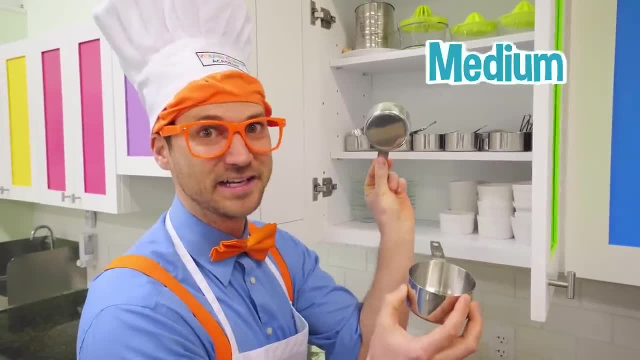 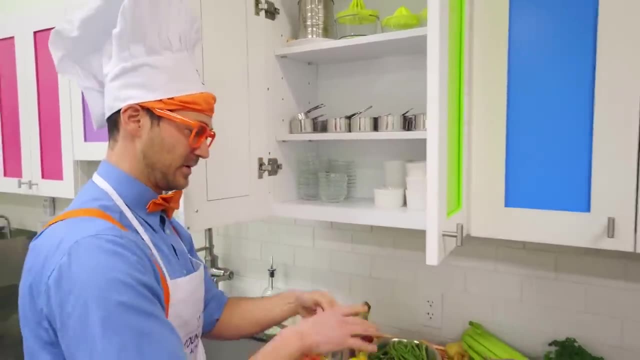 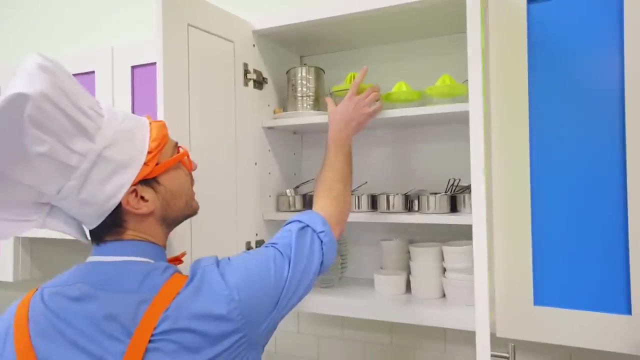 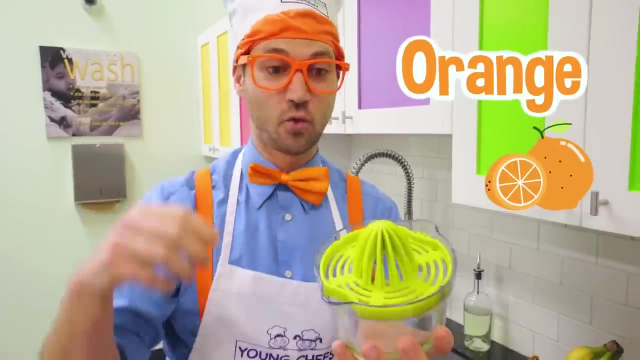 A medium-sized one, Another medium-sized one And a big one. Okay, Put those right back here. Perfect, Then we need whoa, a juicer. This is where you can put a lemon or an orange or a lime, squeeze it on top. 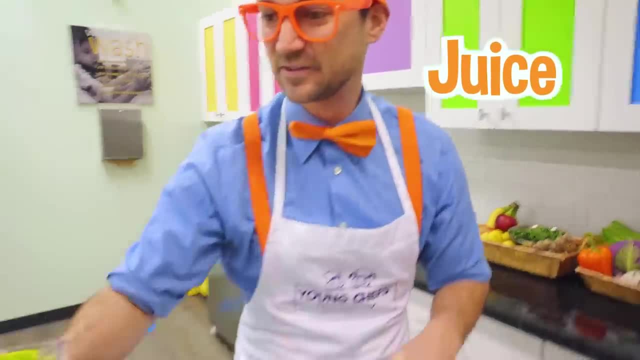 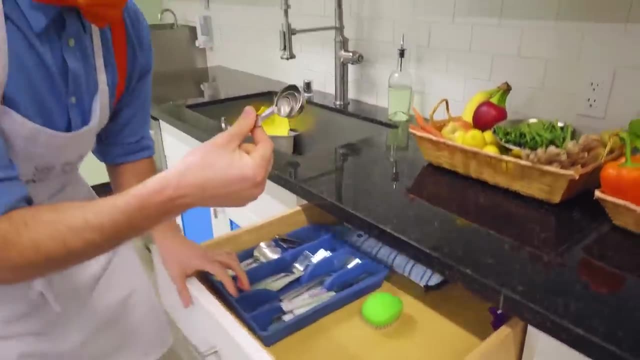 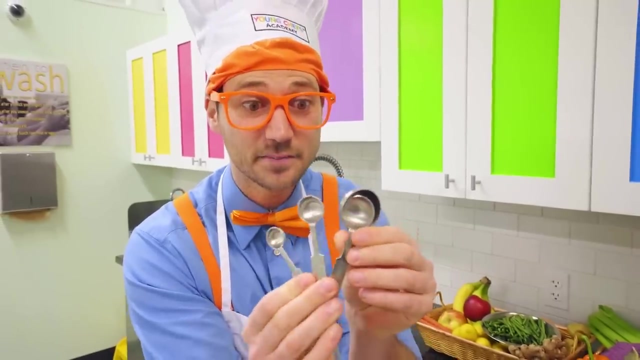 and then all the juice comes out the bottom. Okay, we'll set that down right there, All righty, let's see what's in here. Hmm, oh, we definitely need some measuring spoons. Whoa, Yeah, same thing, just like the measuring cups. 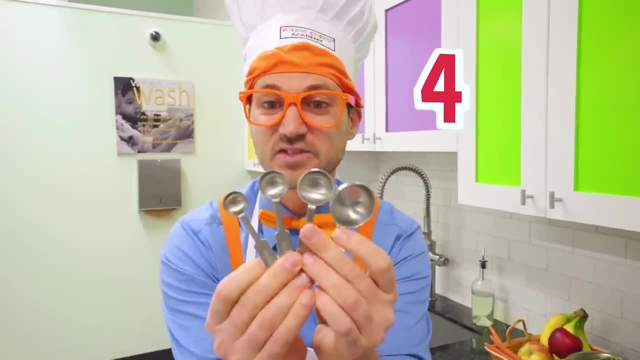 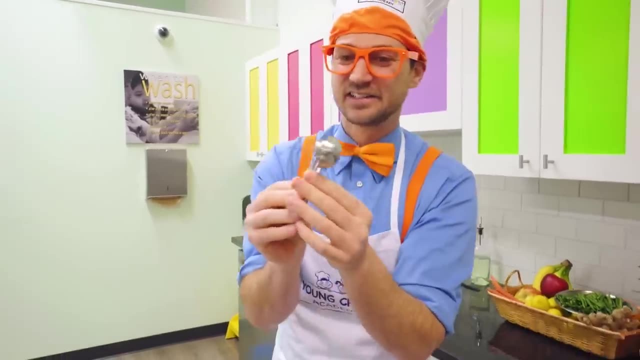 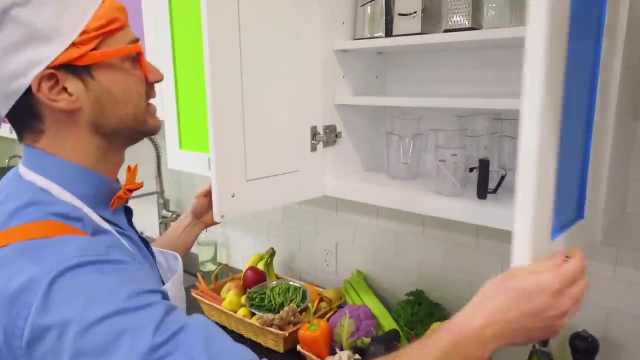 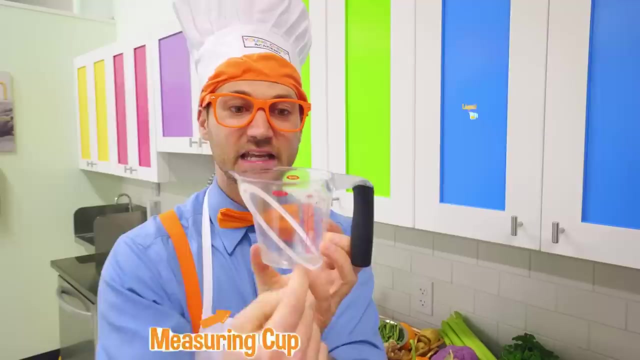 Measuring spoons of four different sizes, From small to medium to medium to large. Ha ha, Okay, put them right in there. Perfect, Okay, oh, let's see how about? oh wow, a measuring cup. This is what you put: liquids, and you could do solids. 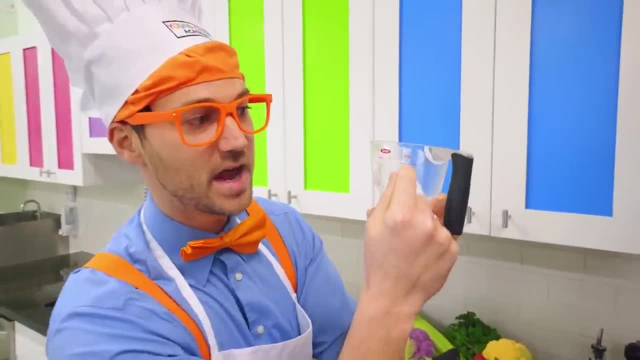 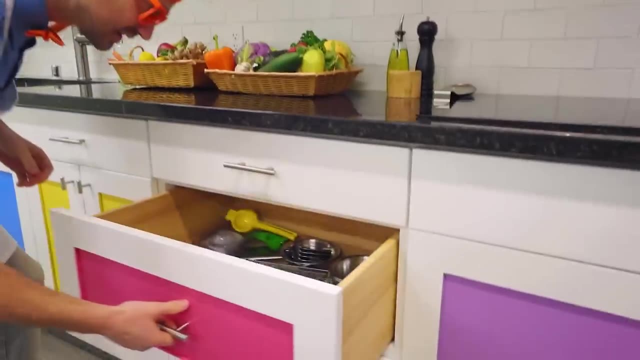 but this is primarily for liquids, And this is what you measure to see how much you have. Okay, put that down right there, Let's see. is there anything in here? Hmm, Hmm, There's a lot of cool things in here. 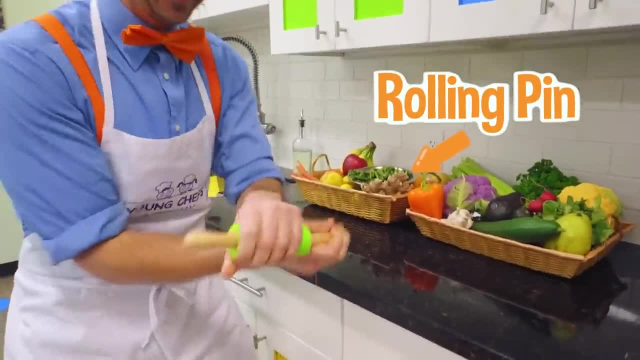 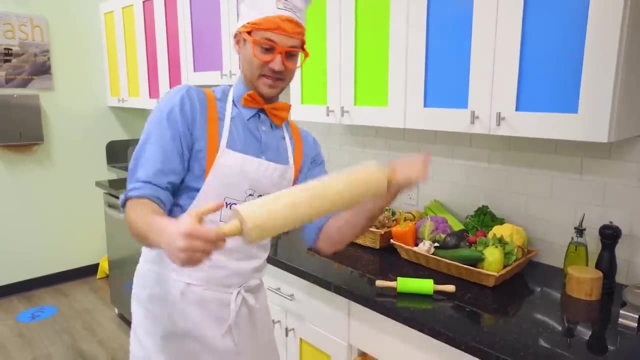 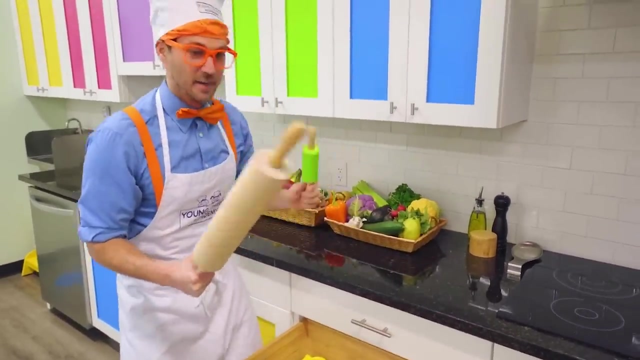 Whoa. look at this, It's a rolling pin. Oh, so cute. This is a small rolling pin- Whoa, Whoa. And this is a big rolling pin- Whoa. They're used to flatten things out. I don't think we need those today. 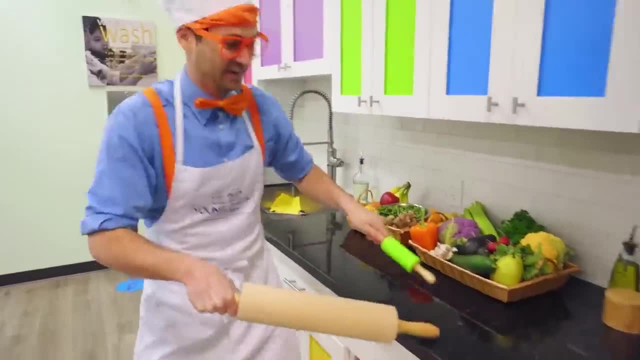 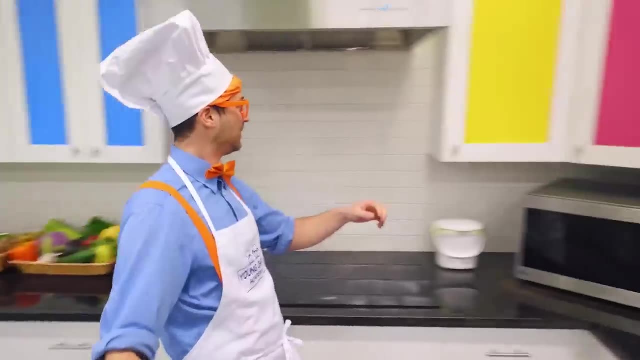 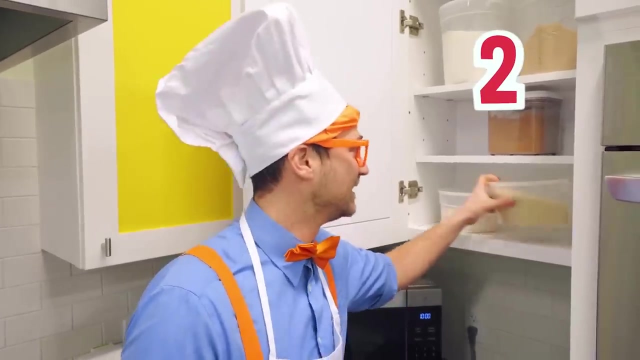 but they're pretty cool because you can use them for drums. Okay, enough playing, Let's get to cooking. All right, let's see probably right in here. Oh yeah, two ingredients that we need: breadcrumbs and flour. 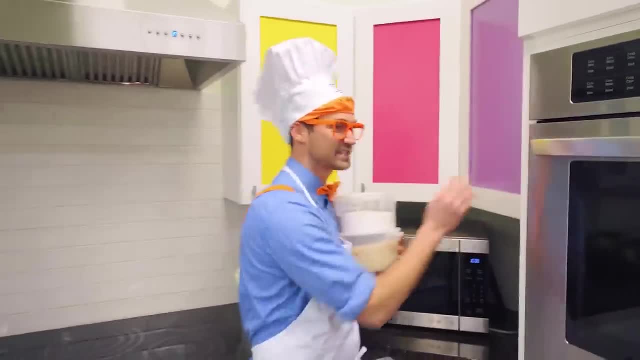 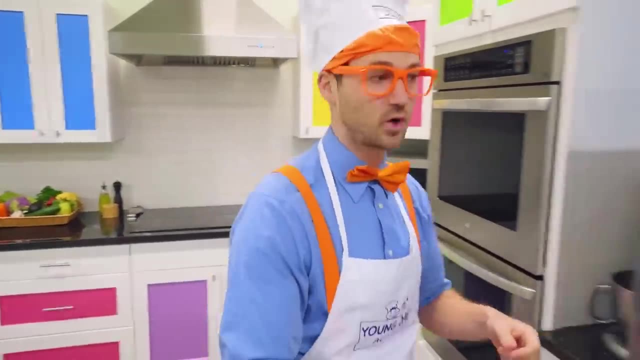 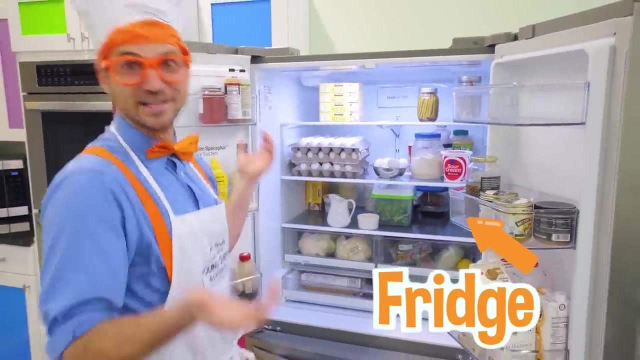 Perfect. Okay, we'll shut this. All right, there we go And let's see how. about some cold ingredients? Wow, Look at this fridge. Wow, It's so organized. Okay, looks like we have some cream, probably for the ranch dip. 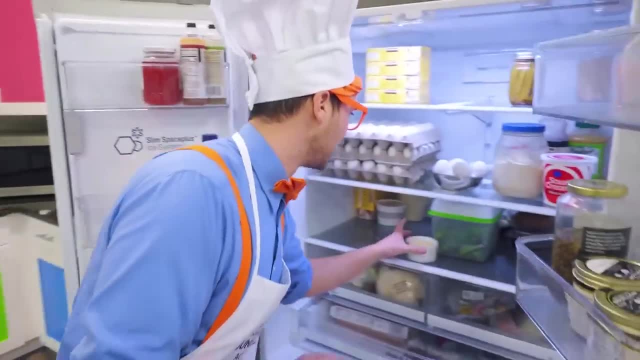 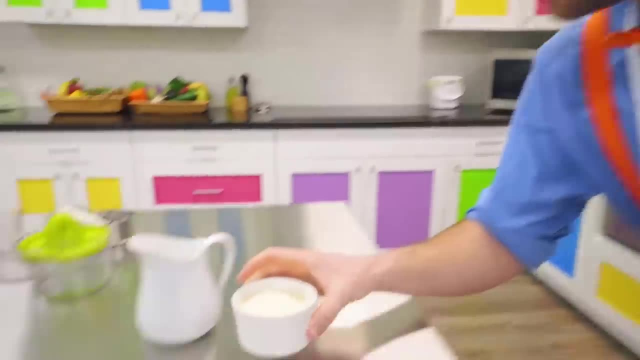 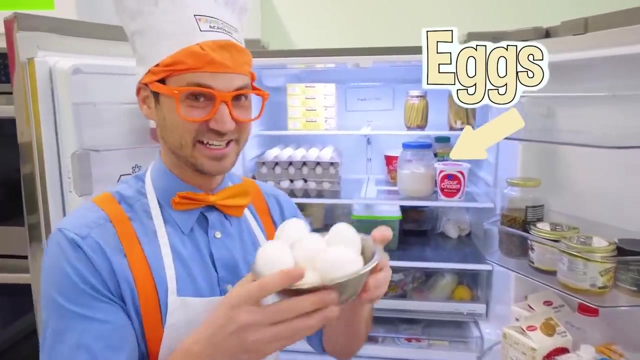 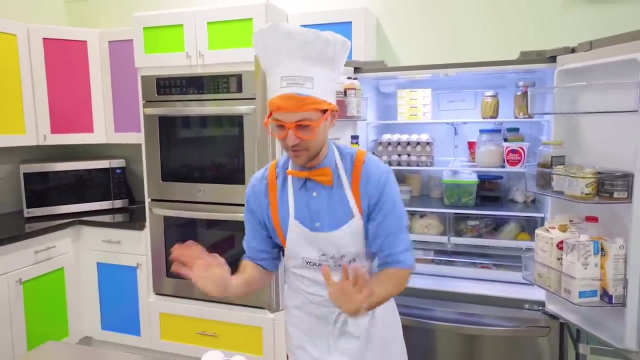 We'll set that down right there. Ooh, some cheese, Parmesan cheese. Okay, we'll put that down right there. And then we have some eggs. Yeah, check this out. Whoa, Whoa, Okay, We'll put those down right there for later. 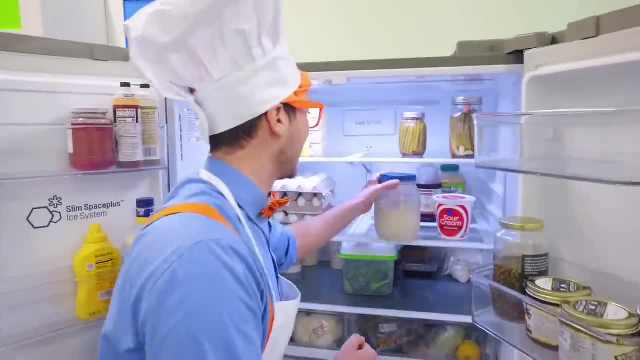 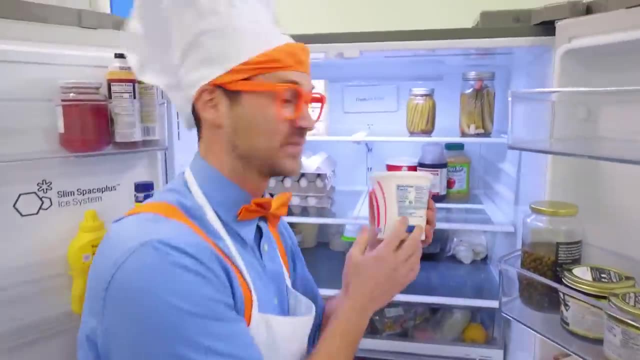 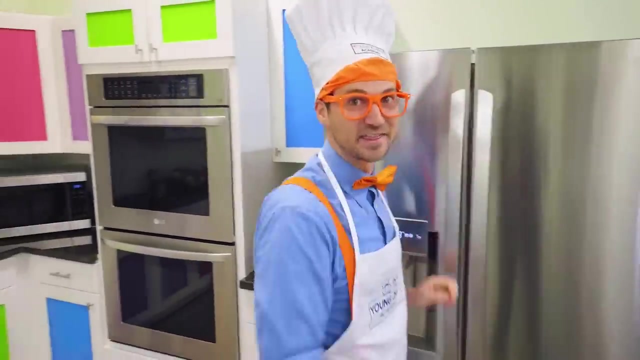 Probably shouldn't do that at home. And then we have some mayonnaise- Put that down right here. And some sour cream- Okay, Put that down. And now I think we're ready. Hmm, Looks like we have most of the ingredients and tools. 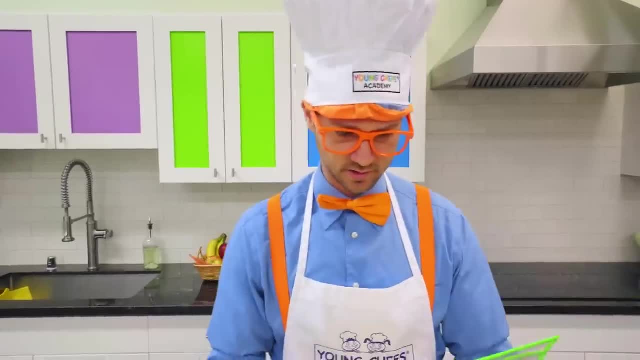 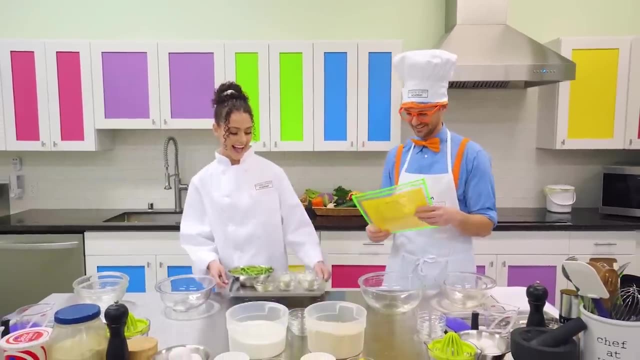 but this looks really hard. Oh no, If only I had some help. Want some help? Whoopi, Oh sure, Hey, Hi. I brought the rest of our ingredients that we need. Oh perfect, Okay, Well, here's the recipe. 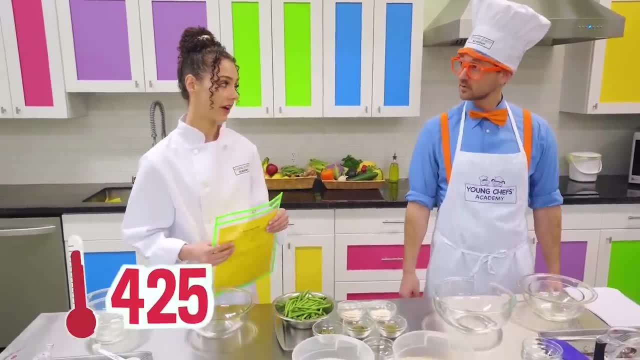 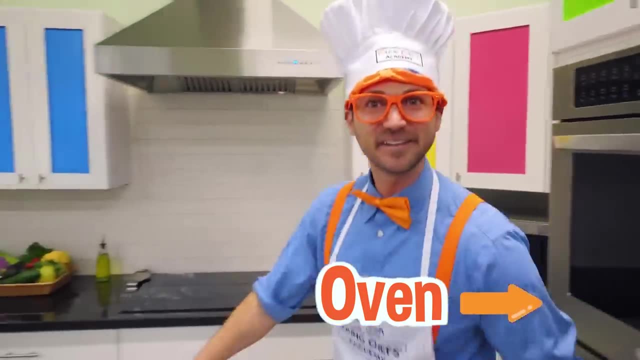 What do we do first? First, we're going to want to preheat the oven to 425.. Okay, I know how to do that. Okay, preheat the oven to 425.. Perfect, Good job, Whoopi. Thank you. 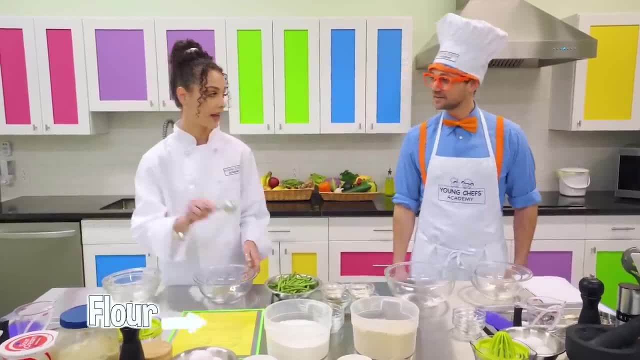 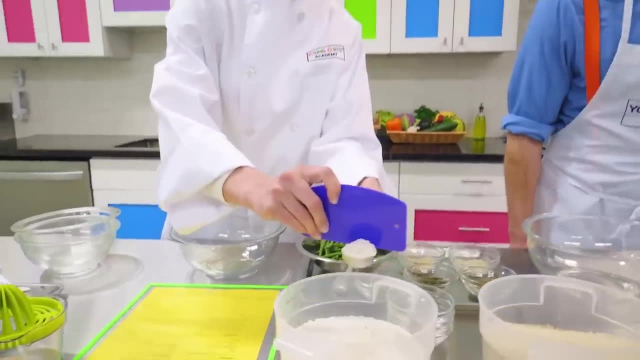 All right. First, we're going to want to do a tablespoon of flour into our bowl. Okay, We're going to want to make sure that we get a true tablespoon, because that is not accurate. So we want to scrape off the extra flour. 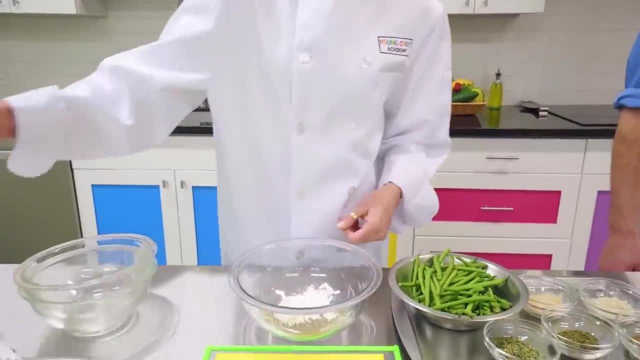 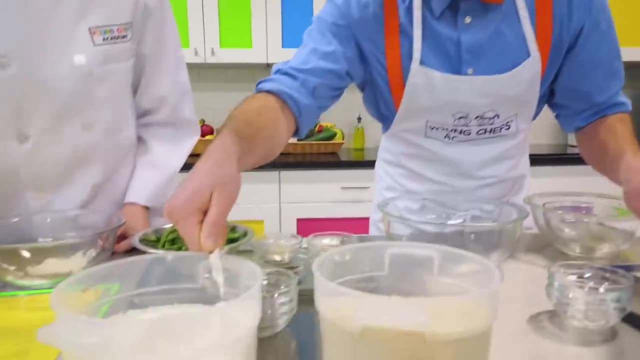 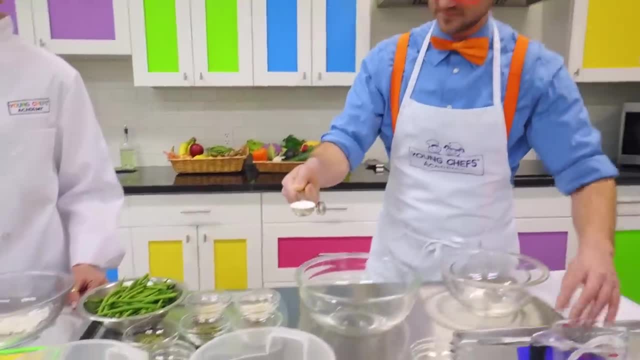 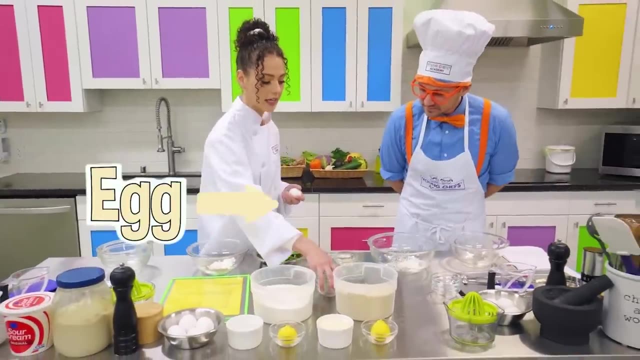 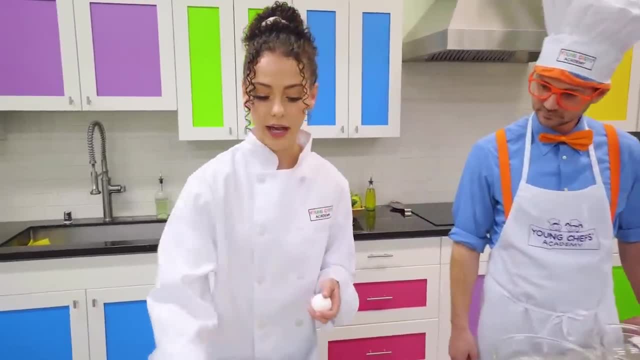 Okay, Let's see. So at Young Chefs Academy, we crack an egg using the table, not the edge of the counter, so that it doesn't get all over the floor in the mix. Okay, You want to crack hard and use your thumbs to break open the egg? 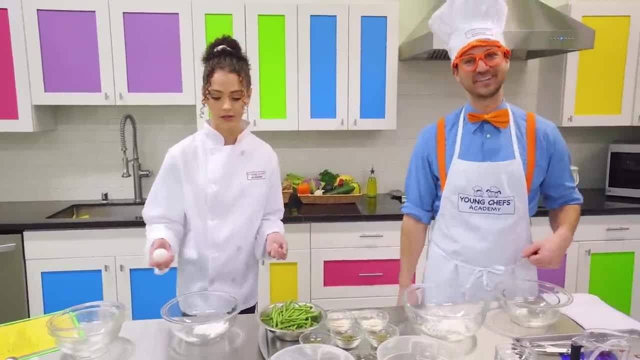 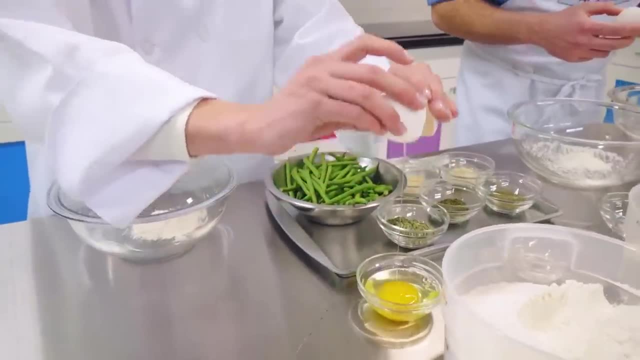 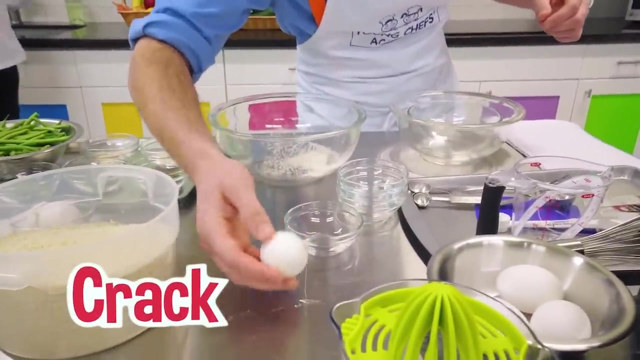 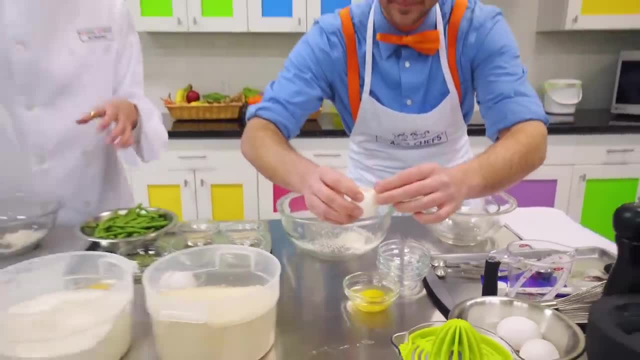 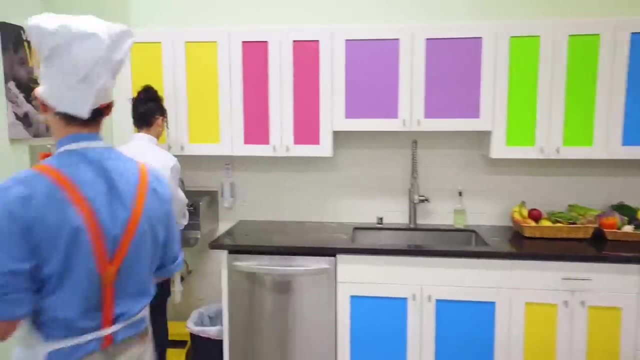 Perfect, Perfect, Perfect, Perfect, Perfect. There we go. Great job, Whoopi, Thank you. Next we're going to want to wash our hands because we touched a raw egg. Oh Wow, she's done it again. 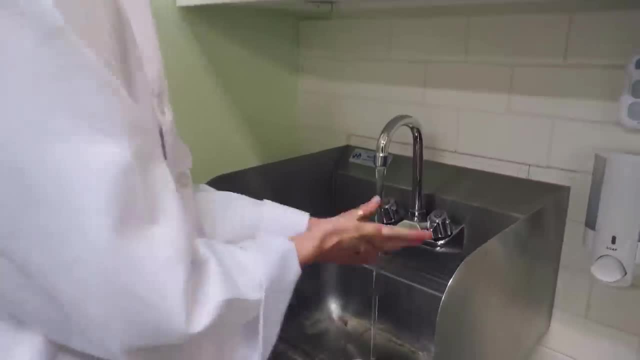 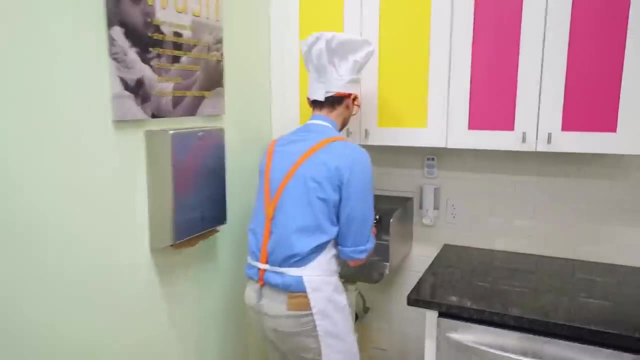 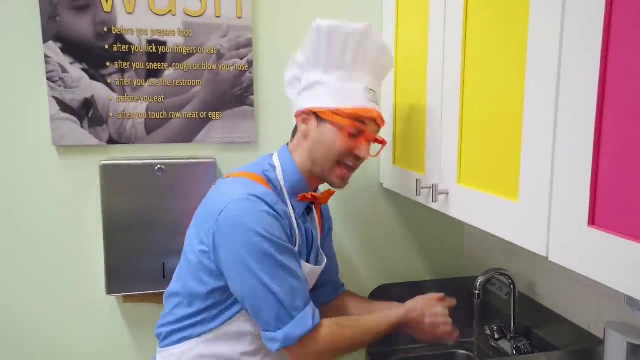 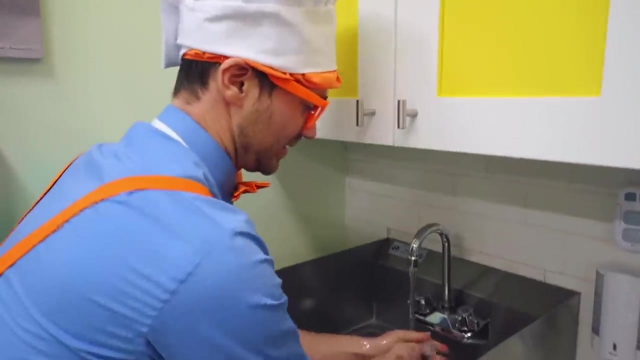 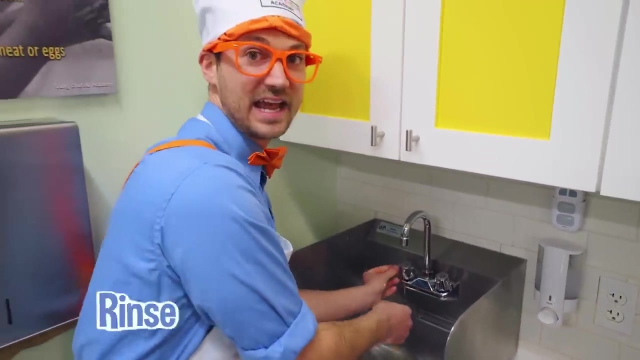 We really did nothing right. Let's put the ник on top. That's the devil. This is awesome, Cool, Thank you All. right, there we go. Let's rinse them off. It's really important to rinse off your hands and wash them completely after touching raw. 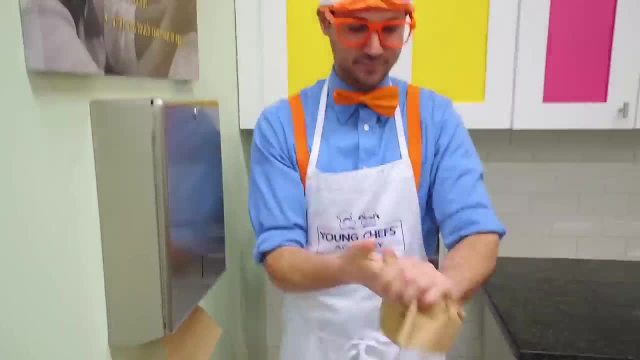 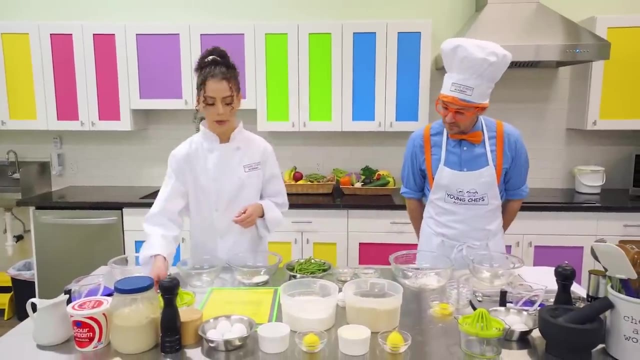 eggs or meat or anything like that. Now we're ready. Okay, All right. Next we're going to want to do a cup of panko. Okay, Use our like there. Wow, That looks about right. Yeah, Is panko just like breadcrumbs. 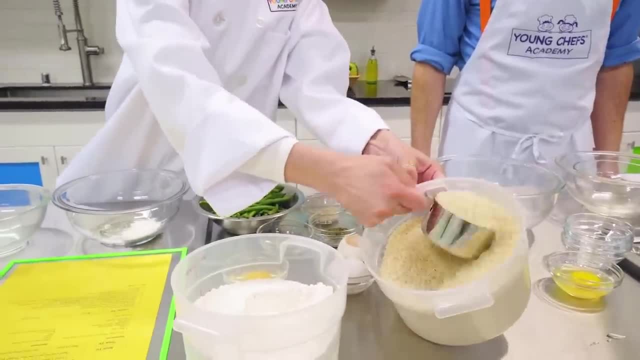 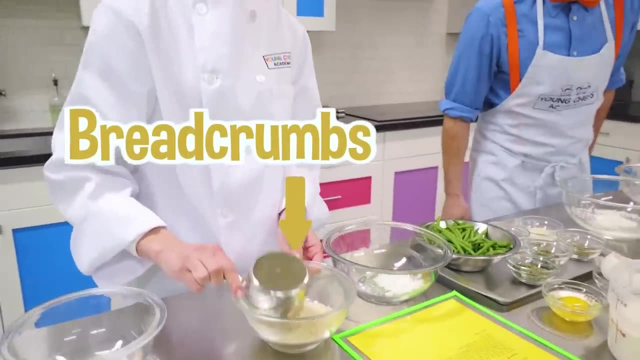 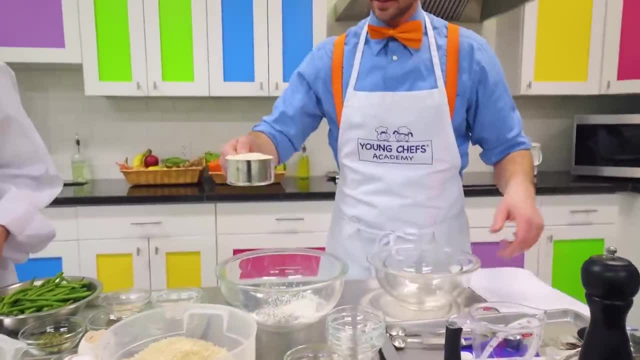 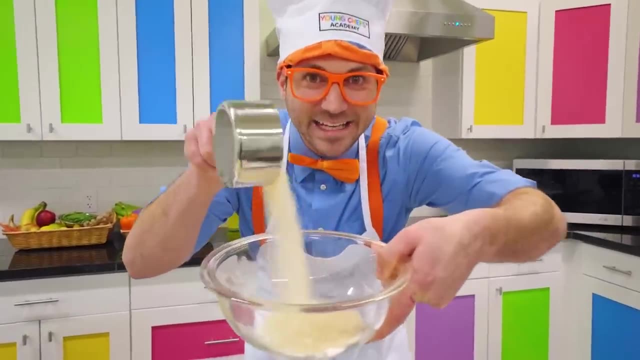 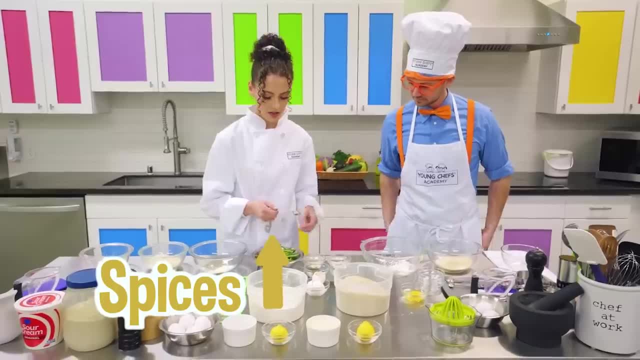 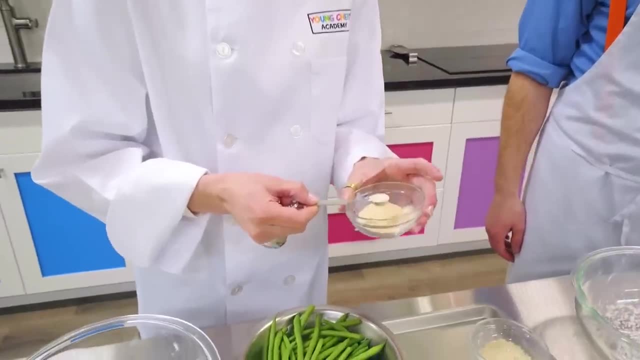 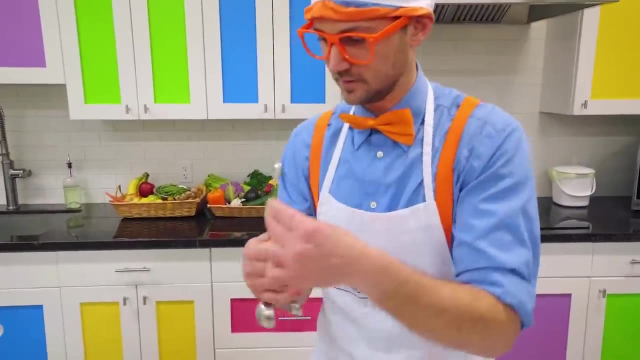 Next, we're going to want to add the rest of our spices, which is garlic salt and salt. Okay, So we're going to want to use a fourth of a teaspoon of garlic salt in our panko. Okay, There we go, This one. 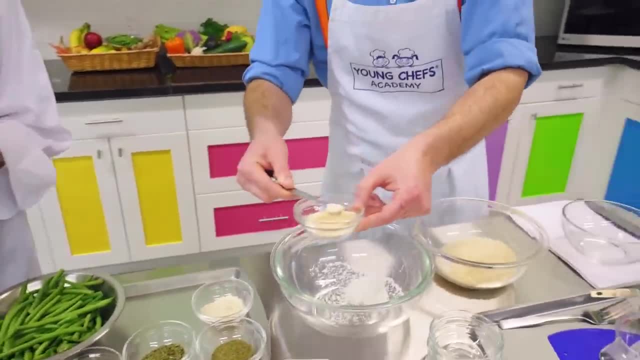 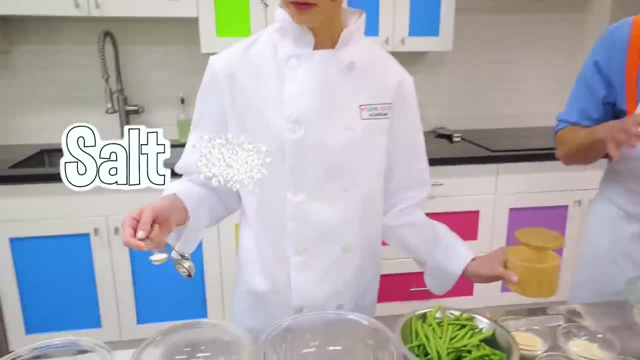 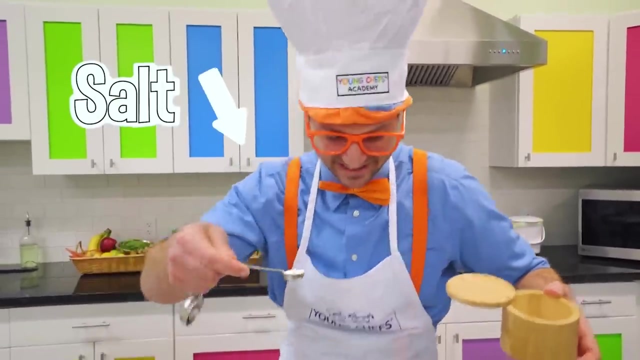 Mm-hmm. Okay, Then put it in the panko. Perfect, And then half of a teaspoon of salt. Thank you, Wow, salt is so yummy, Here we go. Can you use your whisk and whisk that up, Yeah? 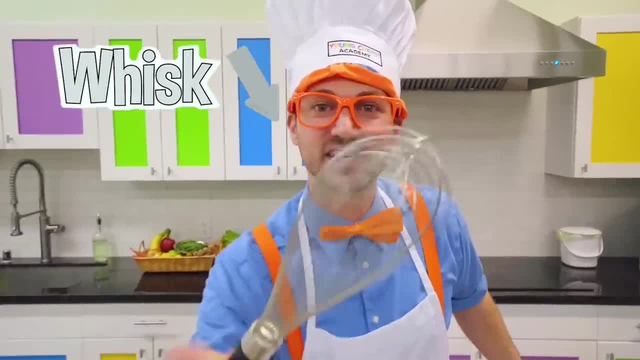 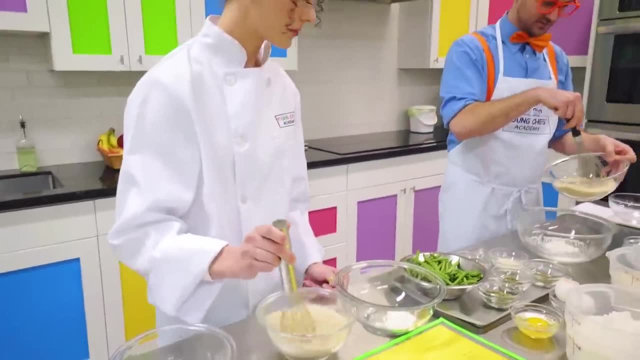 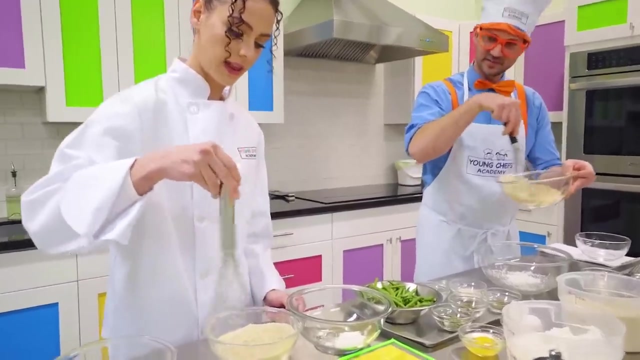 Check it out. This is a whisk. Yeah, How do you do it? And you want to whisk with your wrist? Okay, Whoa, This is a really good way to mix it all up. Good job, Yeah, You want to use it like that. 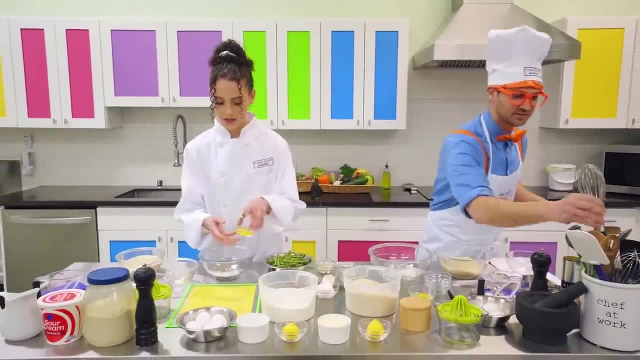 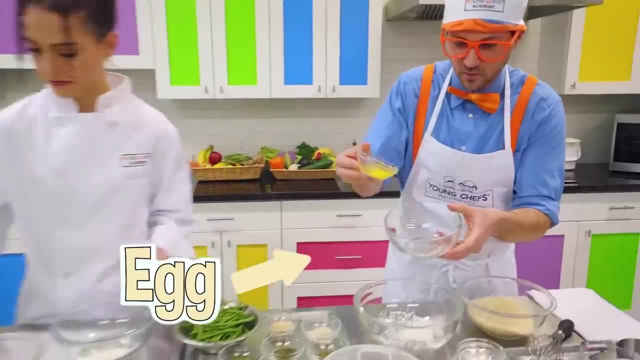 All right. Next, we're going to want to put our egg into this mixing bowl, the clean mixing bowl that we have. Okay, Here we go, Put the egg in this bowl. Wee, Oh, All right. And we're going to want to use a little bit of water. 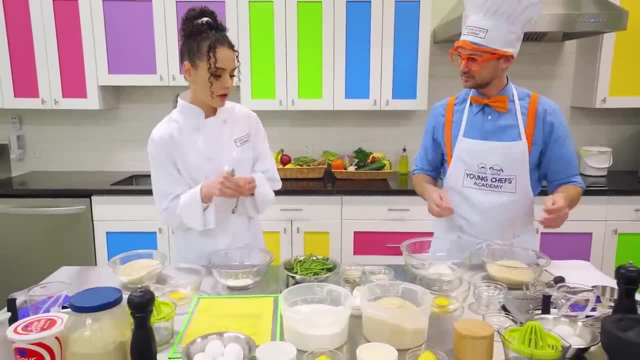 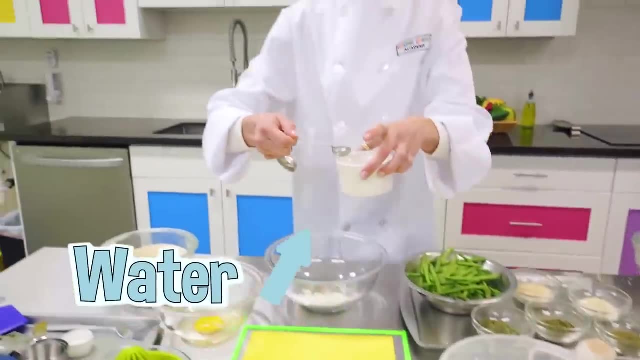 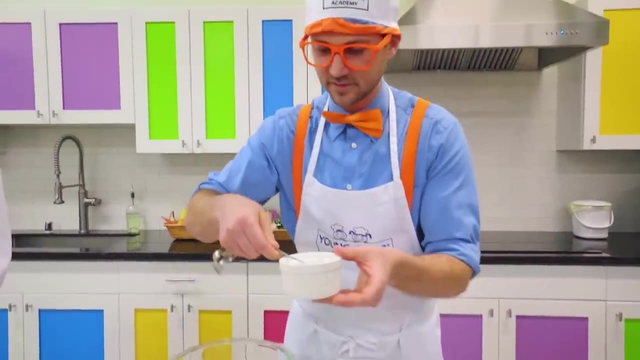 A little bit of water like this In with the egg Perfect. Thank you All. right, Put some water in with the egg Perfect. Can you whisk that egg up with the fork for me With the fork? Okay, Fork. 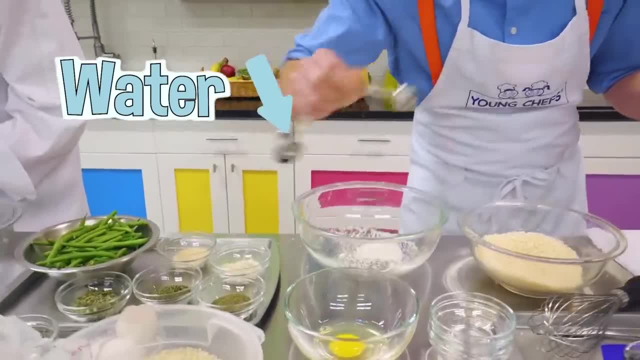 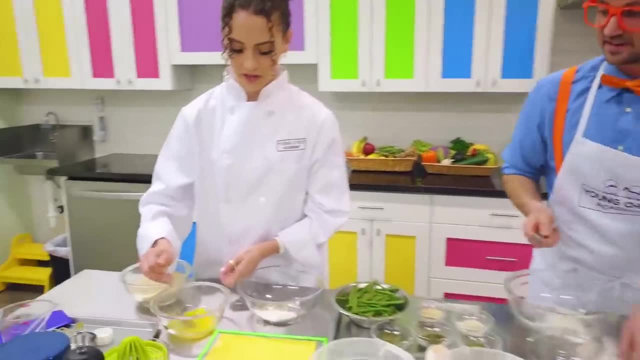 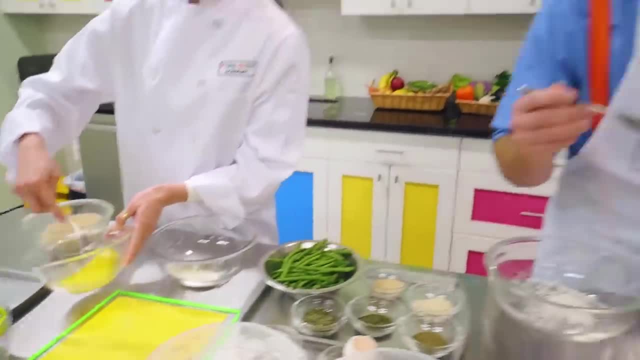 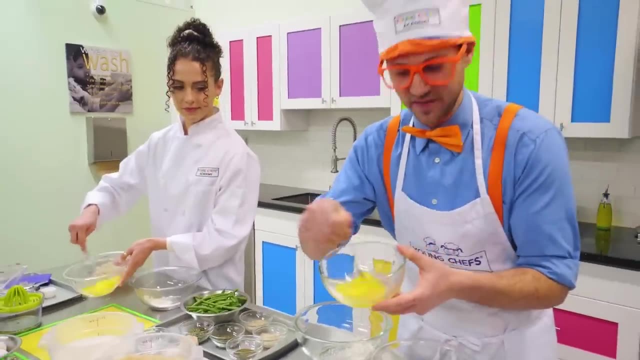 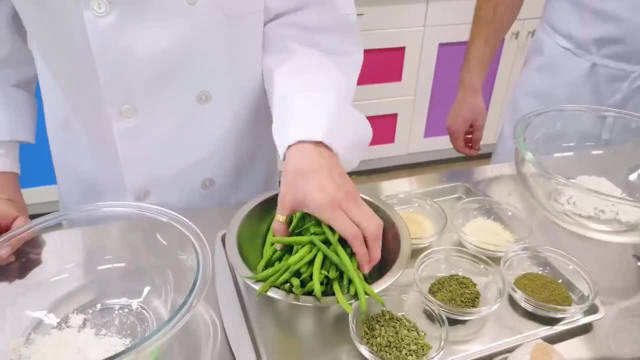 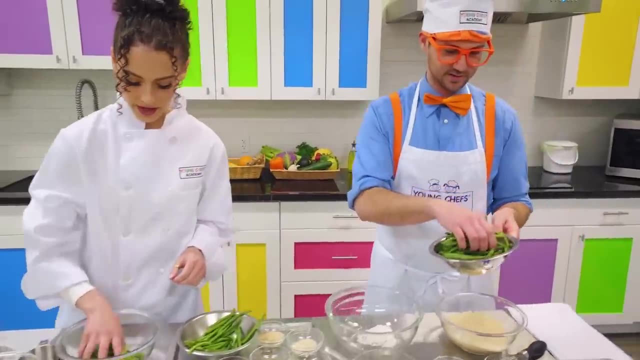 Oh, Okay, So you want to whisk it just like that? Okay, So let's take the fork and let's whisk the egg- Whoa, Did you see how the yolk broke up- and toss it in our flour. all right, make sure you get them all nice and mixed up and coated in flour. 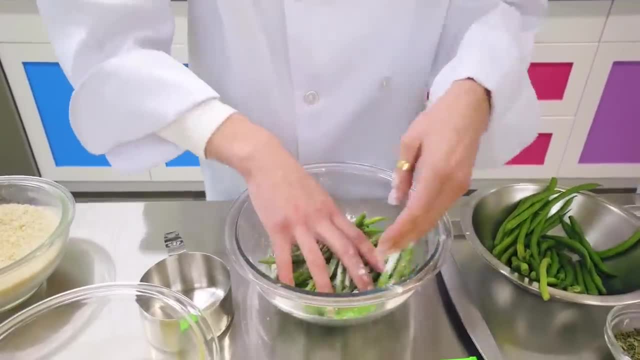 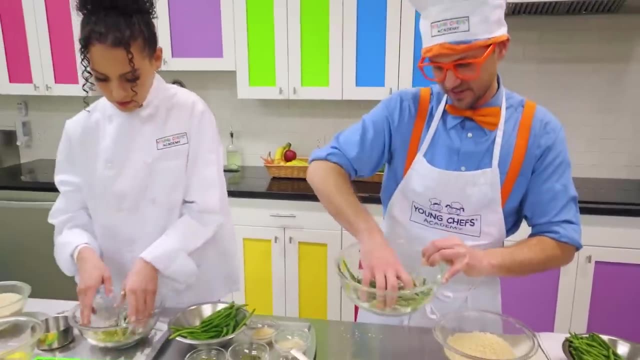 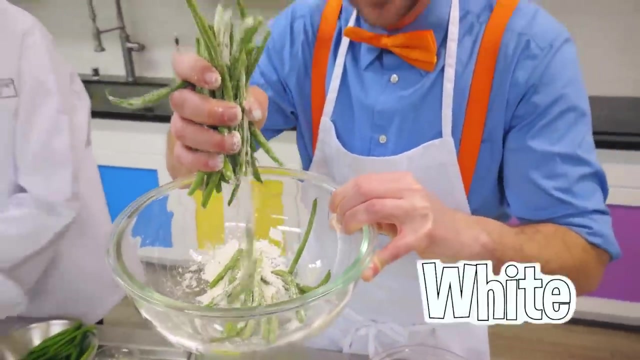 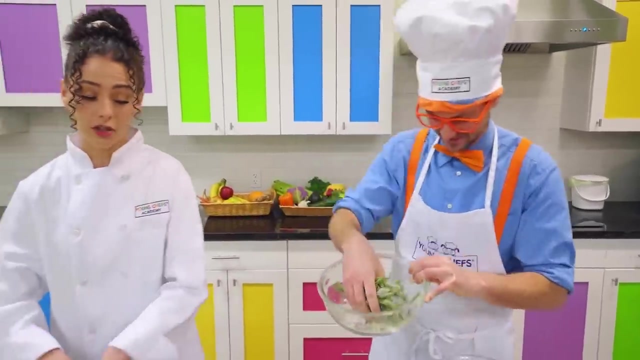 okay, toss it. wow, this is gonna help the egg stick to the green bean. okay, interesting. look, they used to be green, but now they're green and white. hey, remember how we washed our hands? yeah, good thing we did, because i'm touching food with my hands. you don't want to. 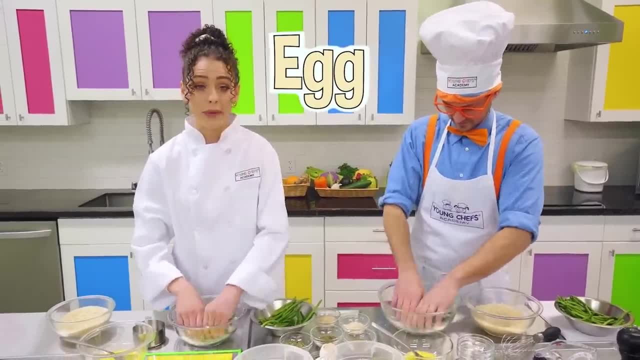 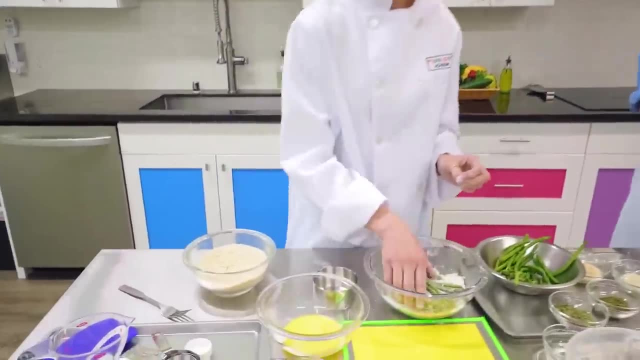 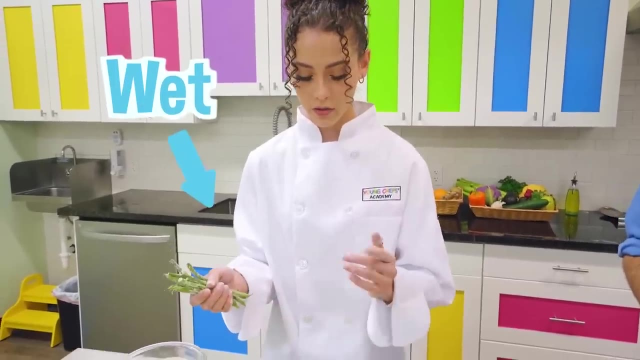 touch anything. after you touch egg or raw meat, you want to make sure you wash your hands? okay, all right, now we are going to touch the egg, we're going to put the green beans, we're going to use two different hands. we're going to have our dry hand and our wet hand, so we're not going to touch. 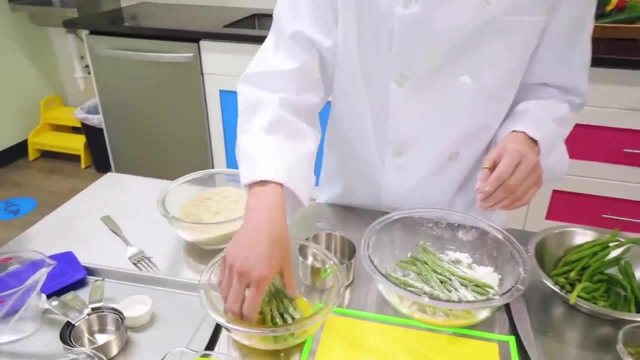 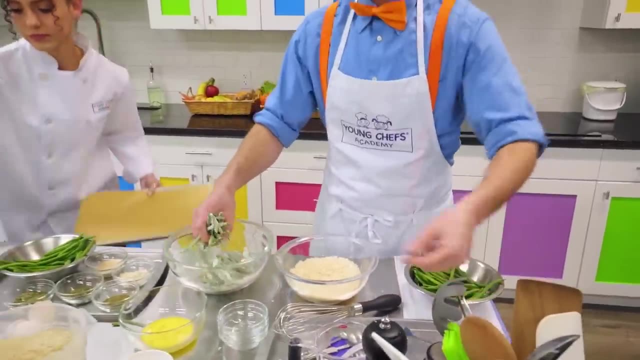 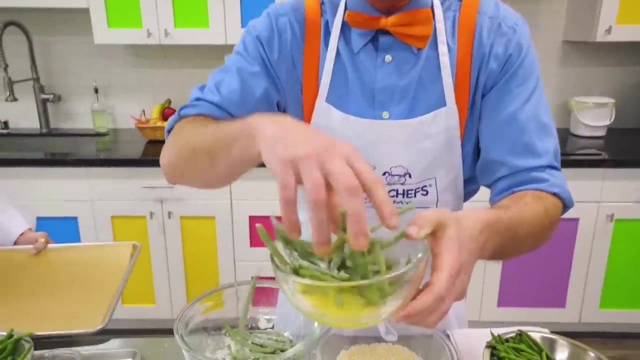 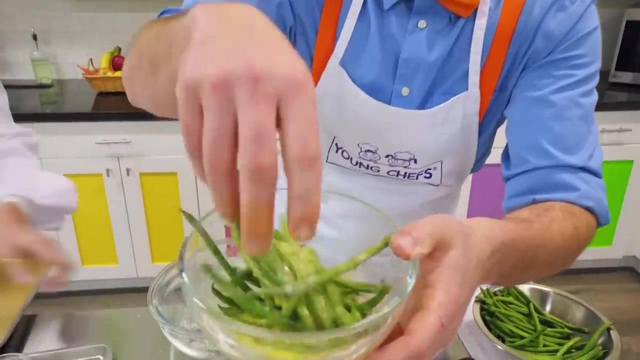 the egg with this hand. we're going to put our green beans in here and toss it around. okay, take the fork out now, toss it. here we go. oh, i'm spilling, that's okay, okay. wow, look at it. there's so much egg on these green beans, okay. 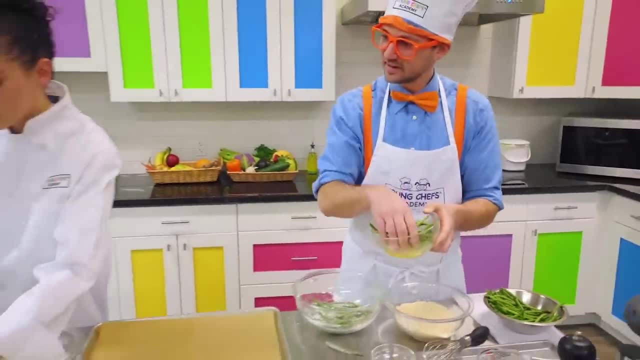 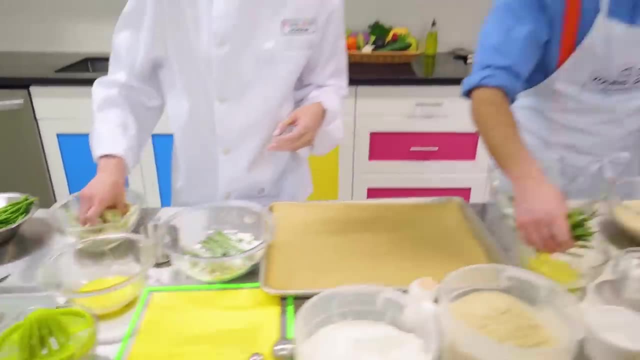 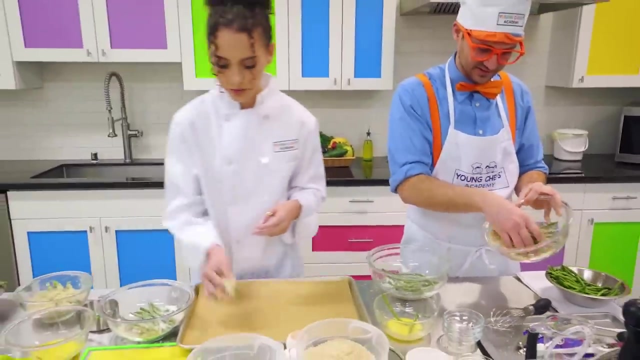 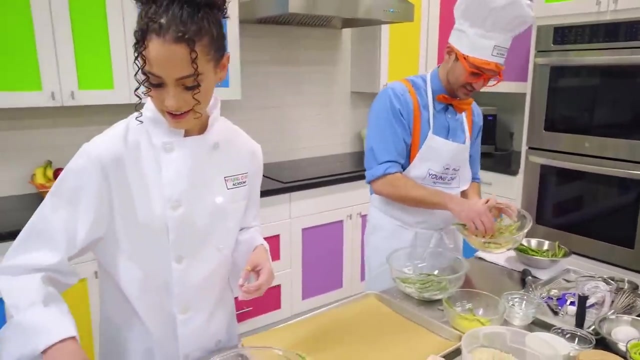 all. right. now you're going to want to put the green beans into the batter panko, toss them around real quick. Okay, Wow, That looks fun. And once they're nice and evenly coated in panko, you want to put them on to the tray. Okay, whoa, These are going to be so yummy. I know I'm excited. 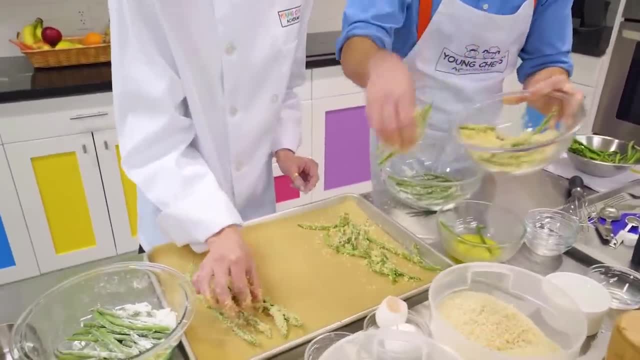 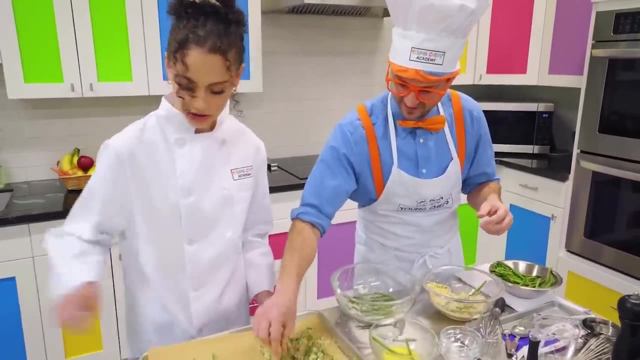 Let's put them a little bit nicer so that they're not so messy. Okay, That way they'll cook really evenly when they're spread out on the tray. There you go. That makes sense. Oh, I see, Because if they're on top of each other then the heat can't touch the whole. 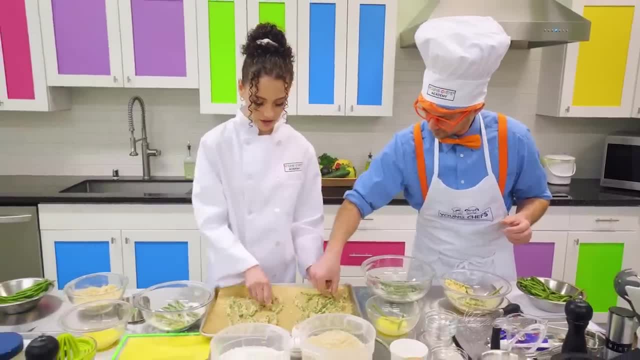 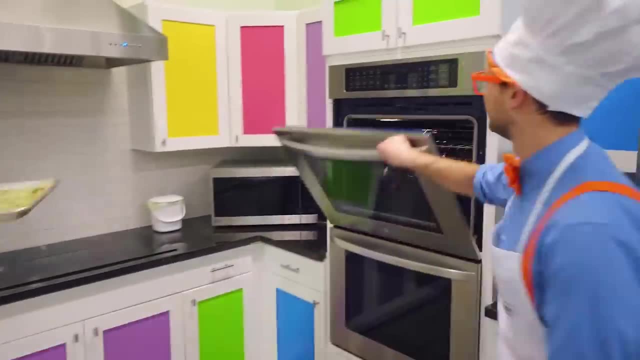 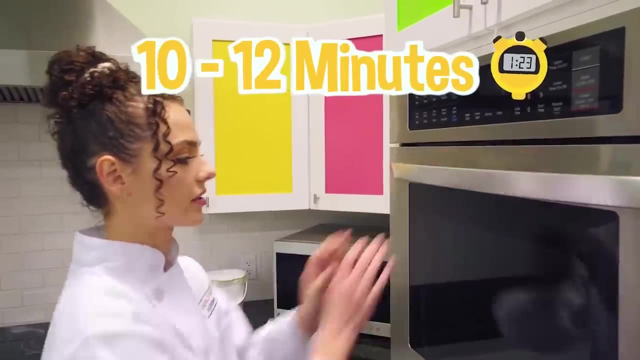 green bean. huh, Exactly, You want to make sure that the whole thing is getting cooked. We're ready for the oven. Okay, Here we go. Here you go. Thank you. All right, Let's put them on the tray. Perfect, Those will take about 10 to 12 minutes to cook. Whoa that. 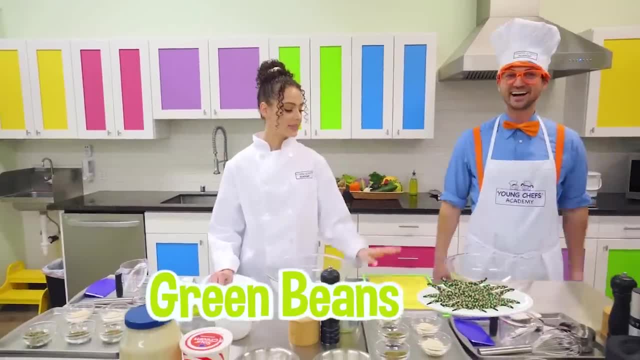 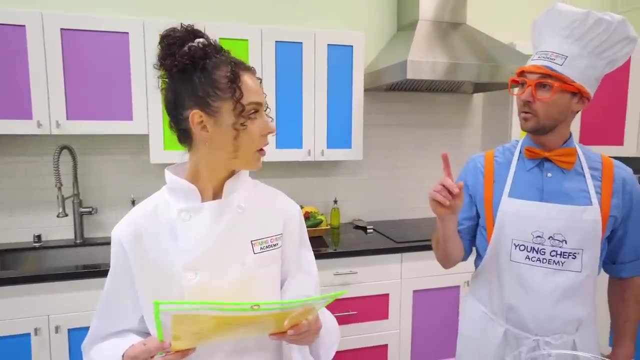 was really fun making those green beans with you, Wasn't it? Yeah, Let's make some ranch to different ones. What ingredients do we need? We need mayonnaise, sour cream, buttermilk- Oh wait, Did you say buttermilk? Yeah, Oh, I said cream earlier. Okay, So we need buttermilk. 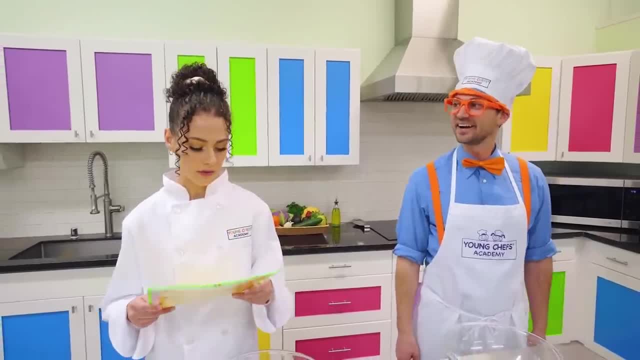 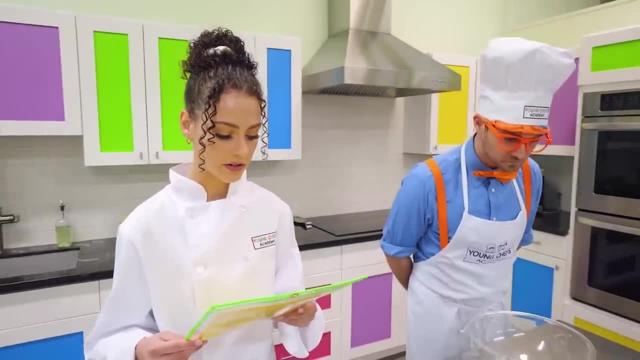 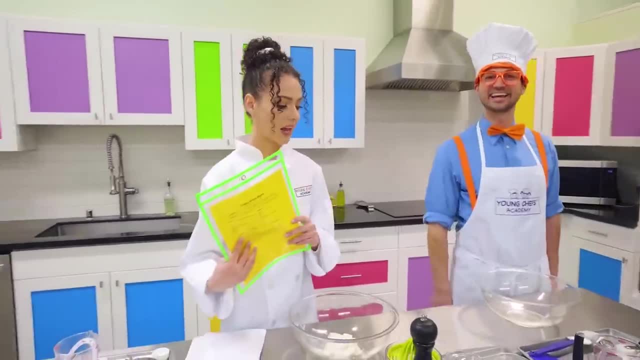 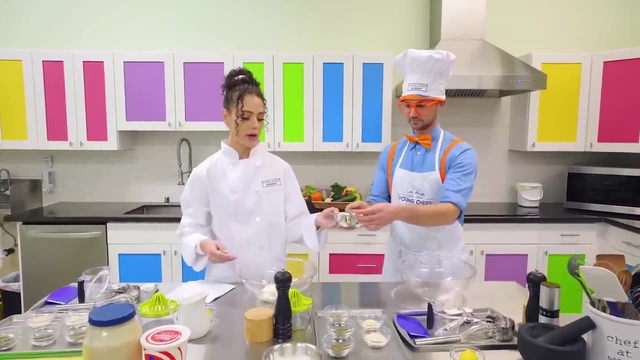 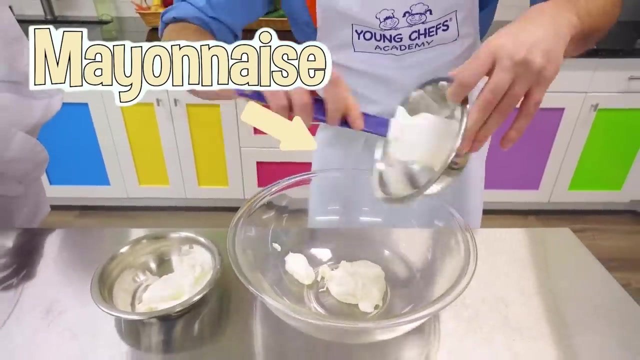 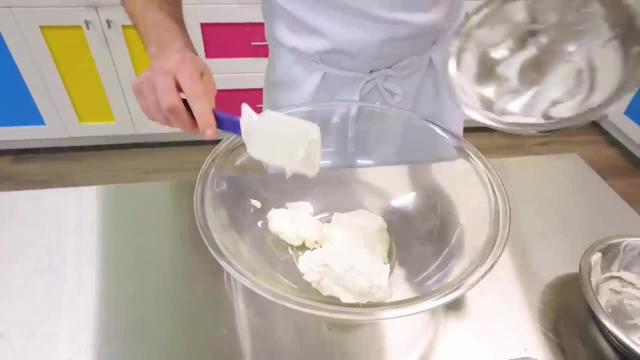 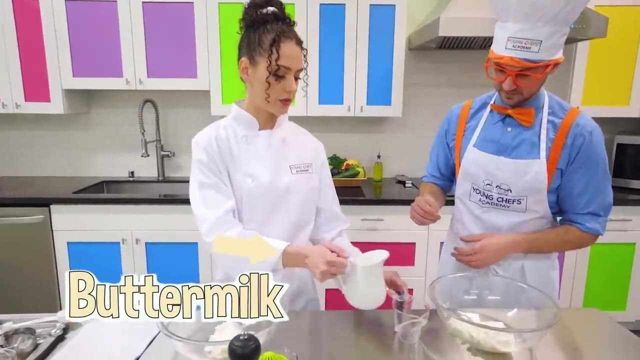 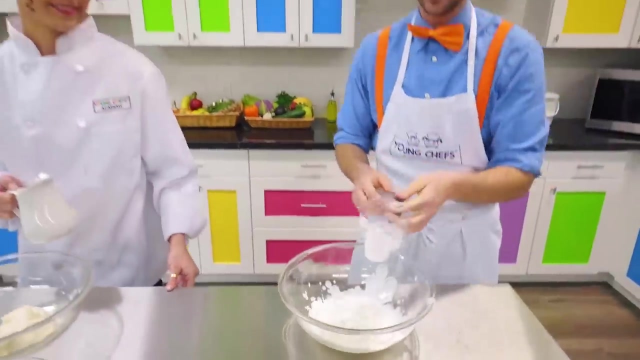 All right, All right. Whoa, Whoa, Alright, there we go. Awesome. Now we're going to want to do half a cup of buttermilk into your bowl. Alrighty, There we go. Perfect, Alright, now we're going to want to get our one-fourth teaspoon. 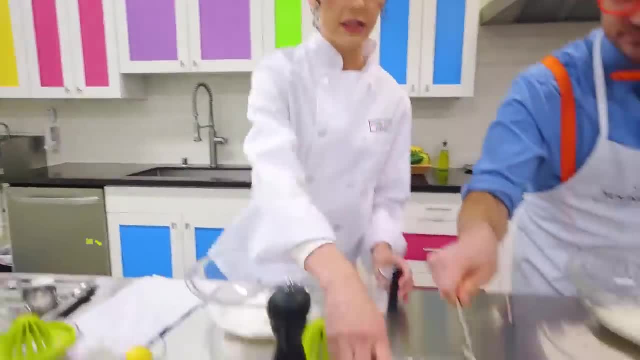 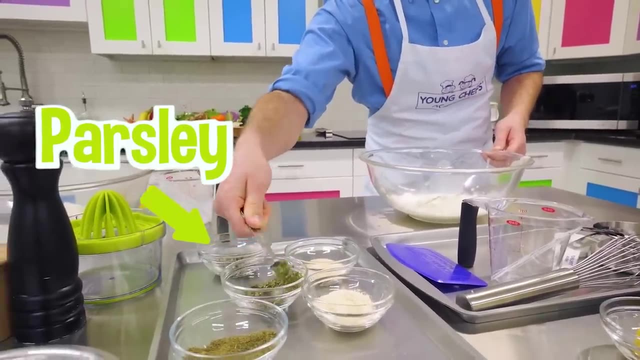 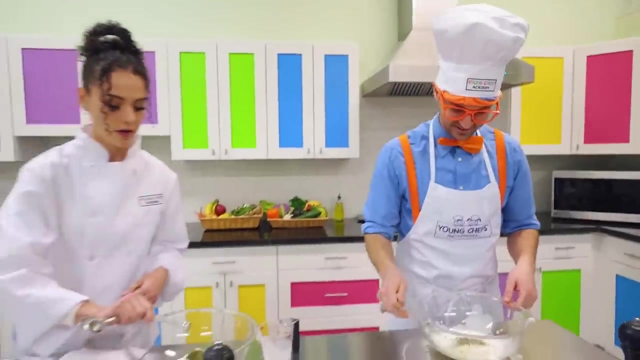 Perfect, I'm ready And we're going to use that for our dill right here: Parsley And our chives. Okay Dill, parsley and chives. There we go. Good job, puppy. Next we're going to want our half teaspoon. 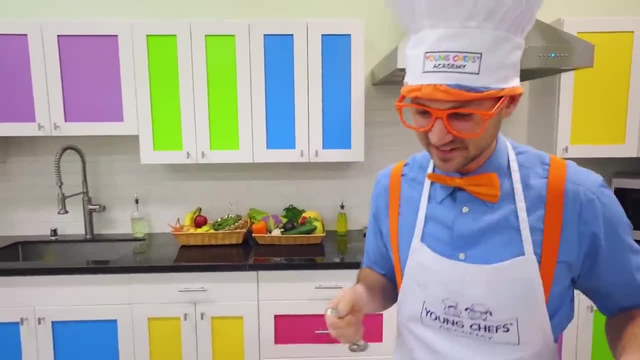 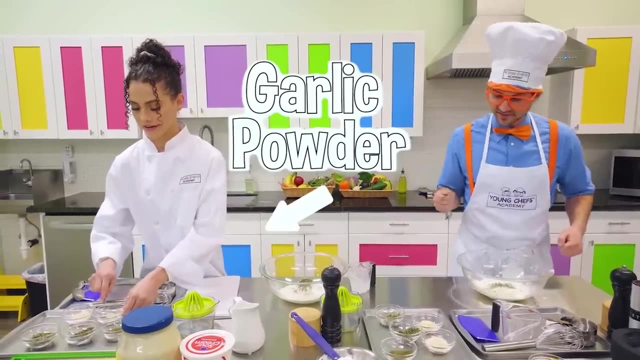 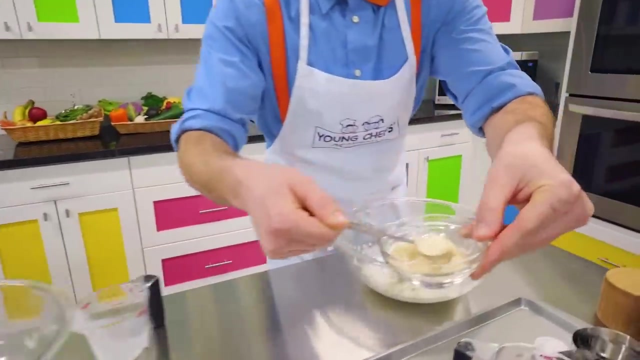 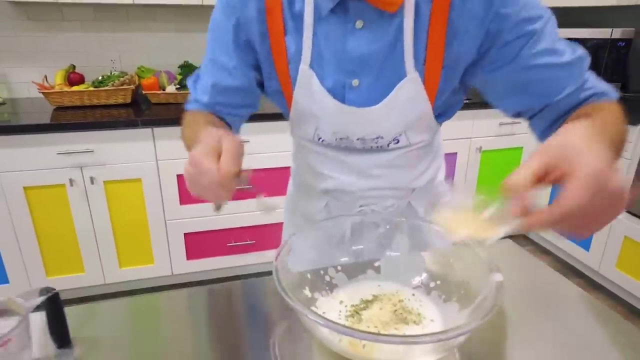 Okay, A little bigger, Alright. Alright, and we use that for our garlic powder and our onion powder. Alright, Let's give it a little scoop. And then this one: Perfect, This is going to be so yummy, Alright. 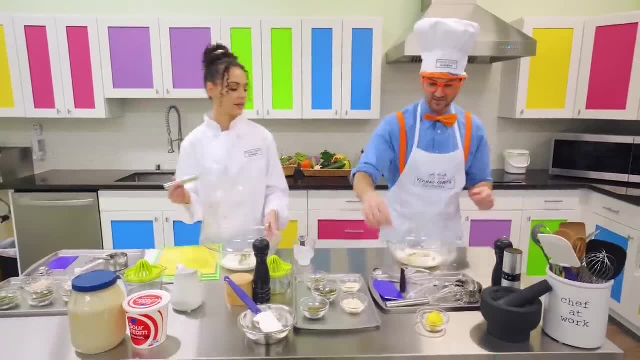 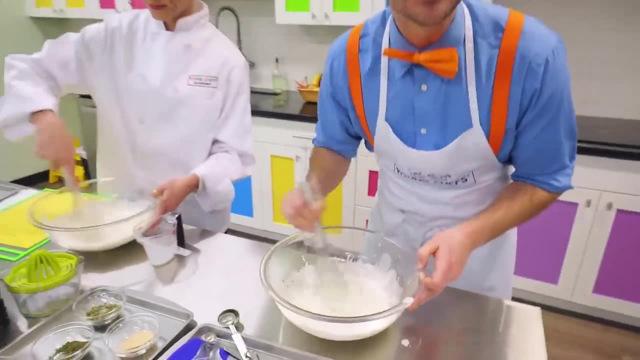 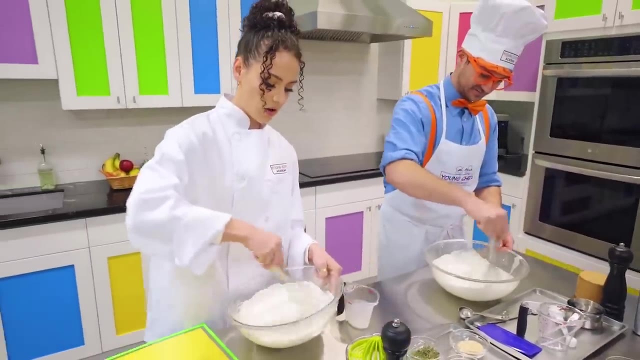 Perfect, Let's mix that up with our whisk. Don't forget, we whisk with our whisk. Alright, This smells so good. Once it's all mixed up, we're going to cover it. We're going to cover it and place it in the fridge to cool. 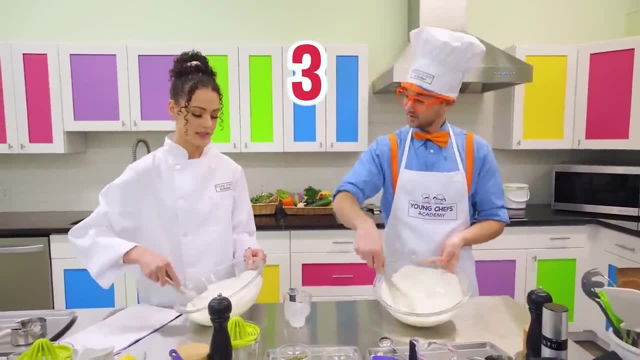 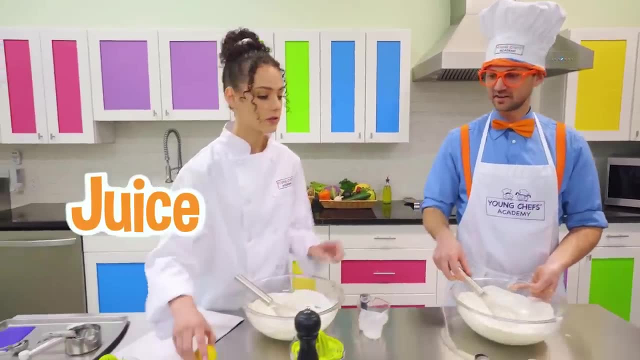 Alright, we only have three more ingredients. Okay, What are they? Lemon juice, salt and pepper. Okay, First, we want to juice our lemon. So you have a lemon right up there. Perfect, We have it cut in half and we'll use our juicer here. 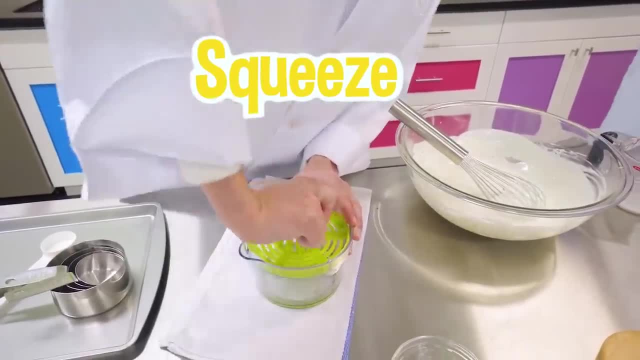 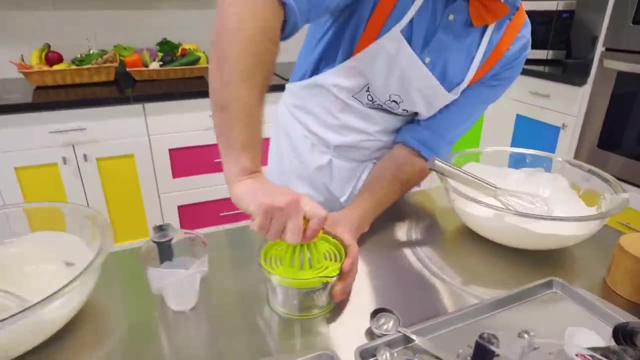 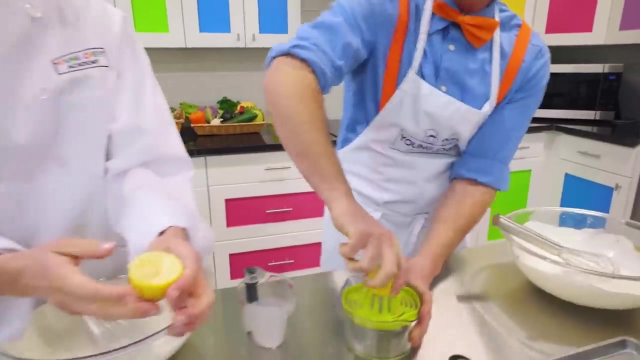 We want to make sure we squeeze really tight, pushing down and twisting it around. Get all of that juice out. Okay, I guess I'll try it. Oh, there we go. Good job, Yeah. And when you take it off, your lemon should look something like this: 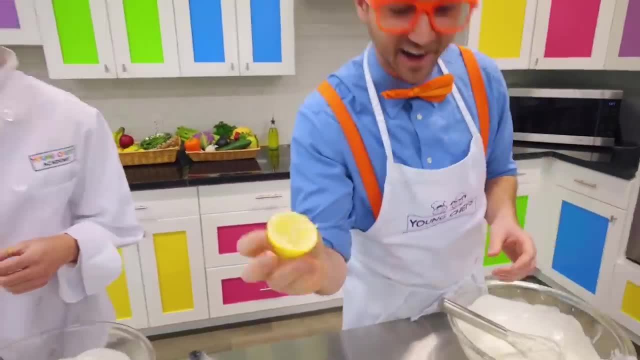 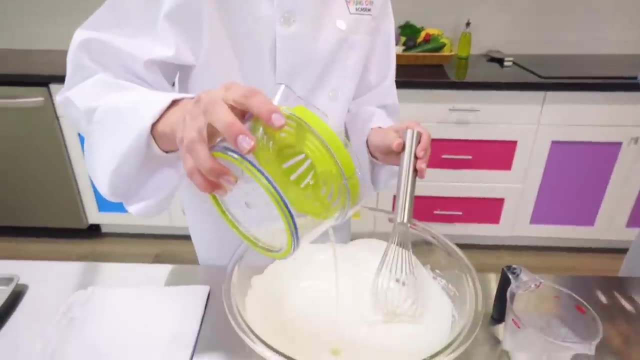 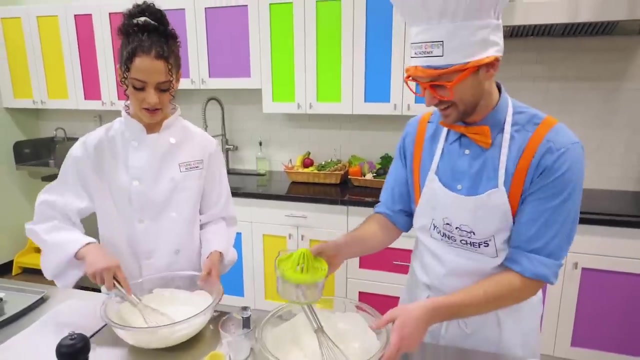 Yeah, It's almost empty. Perfect, Good job, Okay. And then we want to pour our lemon juice into our ranch. Okay, Here we go. Whee, Awesome, Okay, Awesome, Mix that up, All right, Yum. 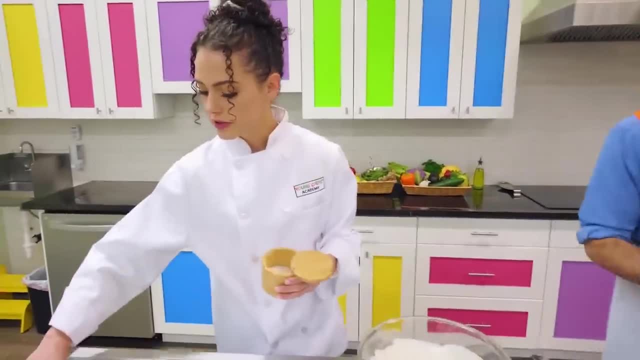 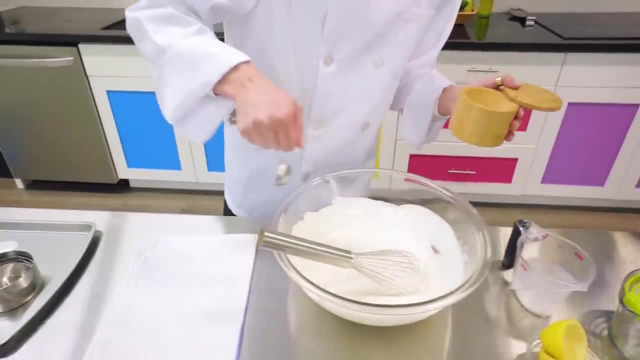 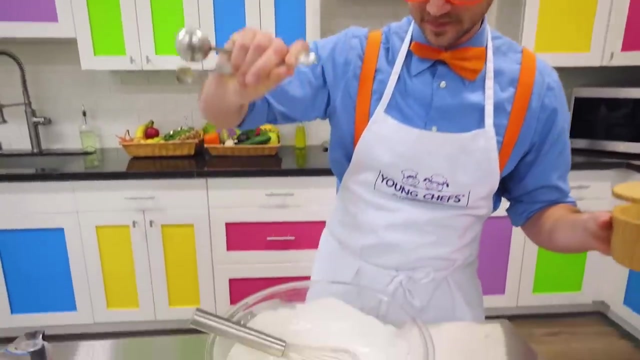 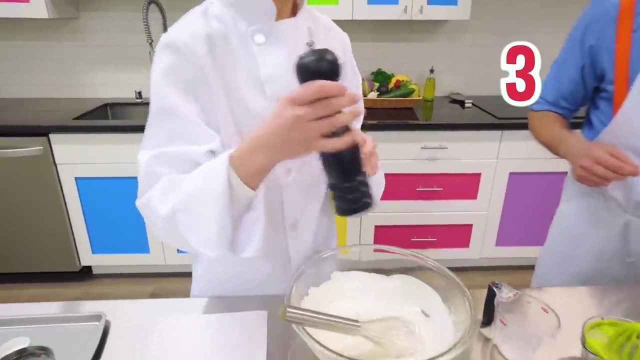 Now we want to do one-fourth teaspoon of salt, Right like this: Okay, Put some salt in here. There we go, Whee And a pinch of pepper. So we'll go about three twists, Okay, One, two, three. 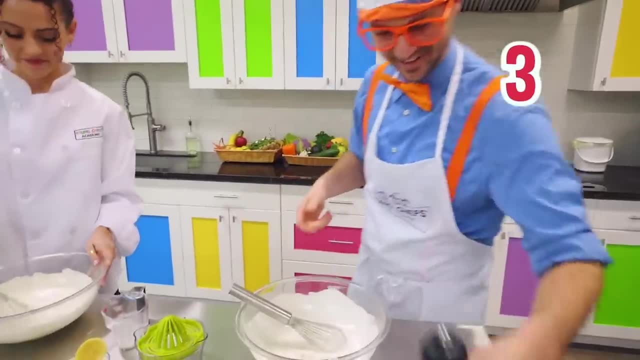 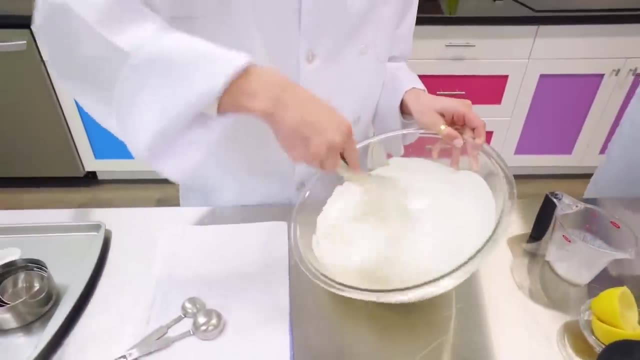 Perfect, Perfect. All right, Let's mix that up. All right, Mix, mix, mix. Remember to mix with your wrist. Oh yep, Oh wow, This is going to be so yummy, Delicious. Did you hear that? 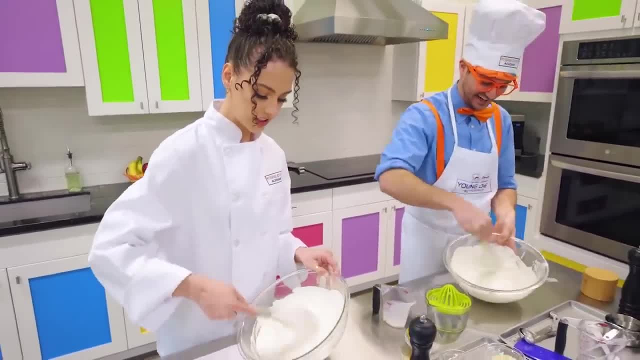 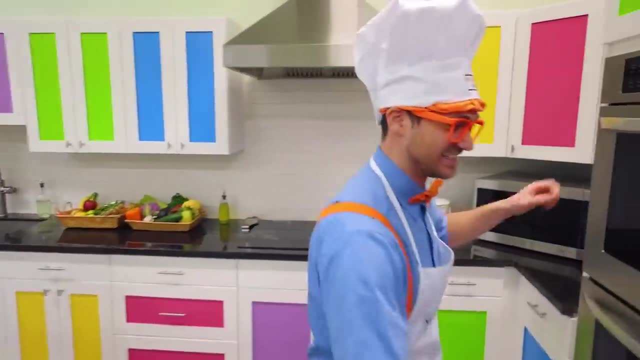 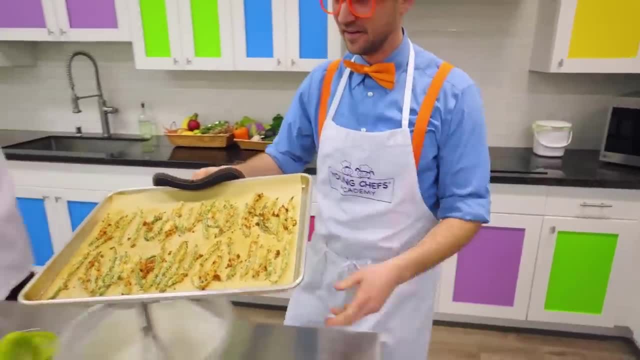 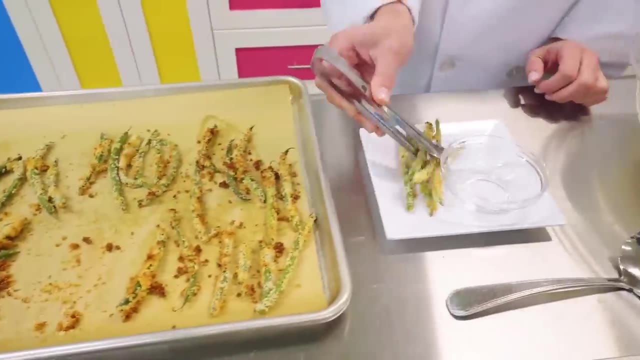 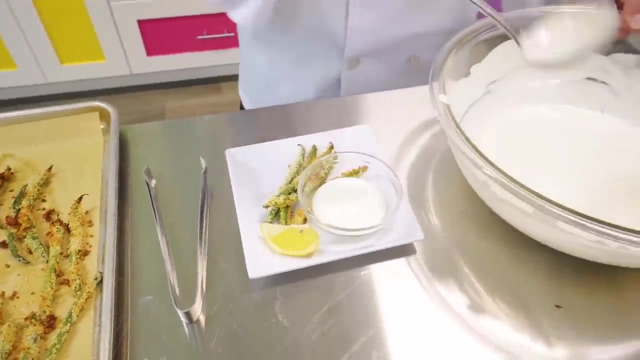 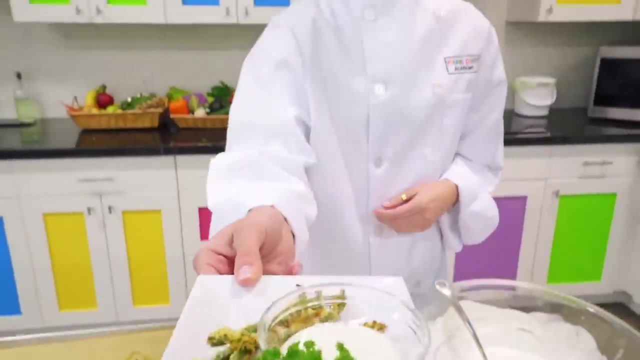 Okay, Okay, Wow, Oh look Delicious Blippy. Whoa check them out. Oh my gosh, All right Blippy. It looks like our green beans and zesty ranch are all ready. Oh, there we go. 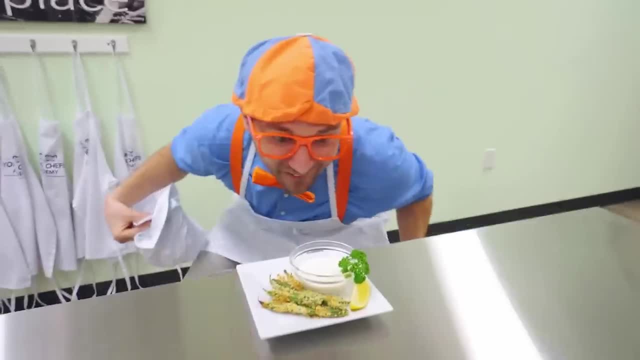 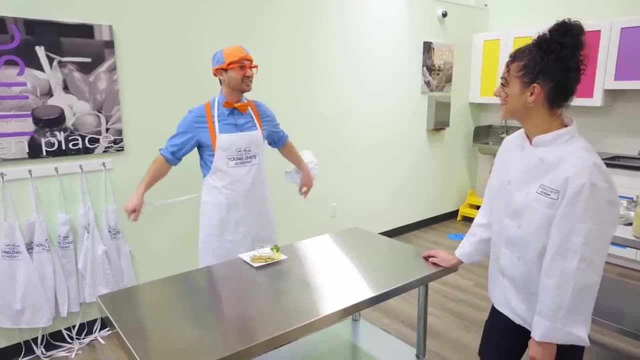 Those look yummy. Check them out. Whoa, I am so excited. Thank you so much for teaching us how to bake these. Of course, you did such a good job. Come back every time, Oh well, thank you, See you later. 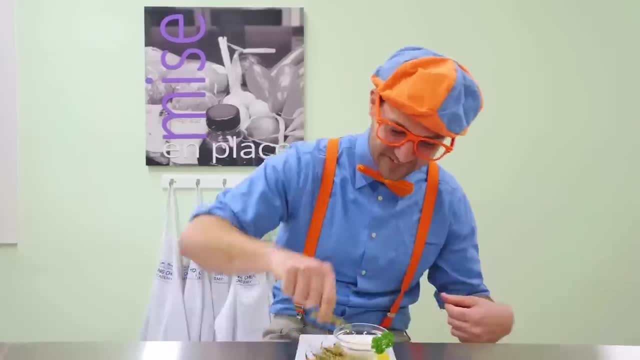 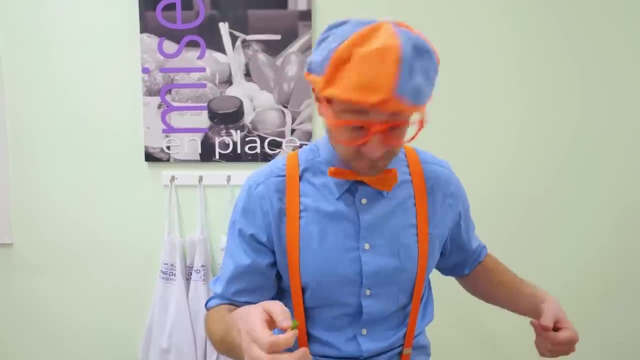 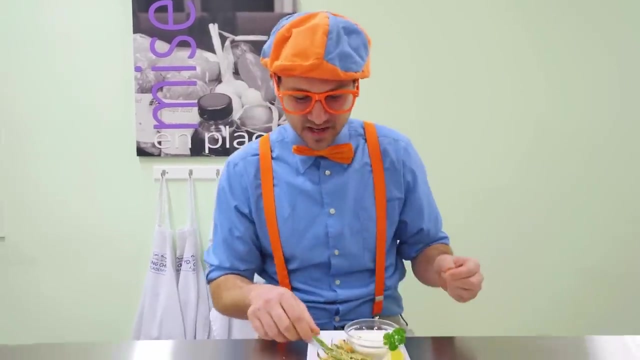 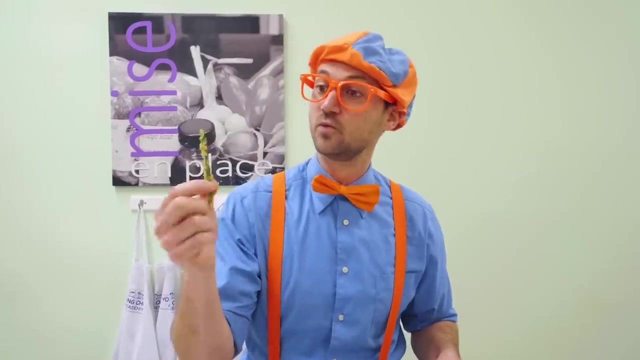 Wow, I am so excited. Here we go. Mmm, Mmm, Yum, That is dippalicious. Ha ha ha. So silly. Yeah, you'd think, because they're green they're not good. But hey, trust me, it's really fun to try new types of food. 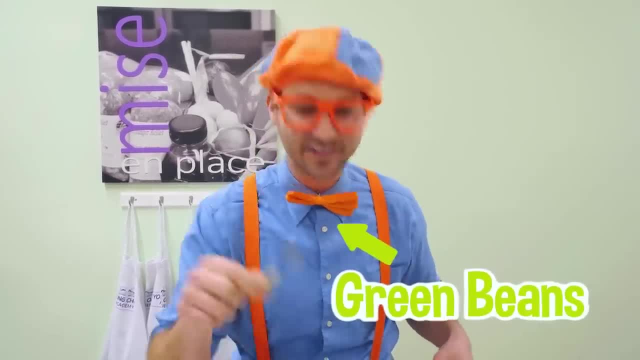 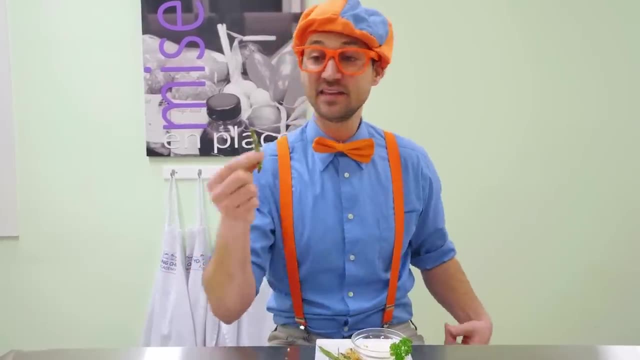 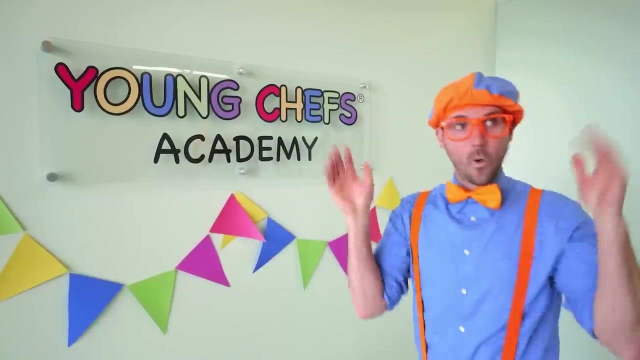 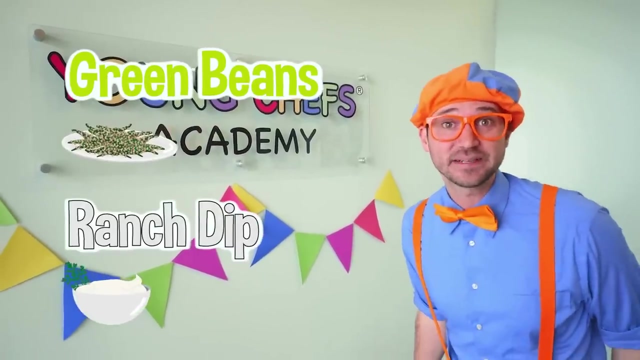 Yeah, like these yummy green beans that we made. Yeah, Mmm, Mmm, Mmm, Yum. Even healthy foods can be really yummy. Good job cooking Whoa Yee-haw Blah. Ha. ha, Wasn't that fun making those green beans and that ranch dipping sauce. 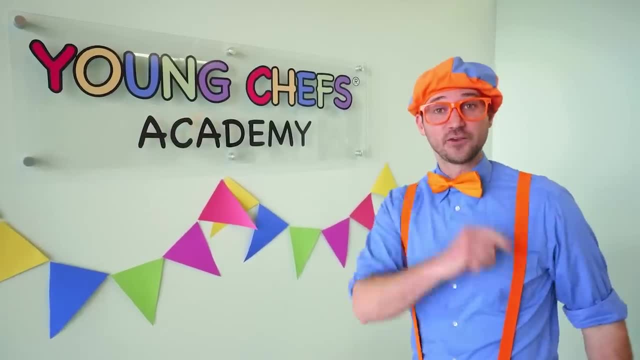 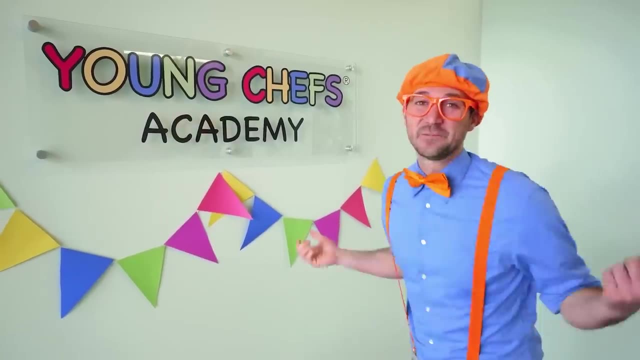 Yum, It was so tasty. Hey, if you want to check out the exact recipe, you can go to Young Chefs Academy's website and check out their blog. Woo-hoo. Well, this is the end of this video, But if you want to watch more of my videos, all you have to do is search for my name. 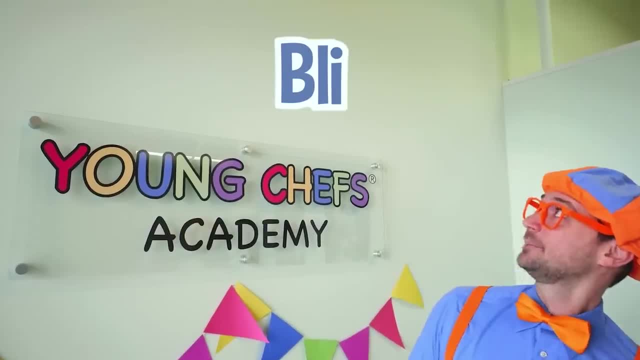 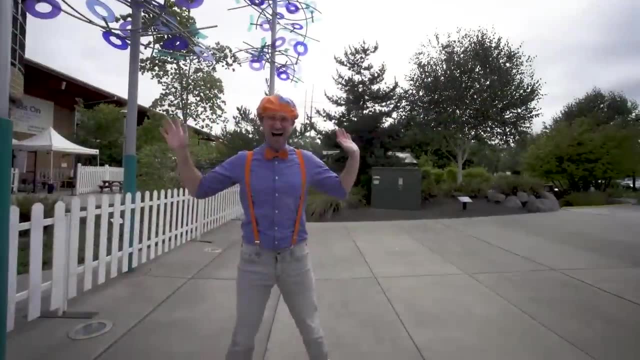 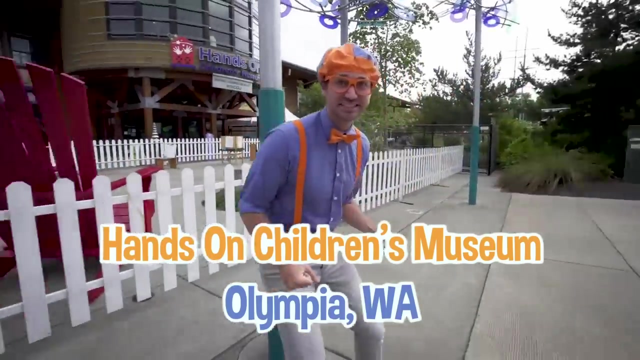 Will you spell my name with me: B-L-I-P-P-I. Blippi. Good job, All right, see you again, Buh-bye. Well, hey, It's me Blippi, And today we're at the Hands-On Children's Museum in Olympia, Washington. 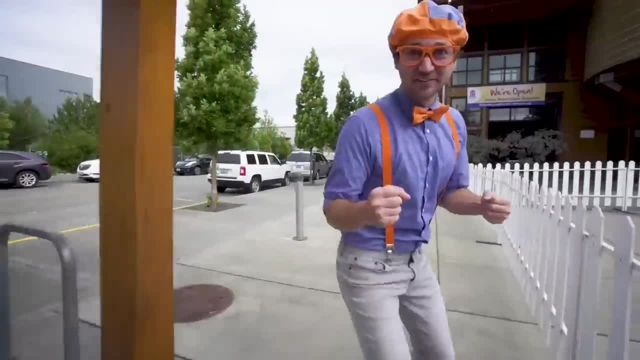 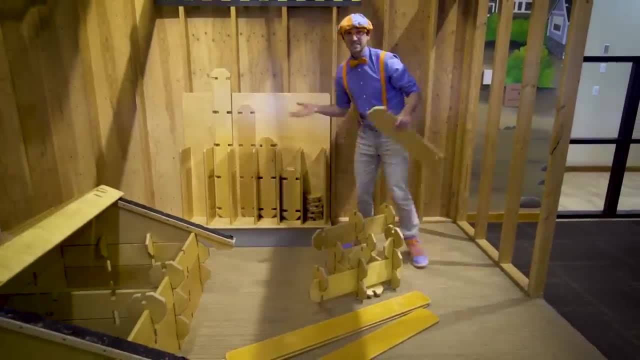 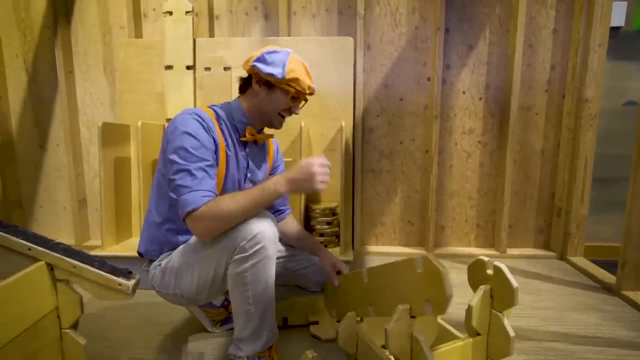 This is going to be so much fun. I love learning with you. Let's go. Ah Hey, This is the Build-A-Gallery, This is where you get to build things. Oh Ha ha, Silly me. Anywho, you put things together. 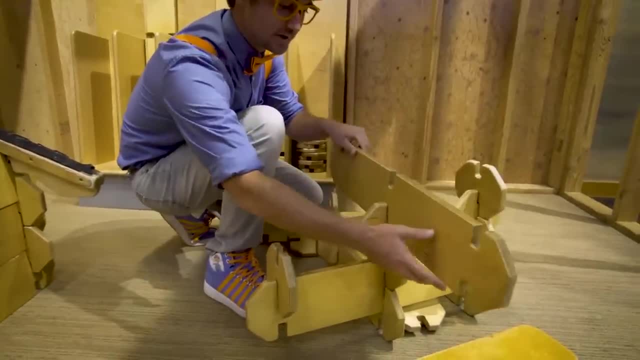 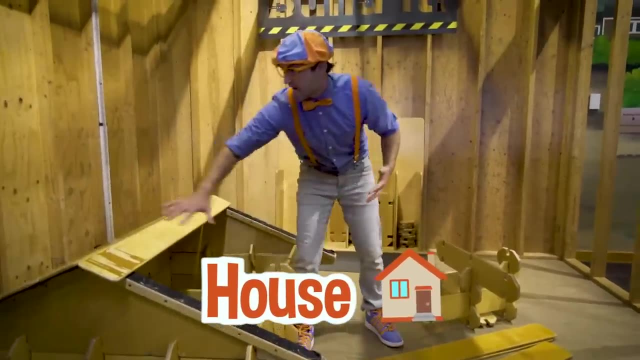 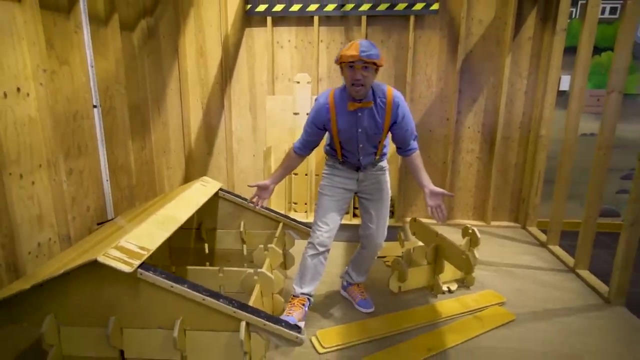 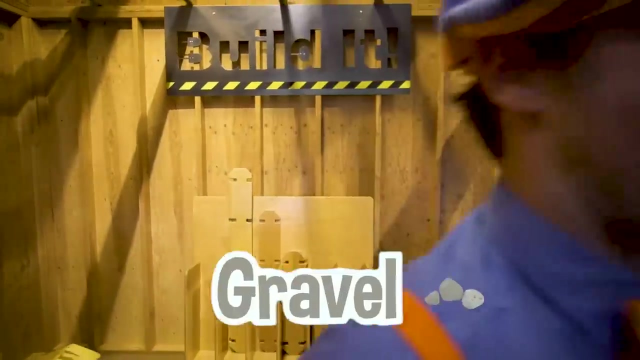 These pieces of wood And that is how you build things in the Build-A-Gallery. Yeah, I almost completed this house, Do you see it? I have a roof right here And the framing of the house And the walls And everything except for the remaining roof and some gravel. 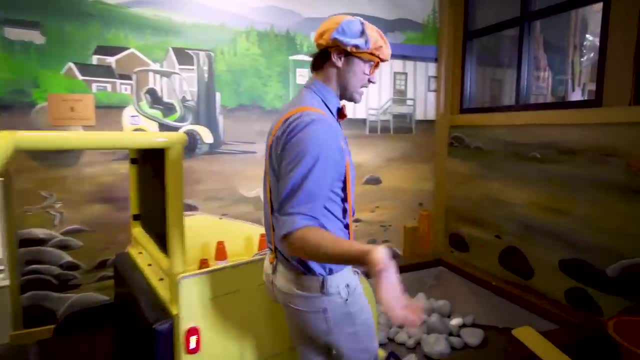 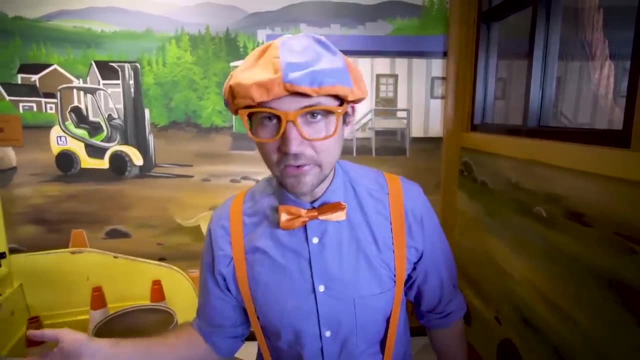 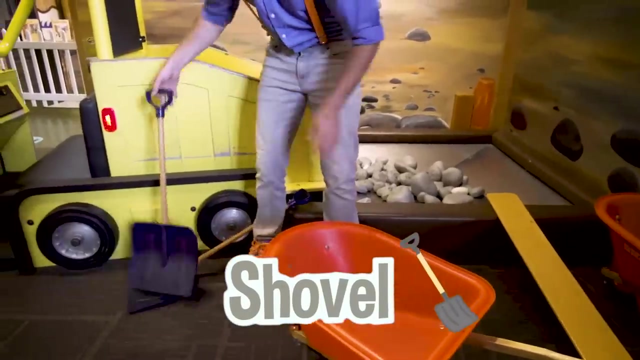 That's what we need: Gravel to go inside the house. Yeah, the floor needs some gravel. Yeah, we're not going to use carpet tile, anything like that, We're going to use gravel. So let's take this shovel and first let's drive the dump truck. 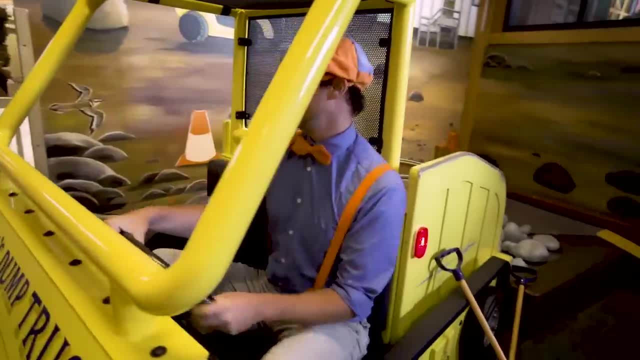 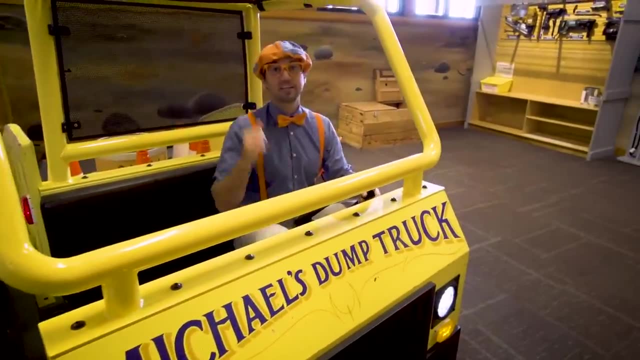 Whee, Whee, Whee, Ha ha. All right, I think we're close enough to the house. Let's go, Let's go, Let's go. We're going to drive the dump truck to the job site that we can get all the gravel out. 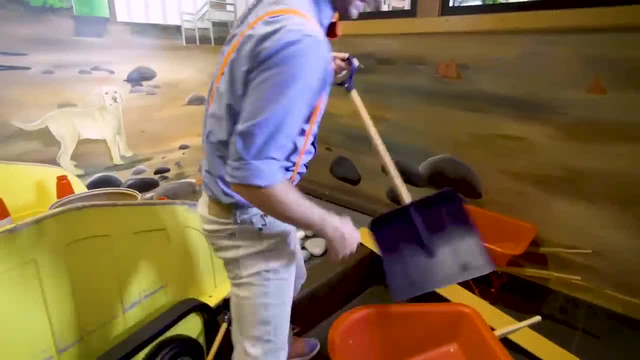 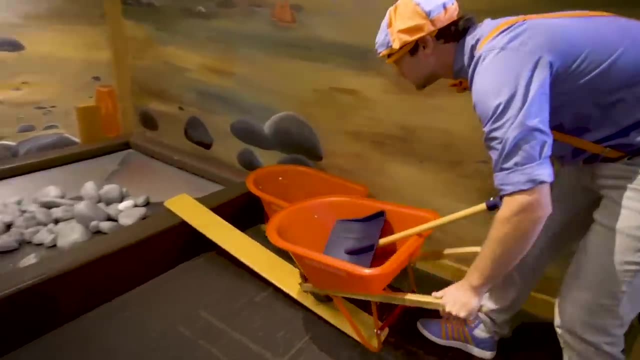 of the back of the dump truck. All right Here, Take the shovel, Put it in the wheelbarrow And then wheel it up. There we go Ugh. All right, Now we need to shovel some of these big rocks. 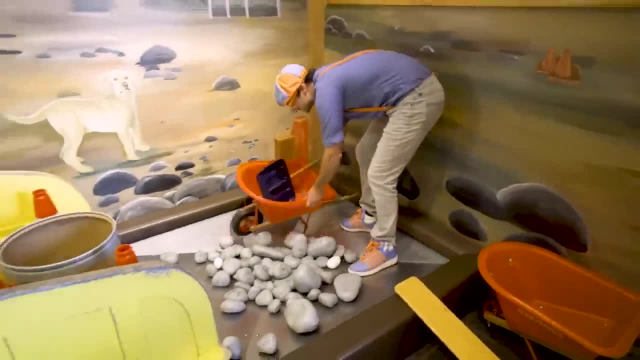 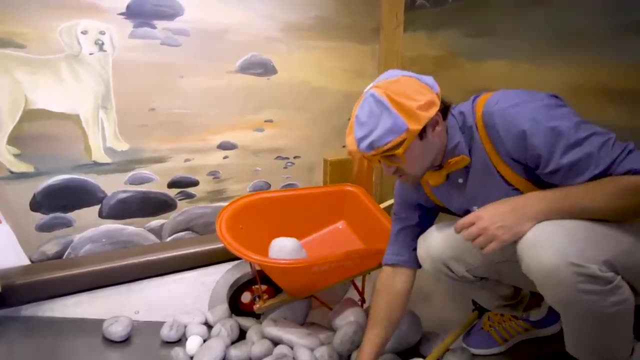 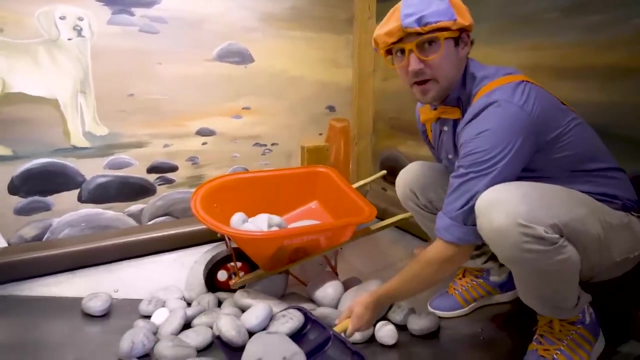 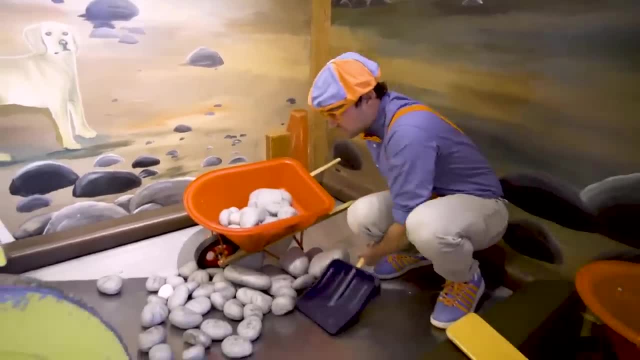 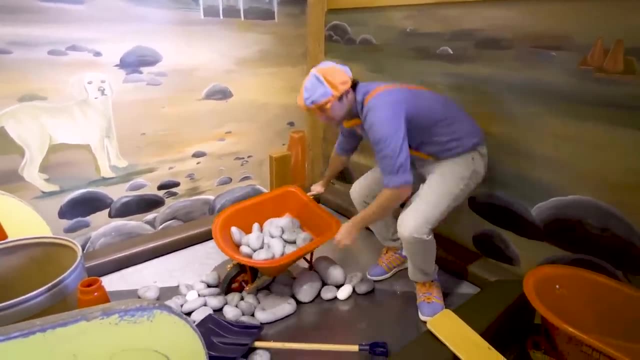 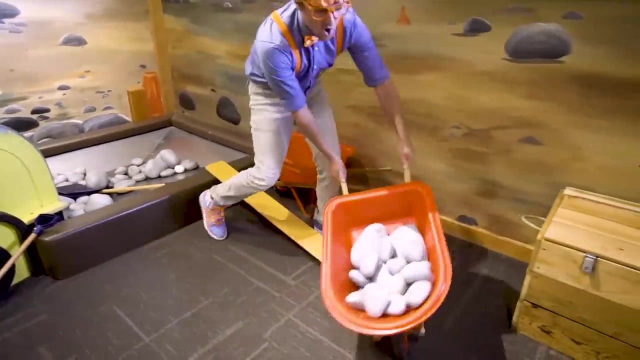 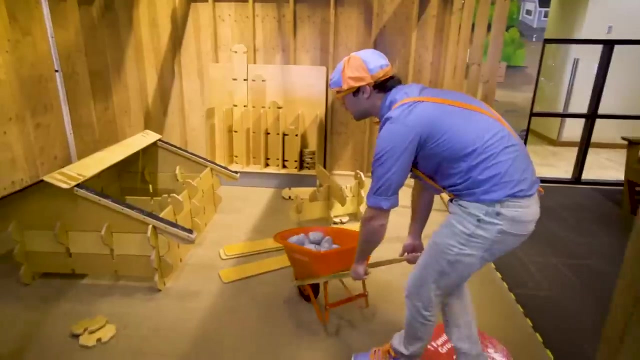 house. Okay, one more scoop. There we go. All right, now we need to take it over to the house. All right, wheelbarrows are super nice to use. It makes hauling things a lot easier. How are we going to get it in there? 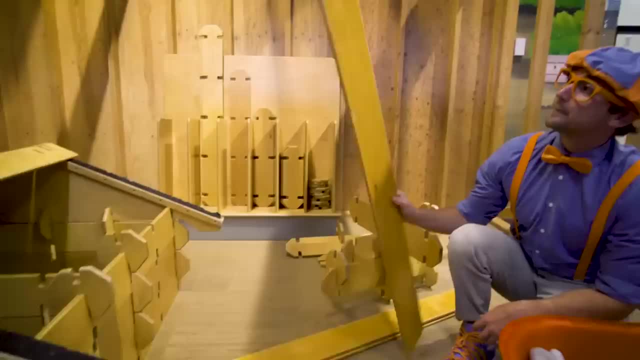 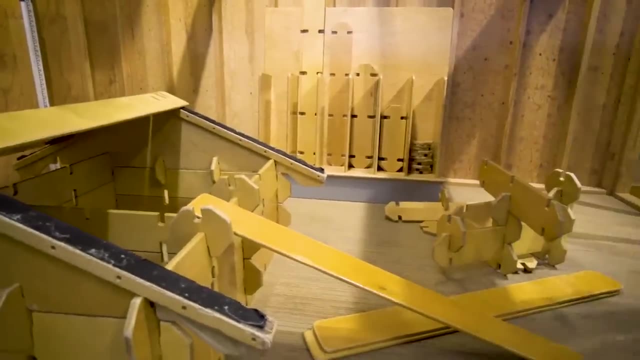 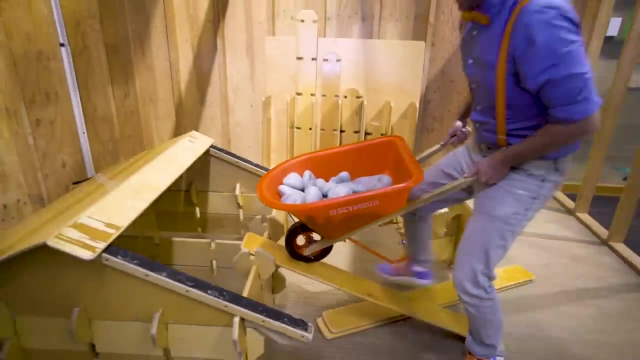 Wait a second. I have an idea. Maybe we can use one of these boards that actually should go on the roof, But for now let's lean it up like this, and then let's take this wheelbarrow, go up and 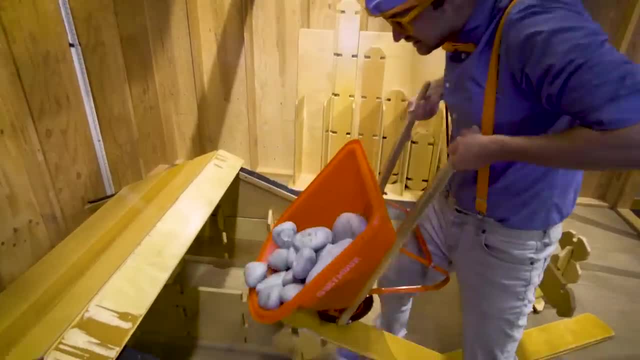 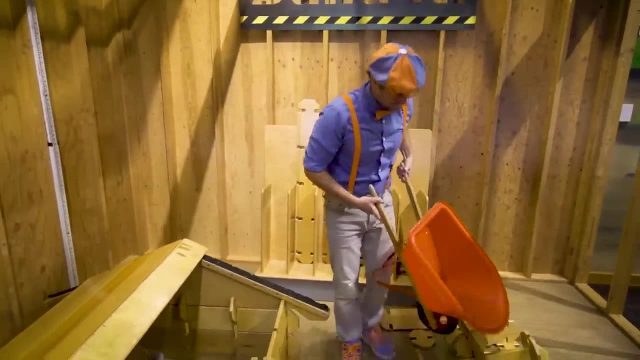 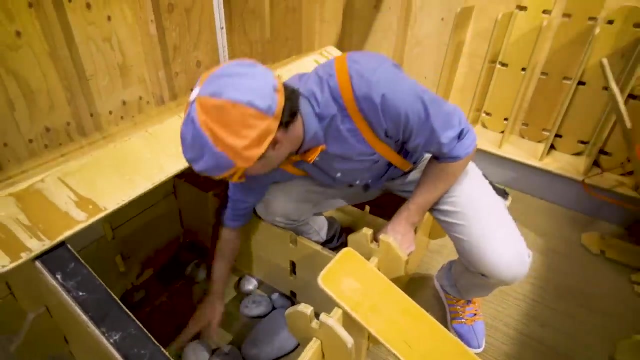 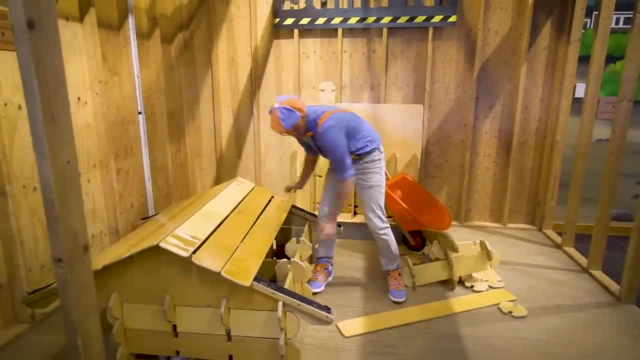 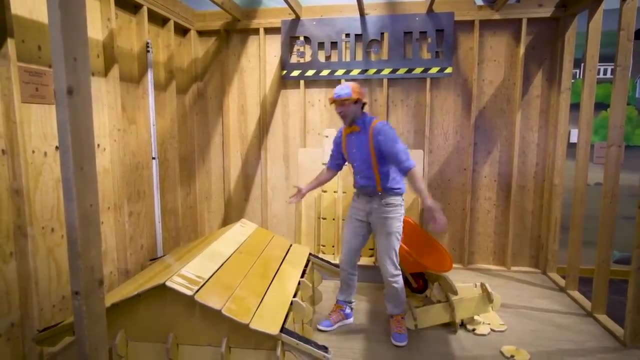 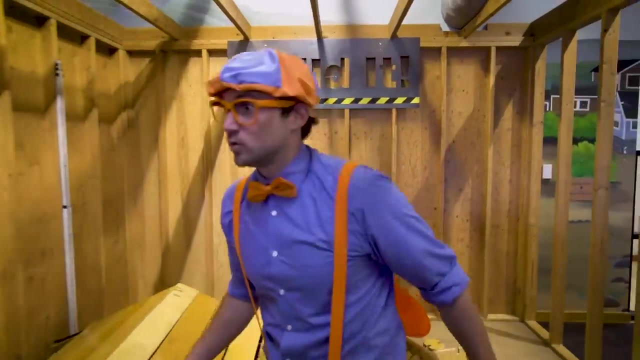 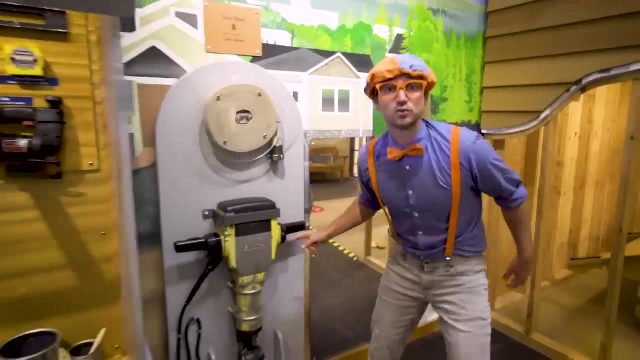 A hard day's work right there. There we go. That looks like a great house. I'm tired, hey, but before we go to another room, I think we should check out the rest of the tools like this. there's a lot of tools in here. you know what tool this is. this is a jackhammer. watch how. 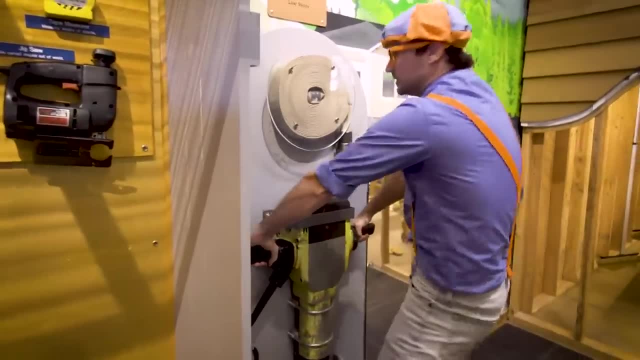 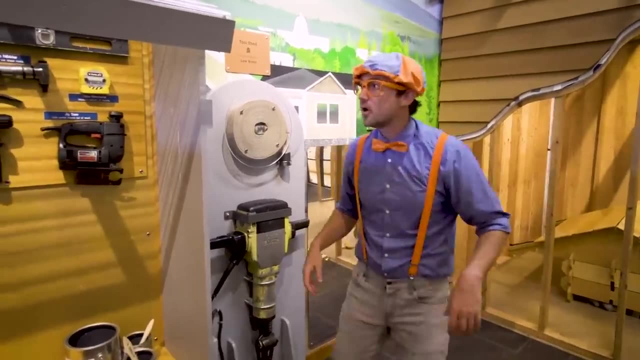 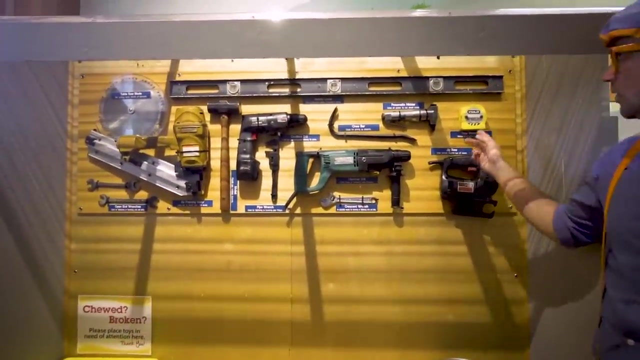 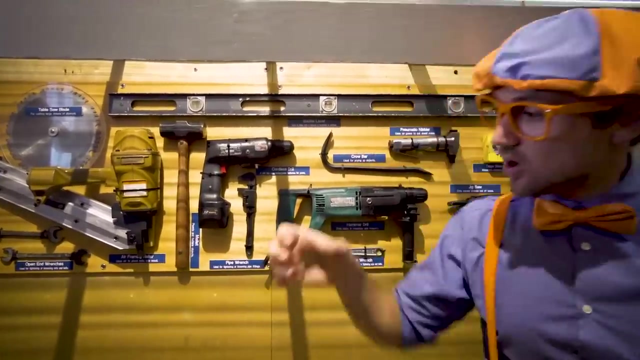 it works. whoa, it goes up and down super fast and breaks the ground up. whoa, and look at all of these. looks like we have a tape measure, so then we can measure things. oh, looks like we have a cordless drill, so then we don't have to go really slow with our hand. this just goes. 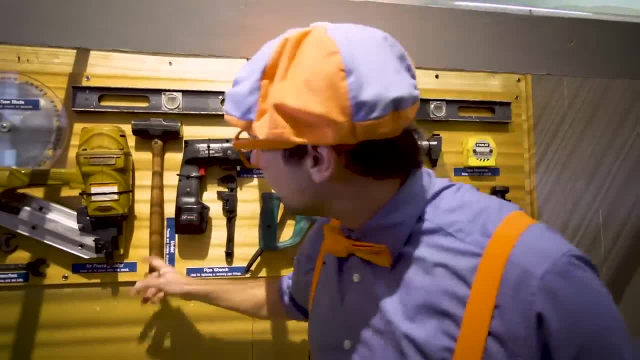 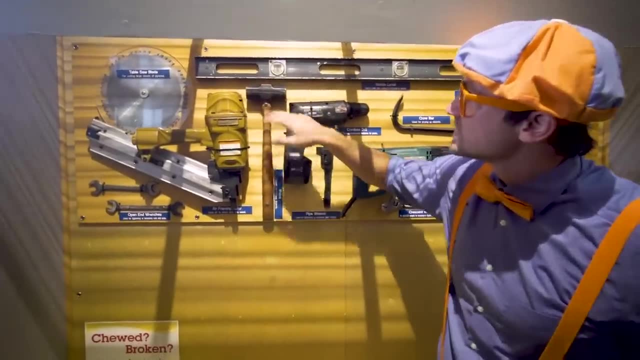 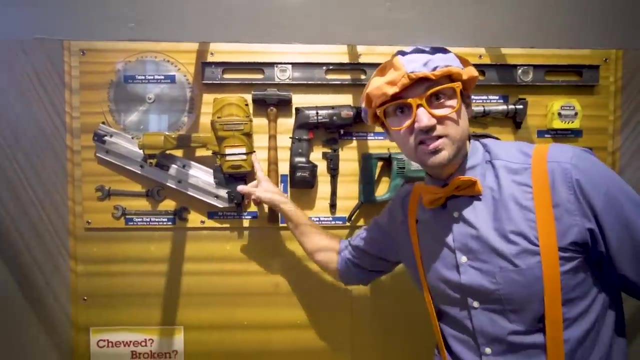 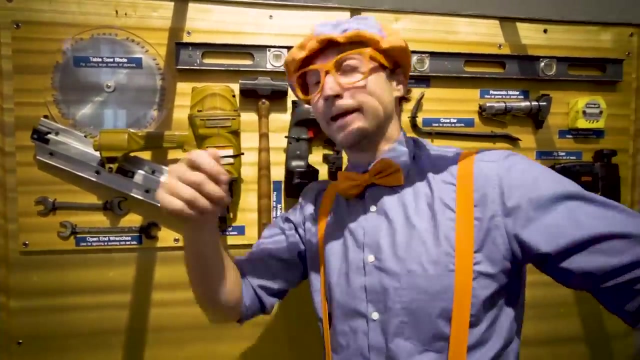 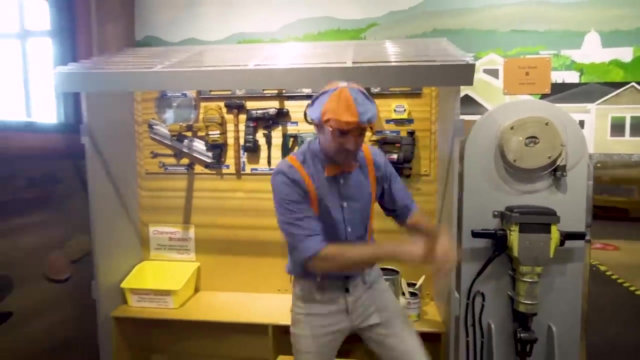 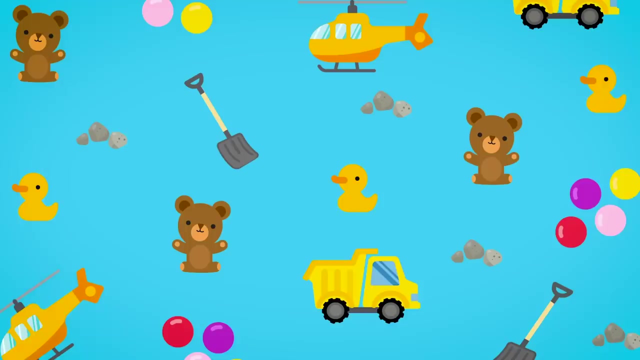 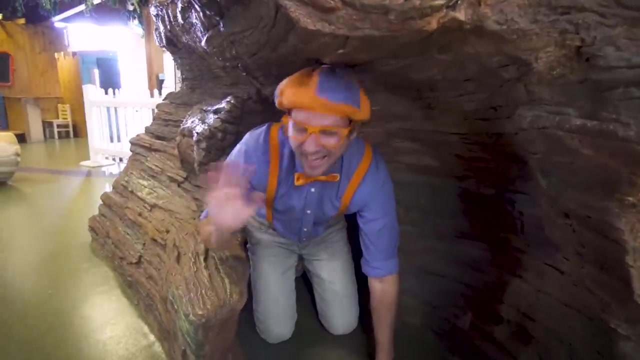 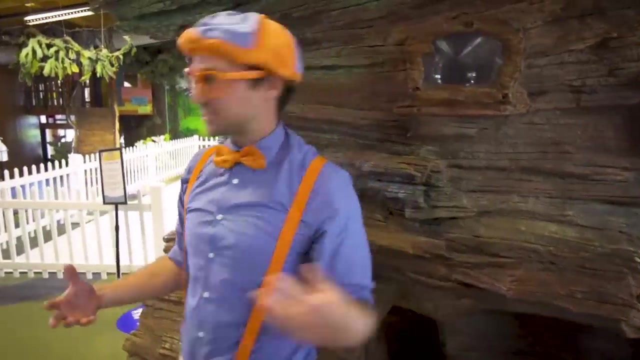 whoa, and a big mallet- yeah, they're kind of like a hammer, but with bigger heads on it. and check this out- an air framing nailer. this is what you use to secure the roof. yeah, with nails. hey, I was just acting like a bear in hibernation. bears love to hibernate during wintertime keeps. 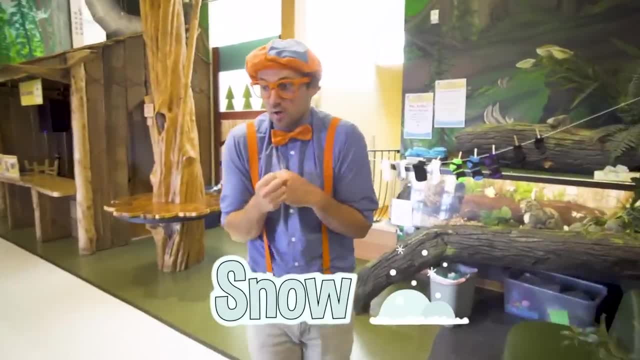 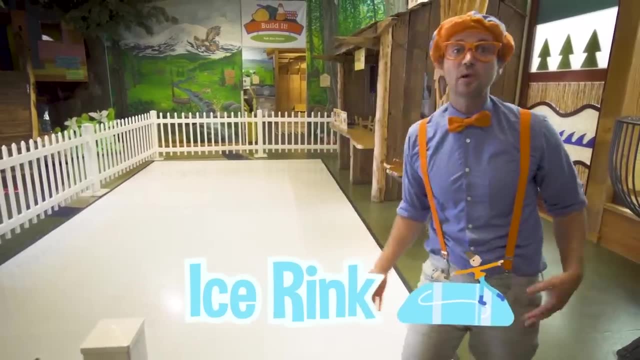 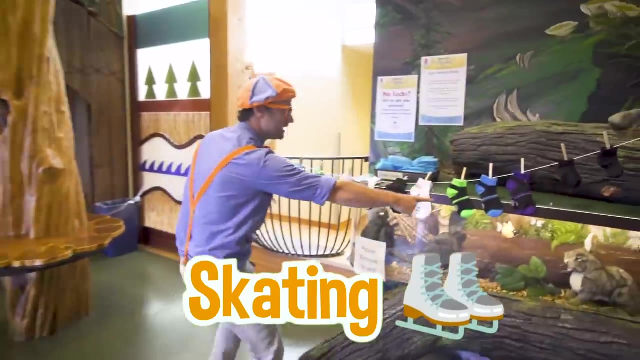 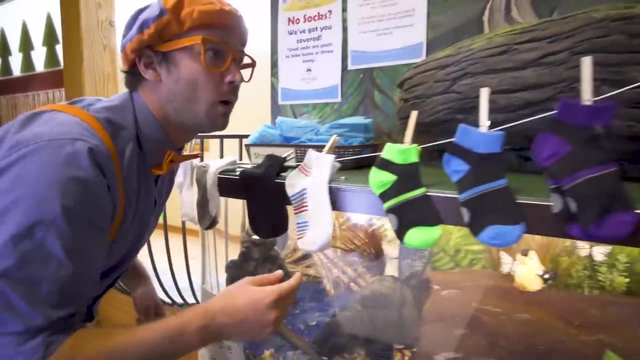 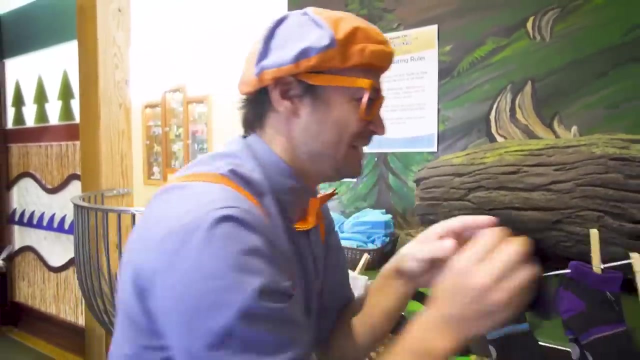 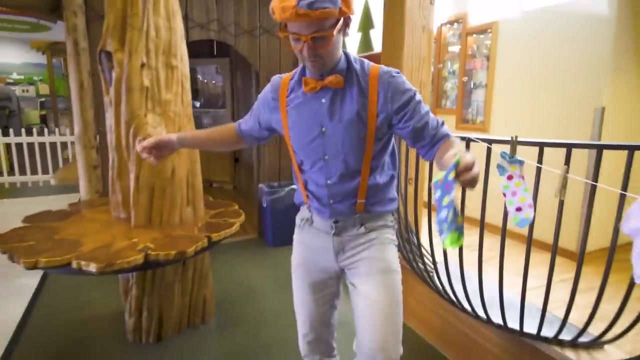 them nice and warm under snow. oh, speaking of snow, this is an ice rink. yeah, when water freezes, it turns into ice and I think you and I should go skating. well, first we need to pick out some socks. hmm, let's see which socks look nice. oh, wait a second, these look pretty cool. all right, take off my shoes. 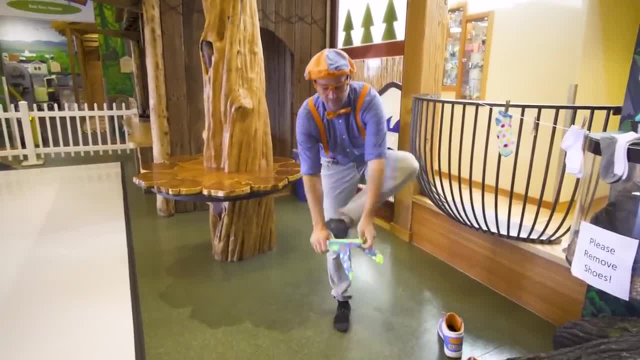 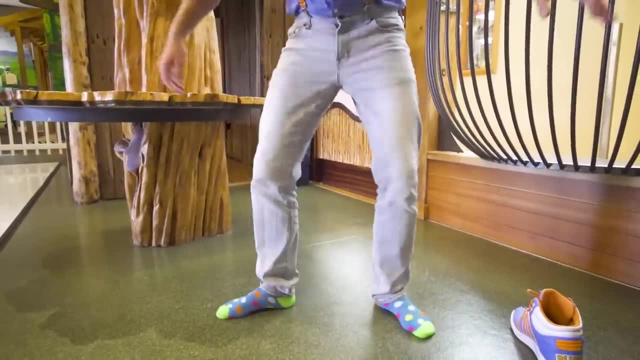 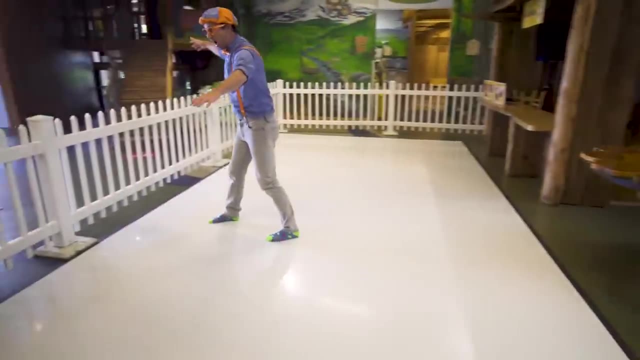 Yeah, I already have socks on, but that's okay, These are really cool And I'm gonna put them on the outside of my feet. Are you ready? Ha ha, three, two, one, Whoa, Whoa. it's so slippery. 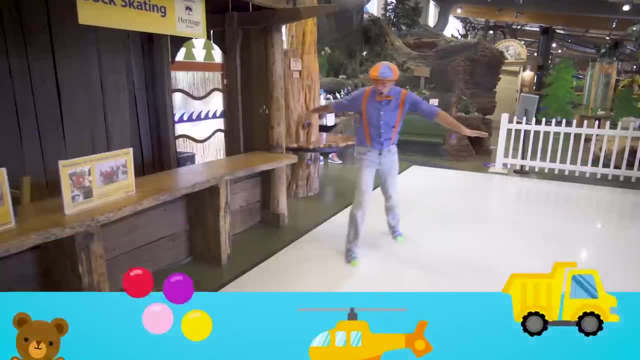 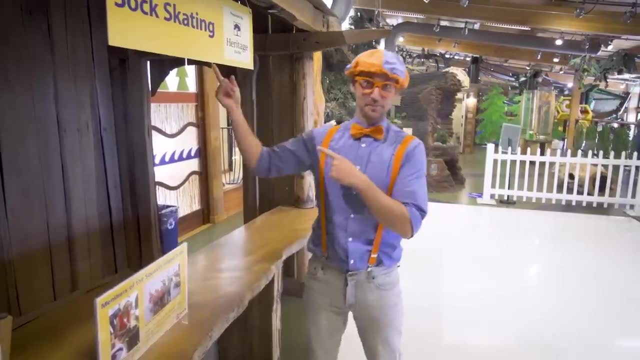 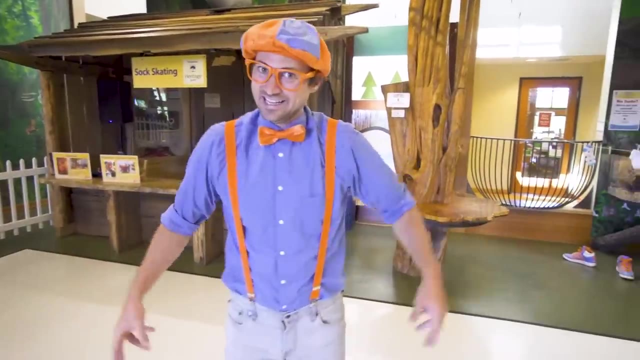 Whoa, ice is so slippery. Whoa. Remember earlier how I said this is ice. It's actually practice ice for the sport of sock skating. Ha ha, Hey, I have an idea. Why don't I do a dance for you? 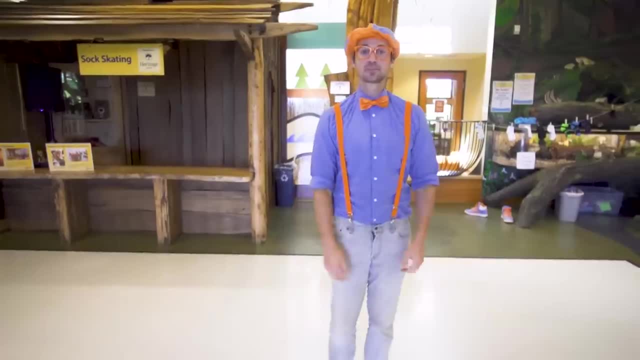 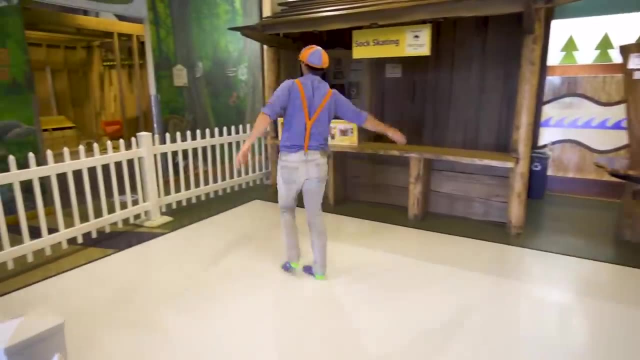 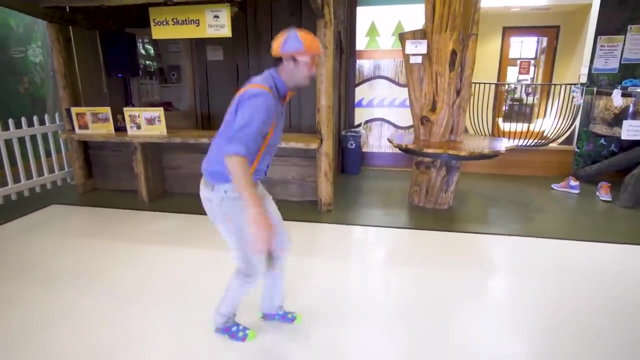 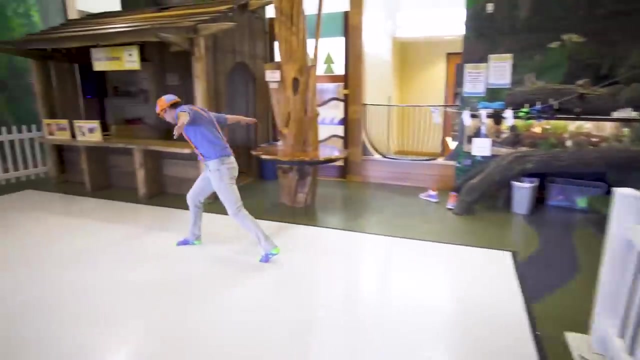 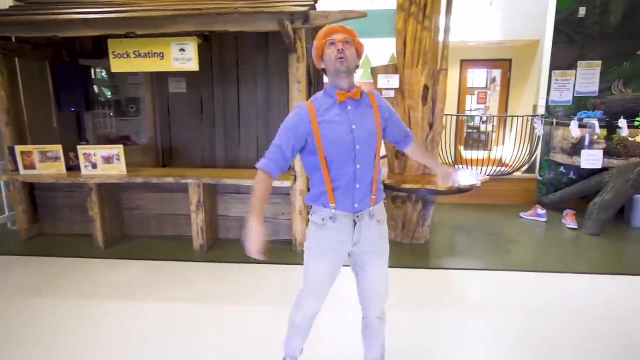 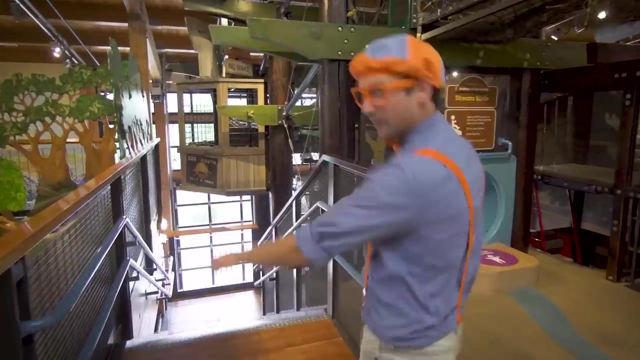 A figure skating routine. Are you ready? Hit the music. Okay, let's go downstairs now. Wait a second. The cool thing about this children's museum is that it's not just for kids, It's for kids, It's for kids. 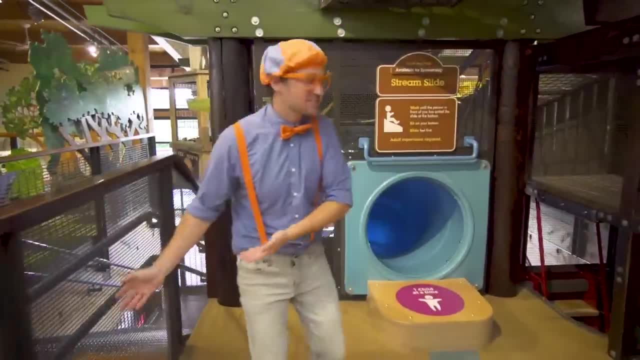 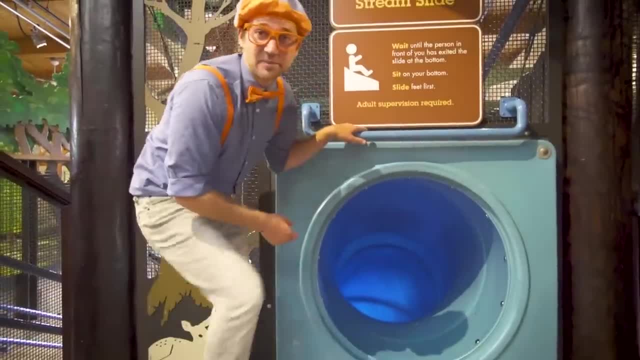 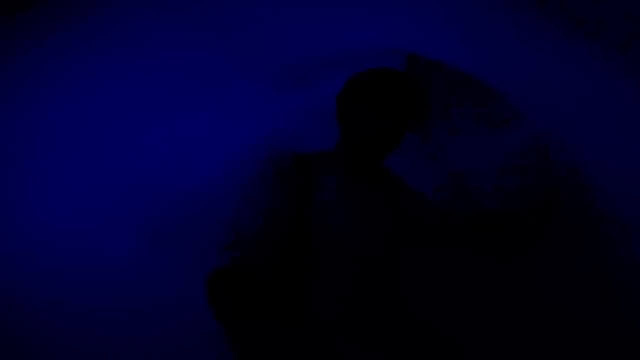 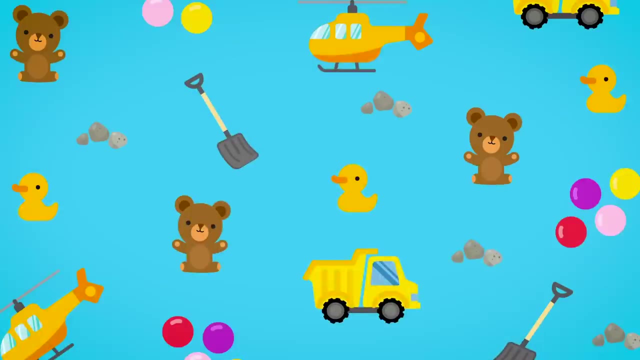 If we want to do this again. Naturally, You can go downstairs with the stairs as well as the slide. That's right, I'm gonna go down the blue slide Ready, See you down there. Whoa, What a fast way to go downstairs. 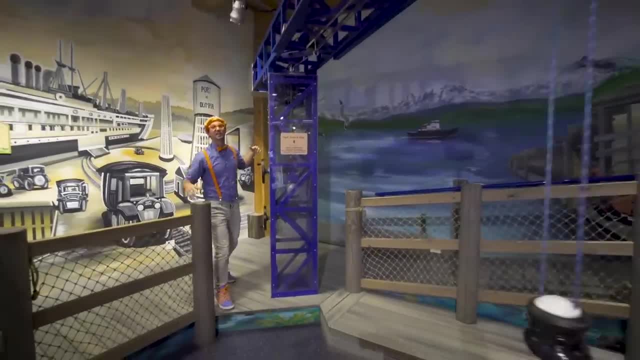 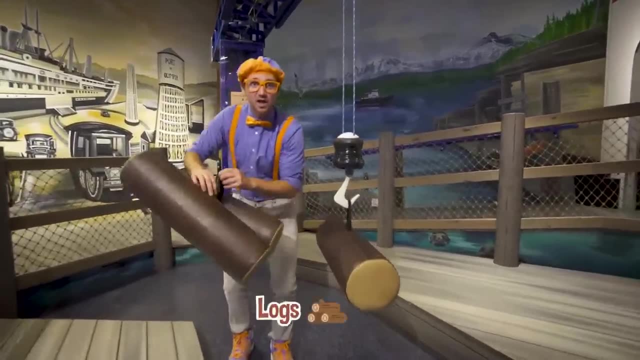 Ha, ha, Whoa. I'm at the Port of Olympia, Whoa, and check this out. This is a giant race. Whoa, Hey, and look, we have some logs. Yeah, two logs that turn into lumber later. 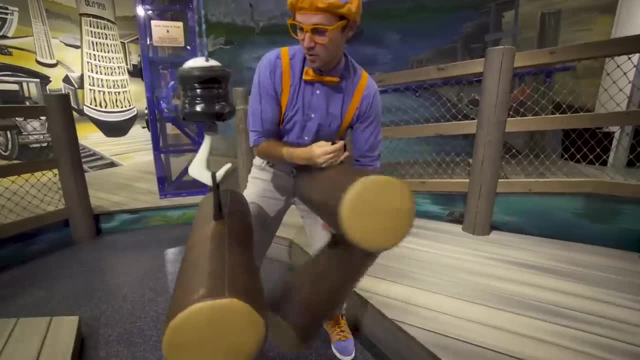 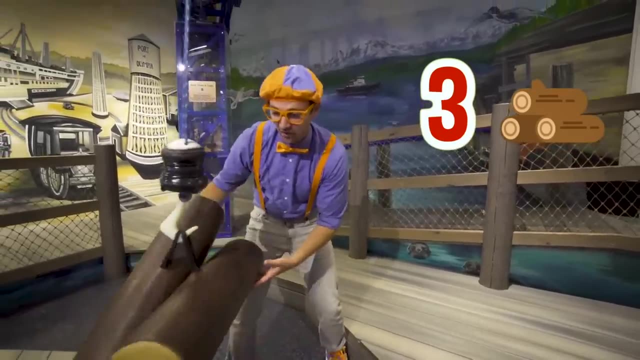 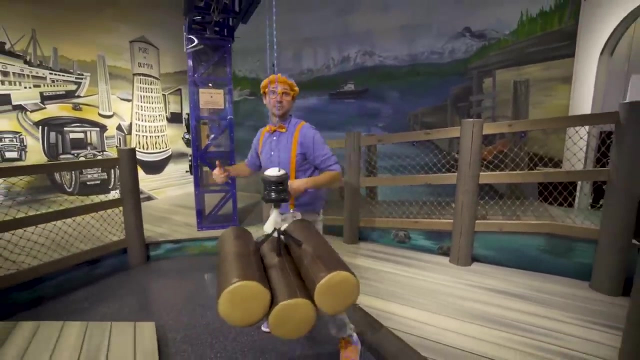 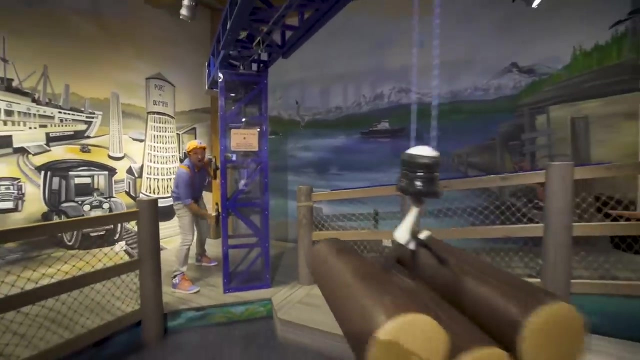 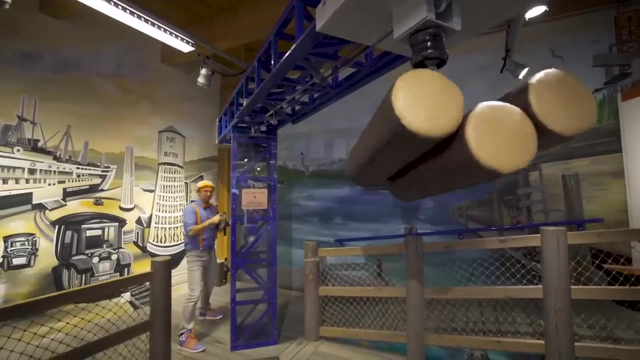 Alright, let's hook them up to this hook. One log, two logs, three. oh, two, three logs. Alright, now I'm going to go hoist it up. Yeah, Woo-hoo, There we go. Alright, we took it off the ship. Now we're going to bring it all the way back. 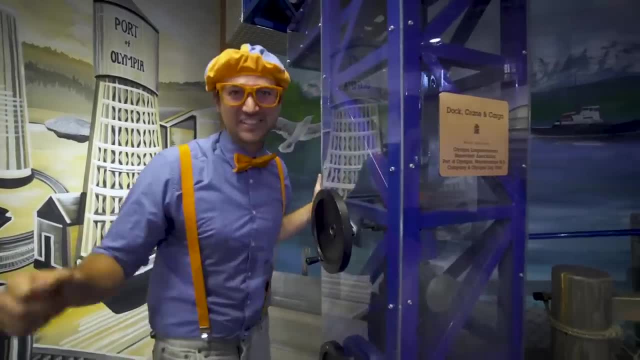 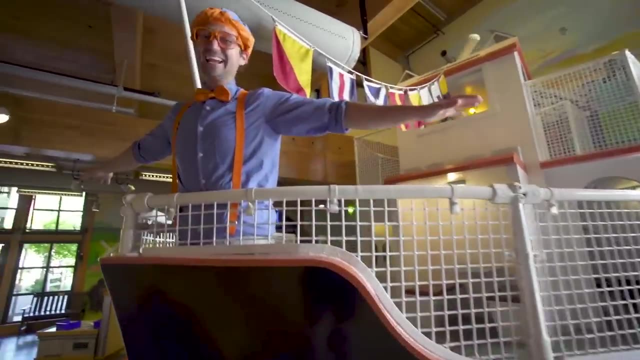 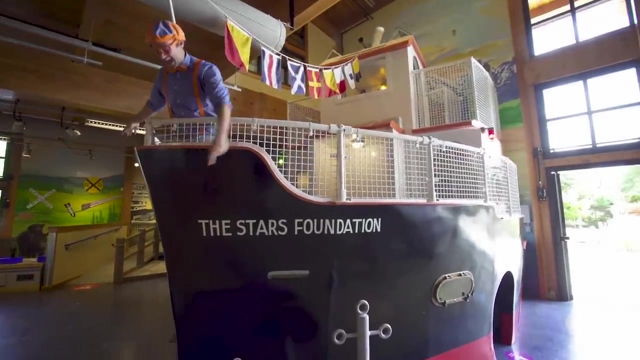 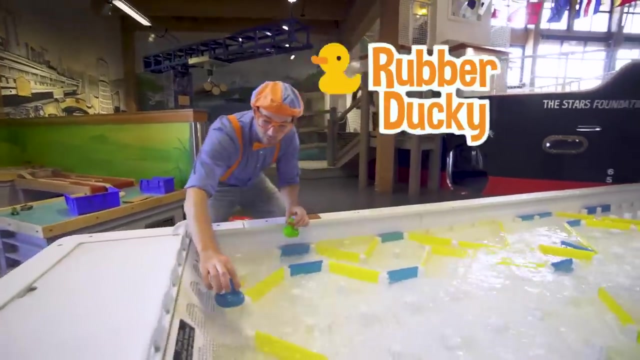 Whoa, That was awesome. Good job, Alright, let's go. I'm flying, Blippi, I'm flying. Yeah, Woo-hoo, Dolphins. Hey, check this out. Whoa, this is so cool how you put the rubber duckies on this end and then the water flows downhill and then they go. 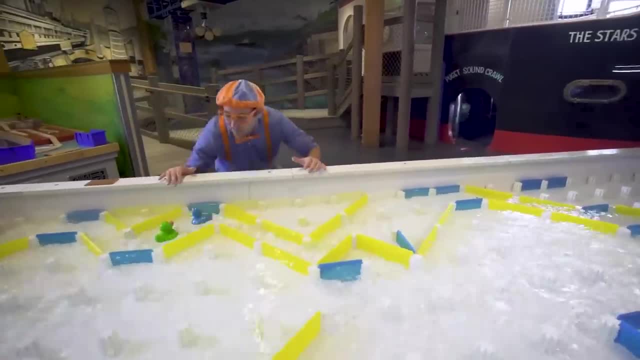 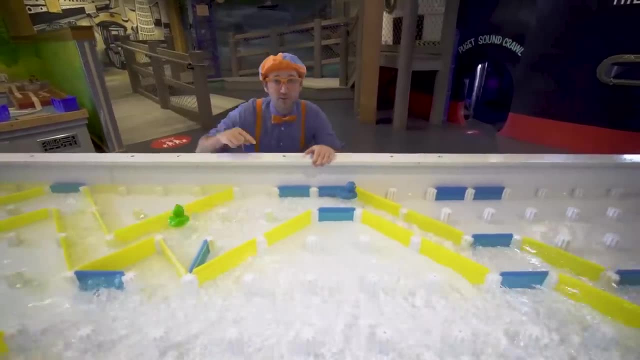 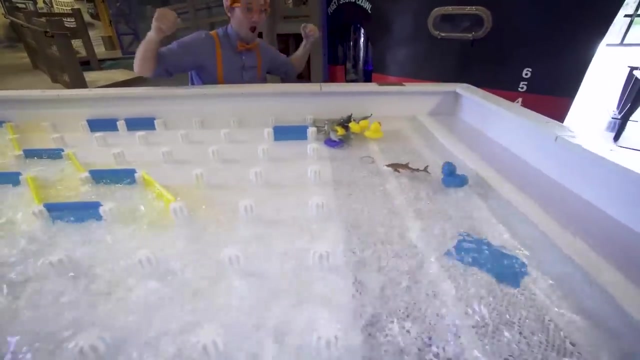 Woo-hoo, Wee, Look at them. Whoa, Hey, Whoa, Oh, whoa. I bet Blue is going to win. Oh, Green got stuck. See you later, Green, Yeah, Blue, Woo-hoo-hoo-hoo. 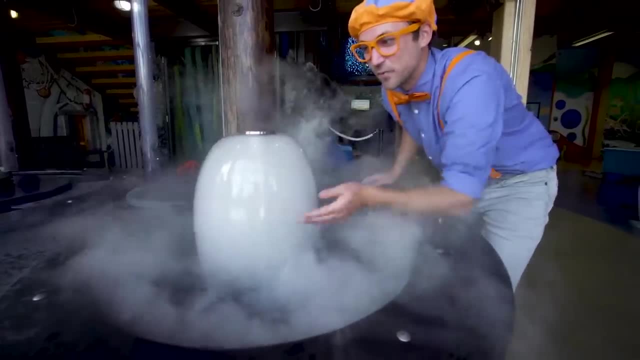 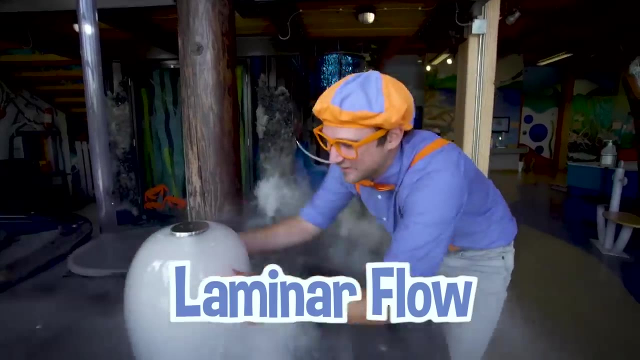 Whoa, Whoa, check this out. When water does this, when it's really smooth, it's called laminar flow. Oh, whoa, But check it out, there's actually smoke on the inside. Whoa, Oh, now I'm all wet. 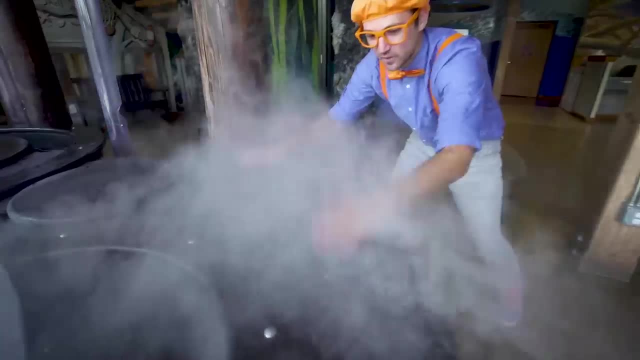 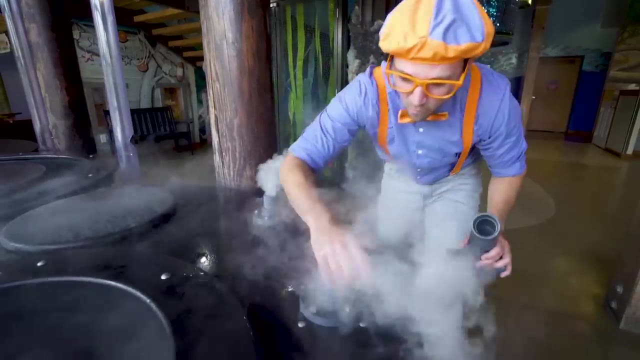 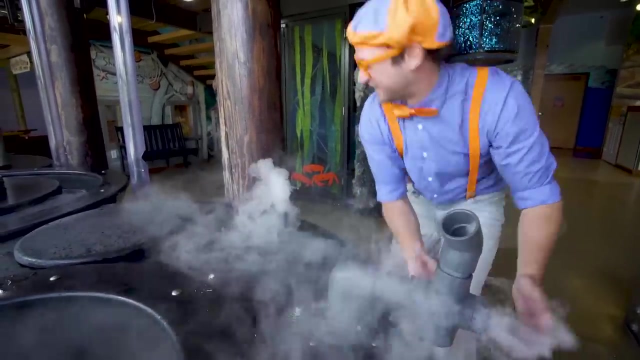 Whoa, look at these two tubes. They have smoke coming out. Check this out. Whoa, When you add these pipes, you can direct where the smoke goes. Whoa, That's so cool. Oh, Check this out. What is this? 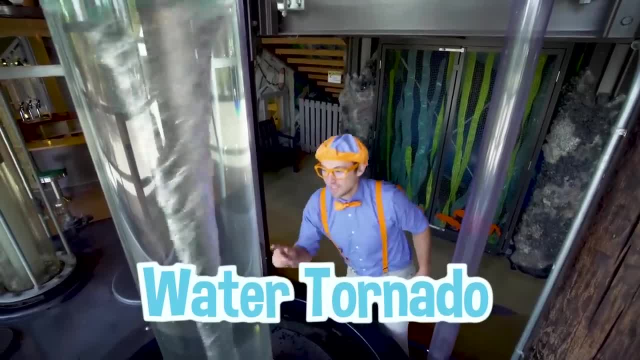 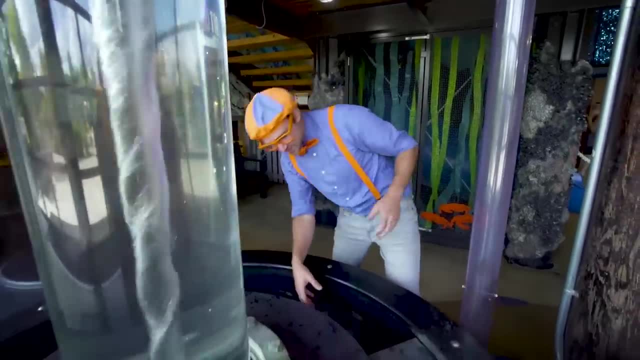 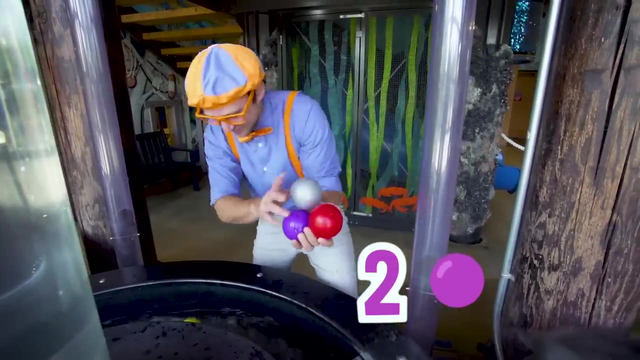 It looks like a water tornado. Its name is the volcano. So cool, Hey. speaking of balls: whoa, we have one ball, two balls, Where are you? Three balls, Four balls, Okay, now just three balls. Let's get one more ball. 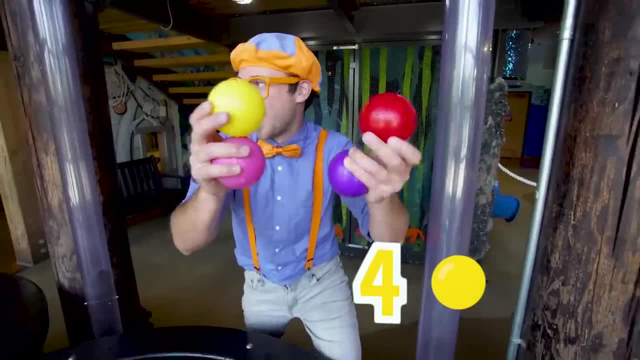 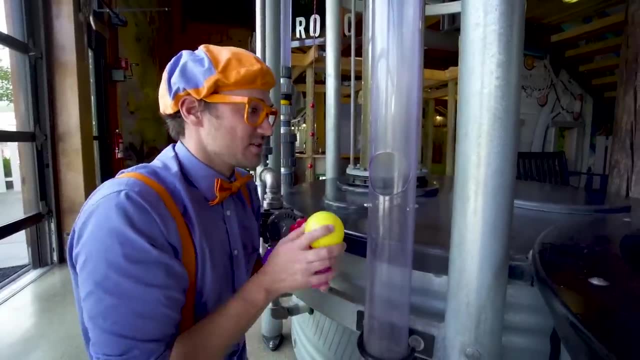 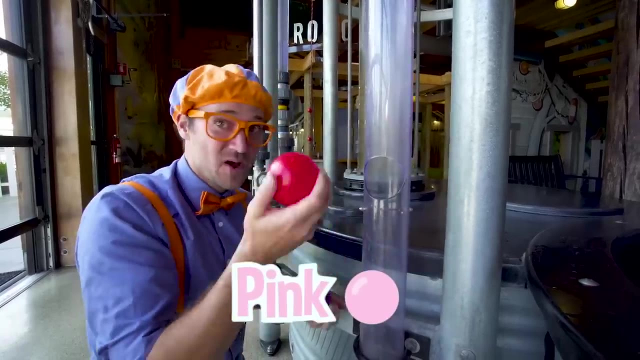 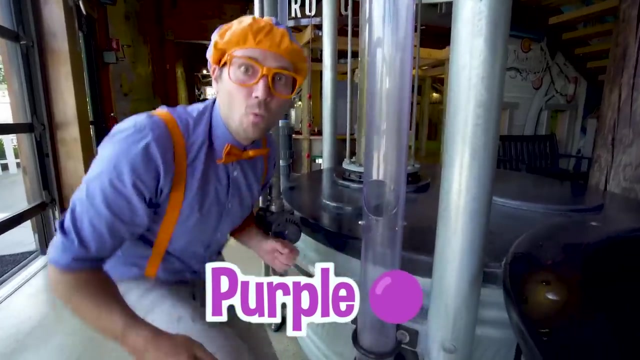 Four balls. Okay, let's go over here. Whoa, and this hole is where you put the balls: One yellow ball, One pink ball, One red ball, One purple ball- Whoa, where did they go? I don't know. 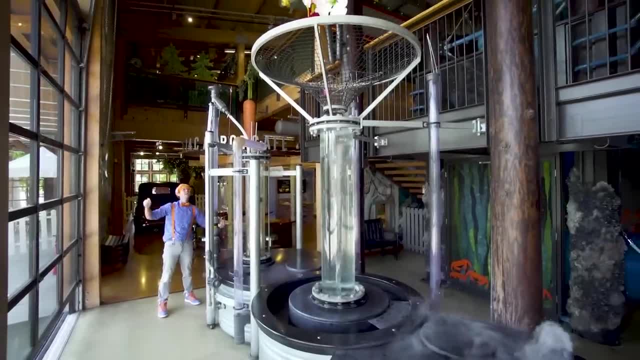 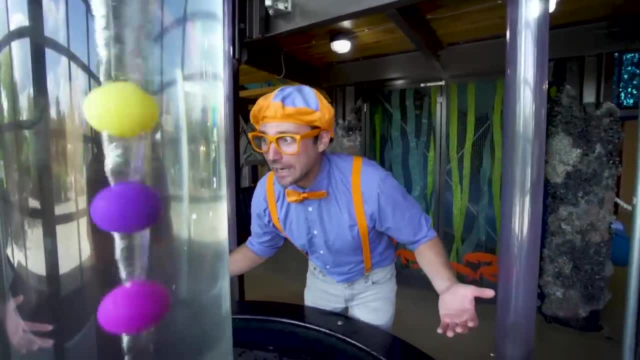 Check this out. Three, two, one, Whoa. Yeah, We did it. Wait a second, That was five balls. What? Yeah, Whoa, Check it out, I'm driving this police car. Yep, we have the steering wheel. 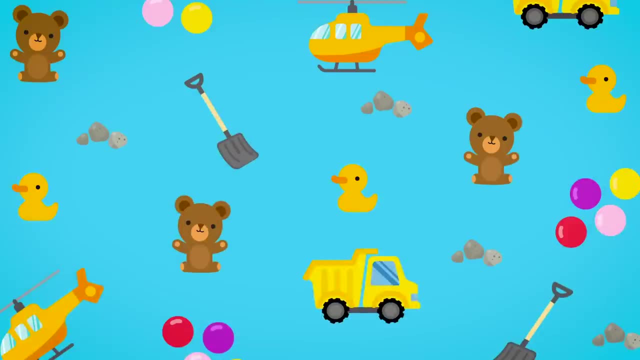 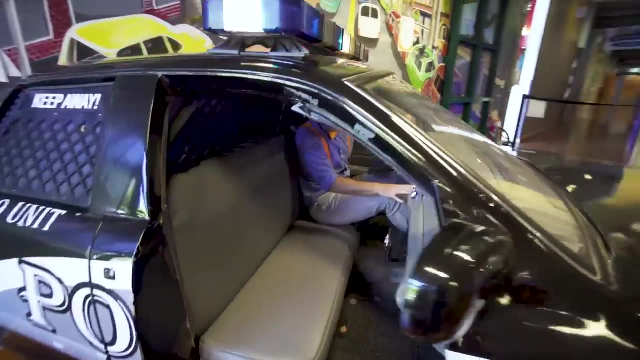 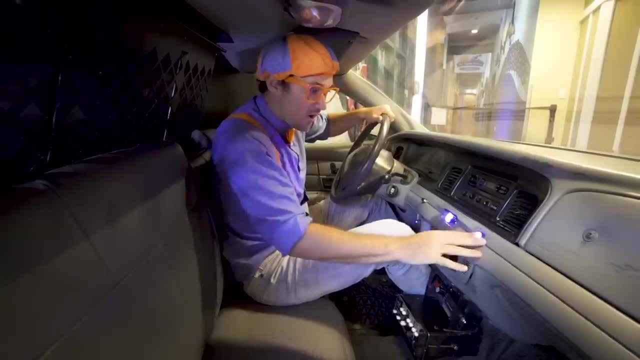 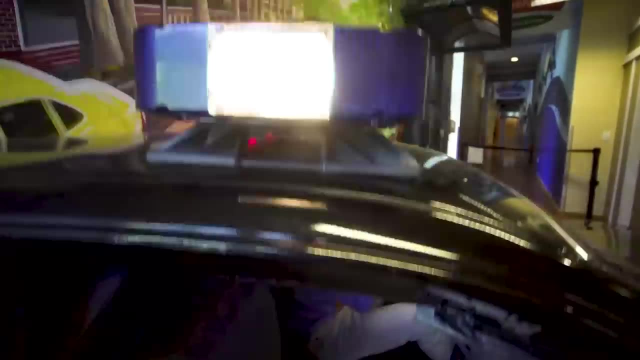 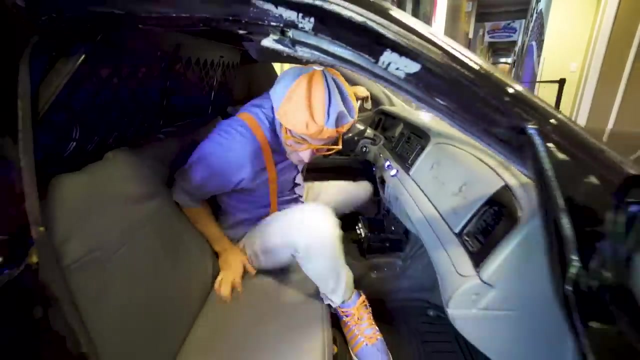 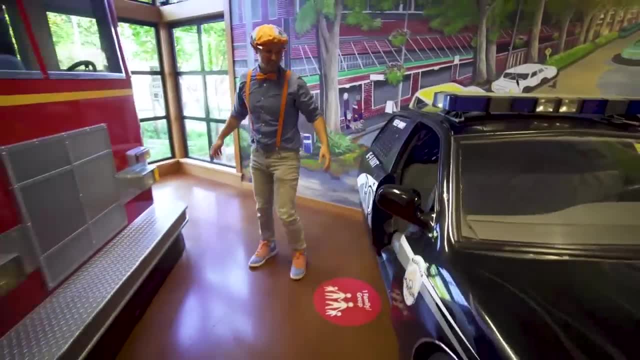 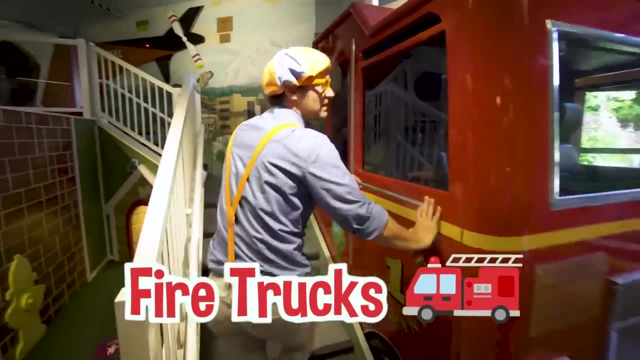 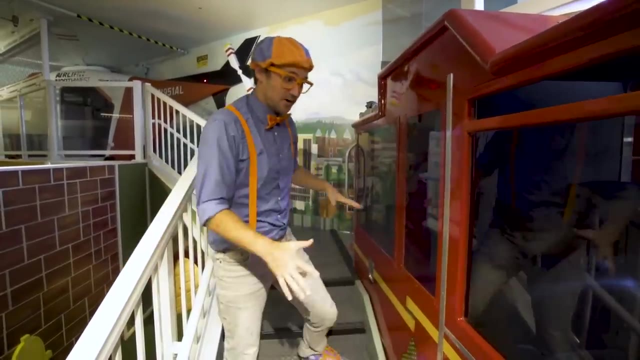 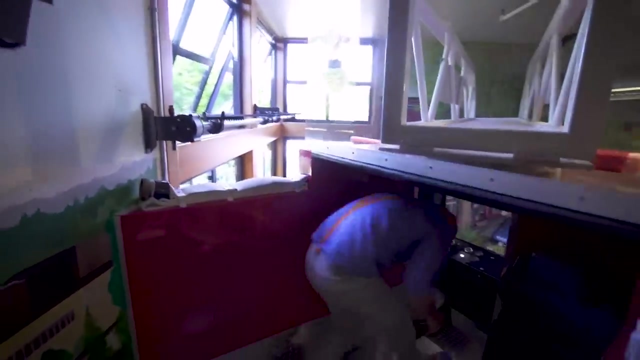 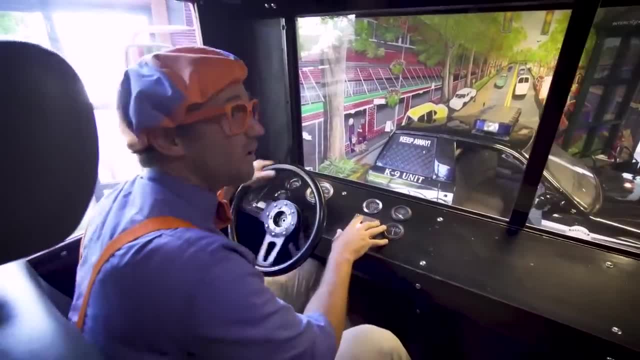 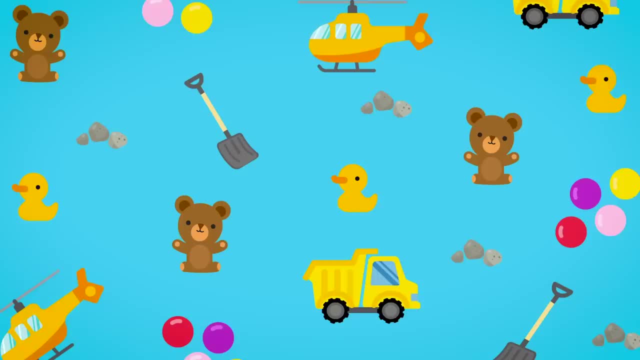 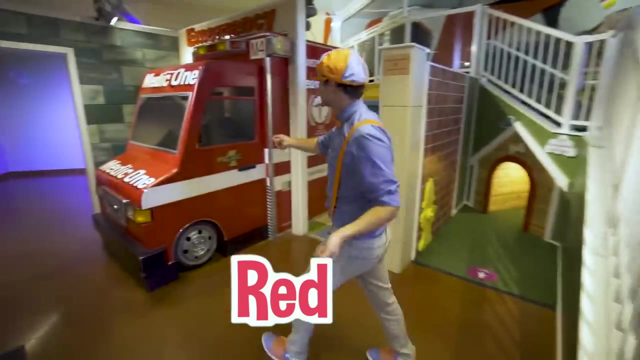 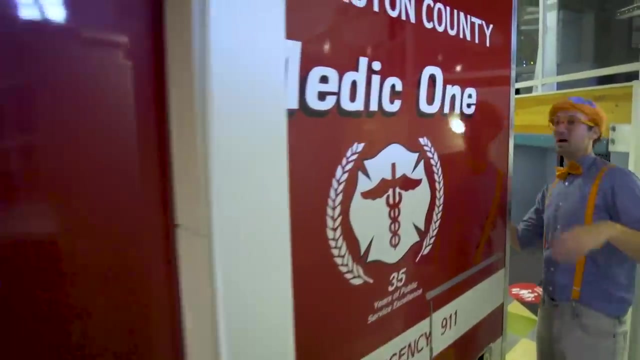 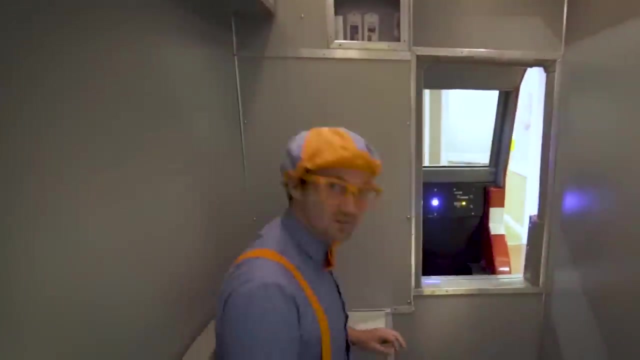 siren whoa, whoa, and i just turned on the lights. whoa, i love fire trucks. most of them are the color red, hey, red. look, this is an ambulance. whoa, the back is a big cube. hey, yeah, check it out. come on, whoa, let's go for a ride. ambulances are great because they show up if anyone needs any. 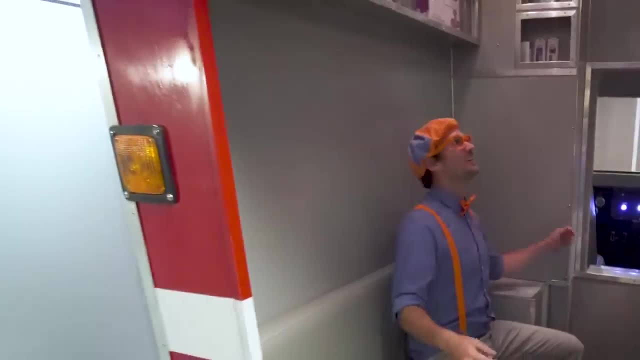 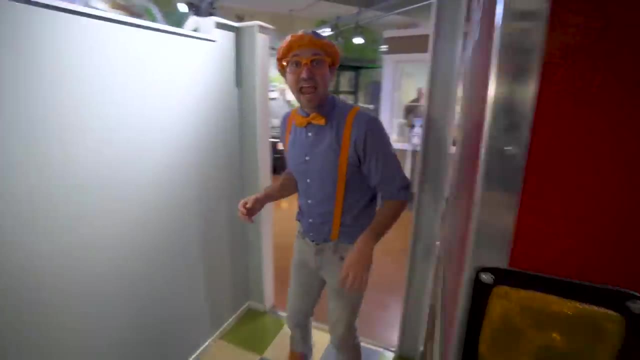 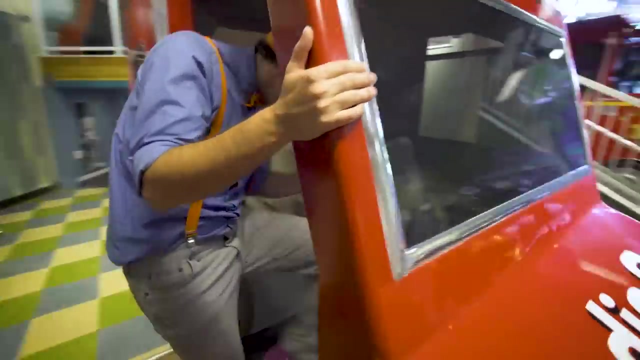 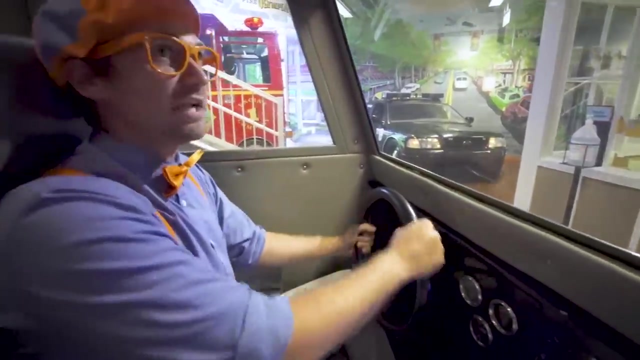 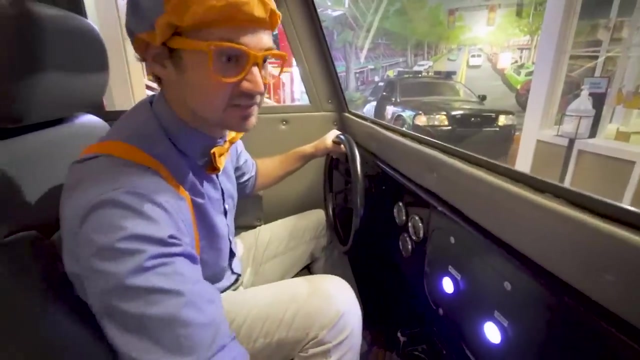 help, yeah, with their health problems. whoa, okay, and i think the front also has some lights and some sirens. whoa, move right around here and let's drive an ambulance. what is your location? oh, my location. my location is at the children's museum. okay, and we got the lights. let's go. ho ho, let's go save some people. 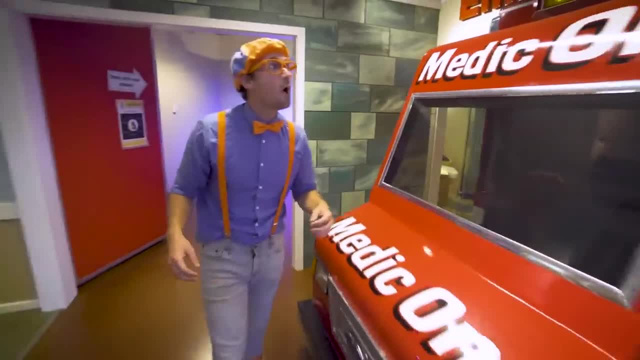 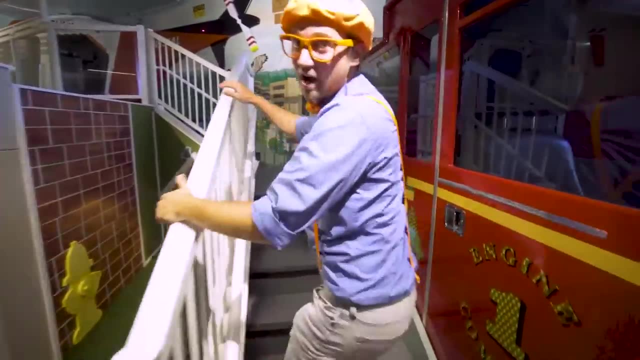 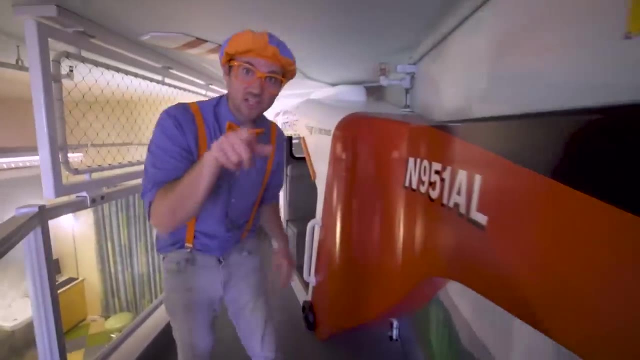 okay, and there's actually another emergency vehicle way up top. do you see it really high in the sky? let's go get it. yeah, it's not an airplane. It's kind of like an airplane because it flies in the air, But it has rotors, not jets and propellers.